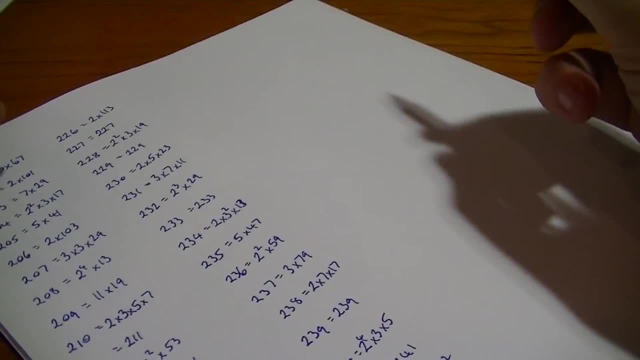 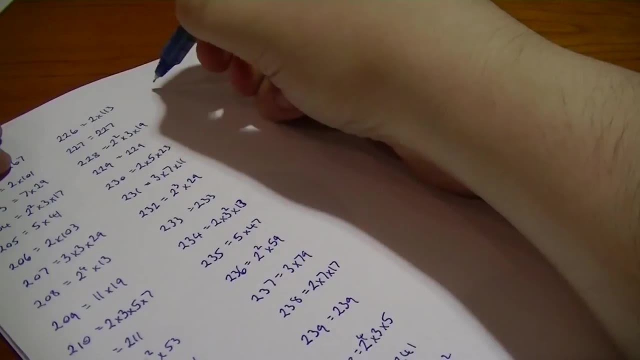 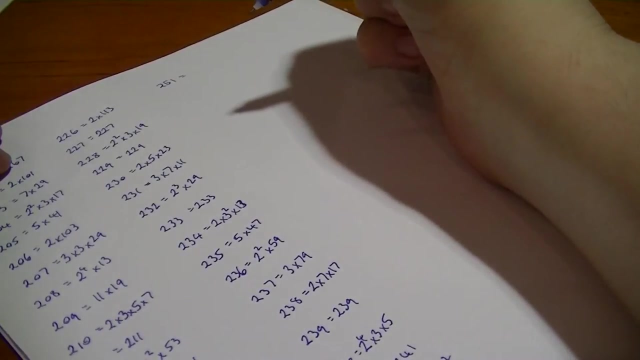 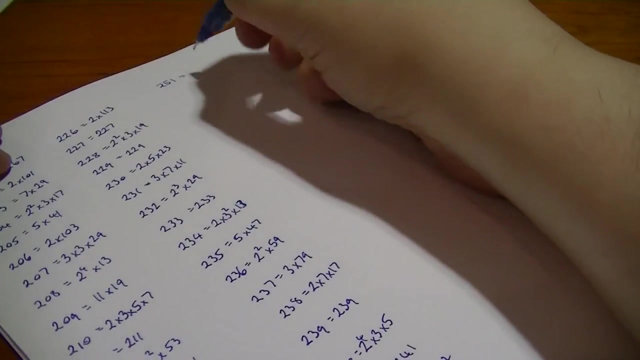 Welcome to the continuing adventures of Prime Factor Man. So let's see, Last time we got 250. So 251 isn't divisible by 2, or 3, or 5,, obviously, or 7, or 11, or 13.. So that's Prime. 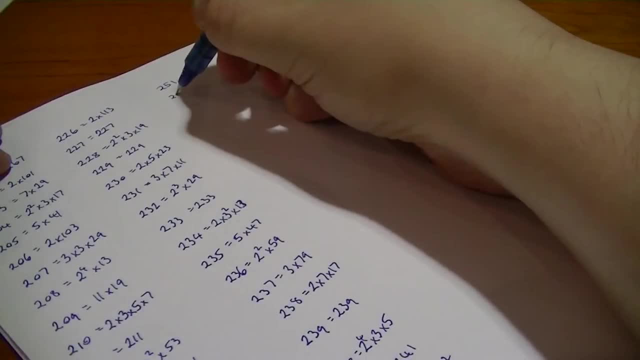 Okay, 252.. That is 2 times 126, which is 4 times 63.. So that would be 2 squared by 63, which is 9 sevenths, So that's 3 squared by 7.. 253.. That's 3.. 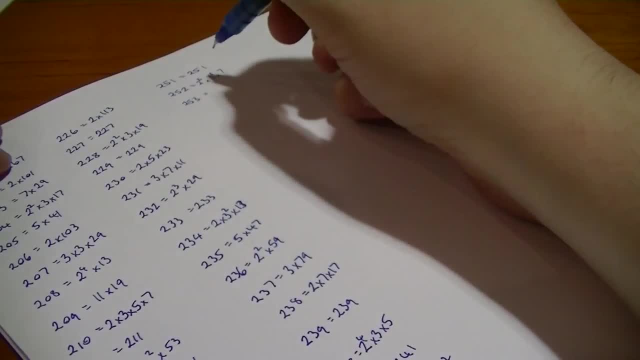 Okay, So it's divisible by 3.. Let's see 5 versus 7.. Let's see 7.. 7 does go into it. 7 goes into it. 7 goes into 25 three times, 4 times. 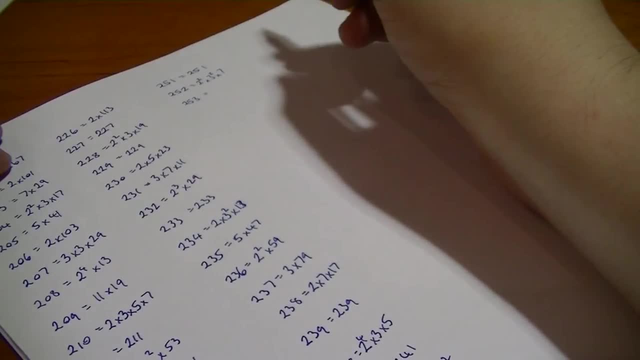 3 times 4.. So it doesn't go into 7. 11. 11. 11. 11. 23 is supposed to be 11 times 23.. 13 plus 23. Yep, So it's 11 by 23.. 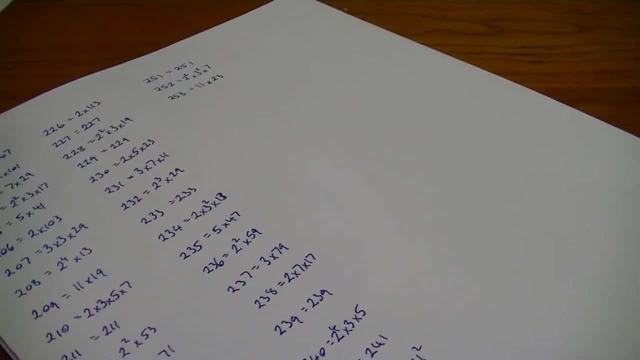 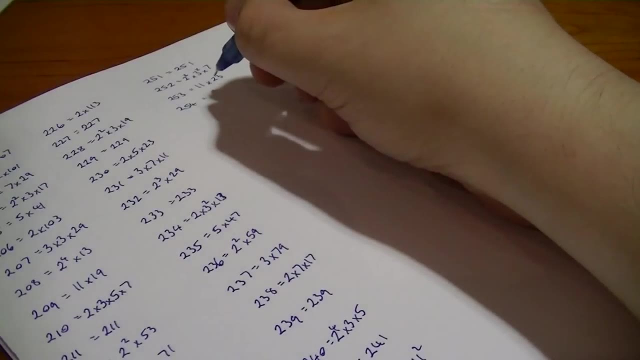 It's always going to be more awkward to figure out what is 2 primes multiplied by each other. Let's see 2 times 54.. That's 2 127ths. 127 was a prime, So that's 2 times 127.. 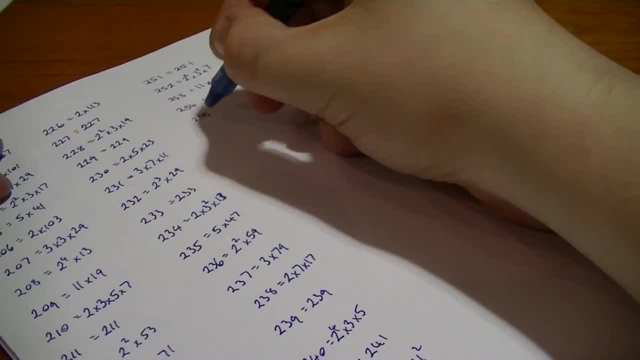 227.. 255.. That's 5 51ths. So that's 3. 5, 5.. 5, 17.. 256 is 2 to the power 8. 257.. Let's see, 2 just goes to 3, or 5, or 7, or 11.. 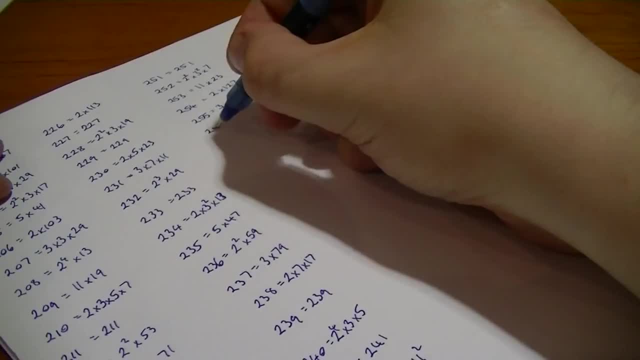 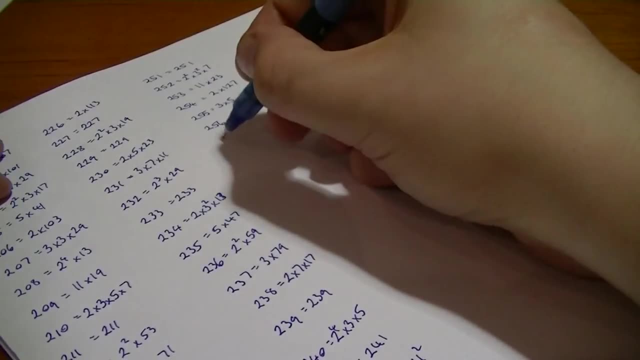 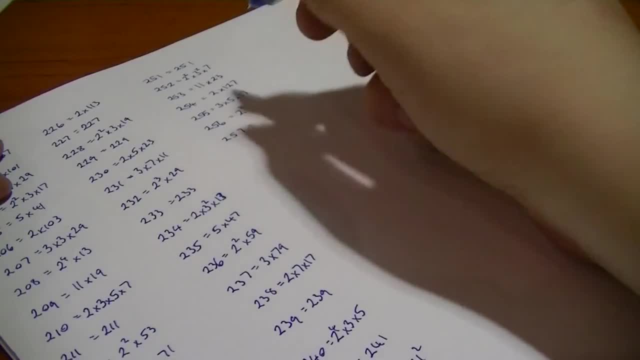 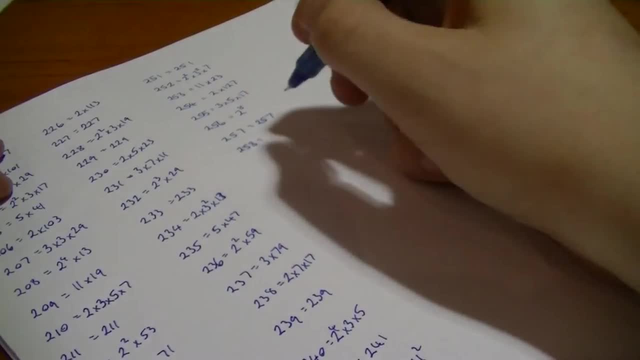 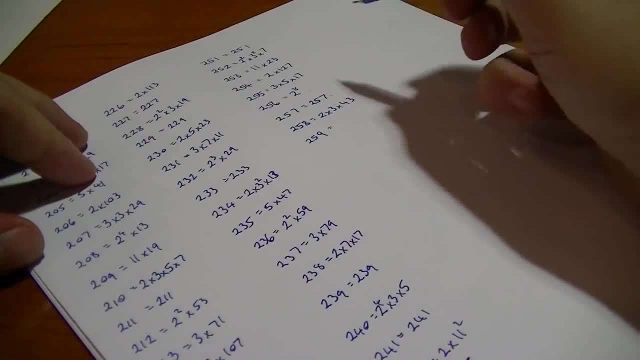 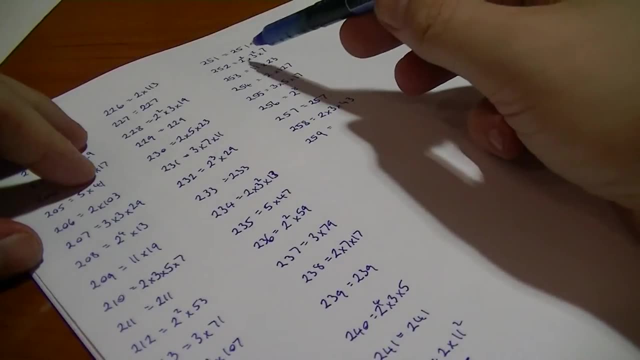 1. 1. 1. 1. Isn't divisible by 2, or 3, or 5? No, it's 7.. It is divisible by 7. That's 4 by 9, 36.. 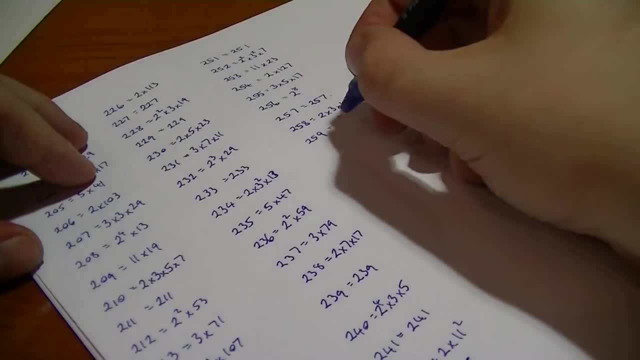 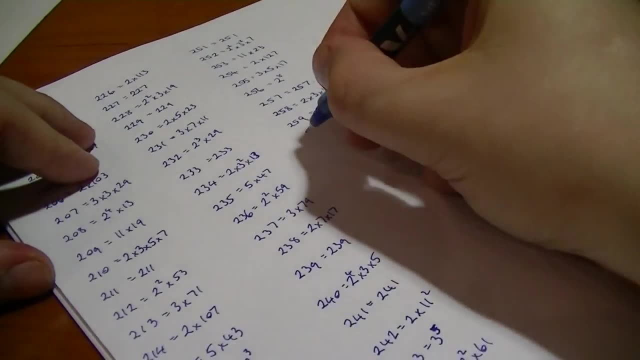 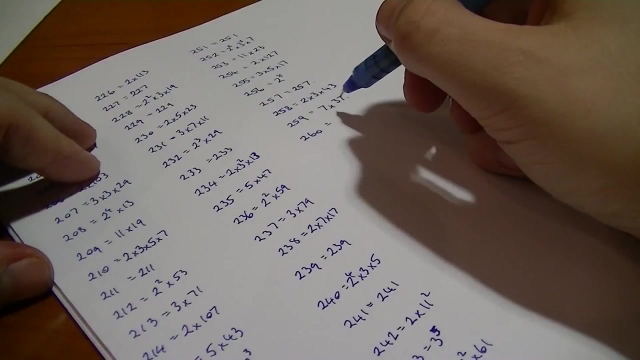 So it must be 7, 37s. Yeah, okay, 37s are pretty, So that's 7 times 37.. Let's see 260.. Right, let's see, That's 2 130s, which will be 4 65s. 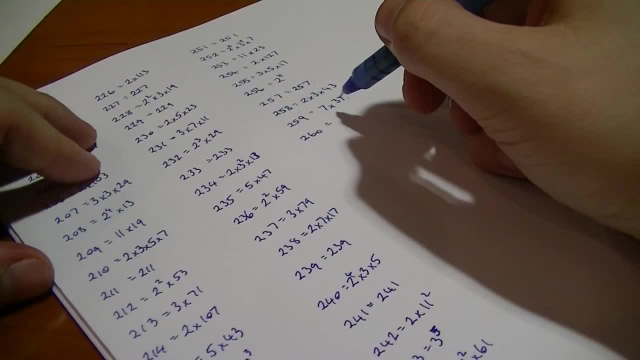 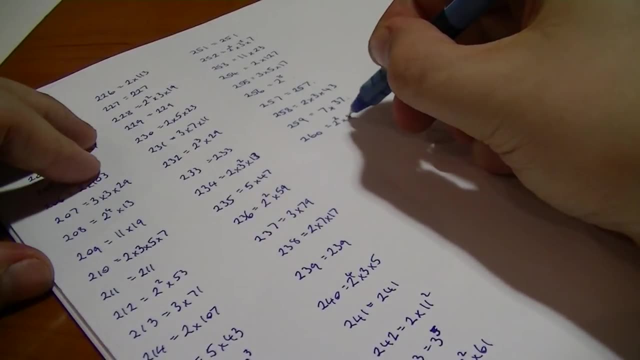 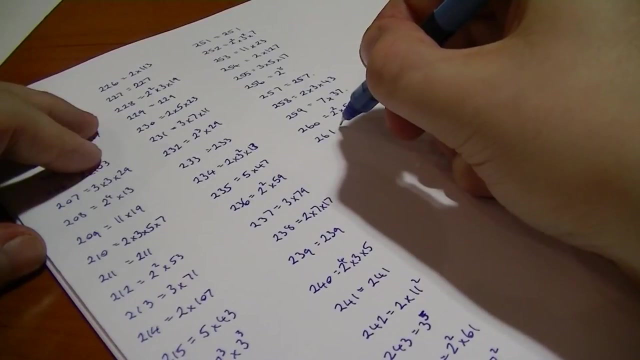 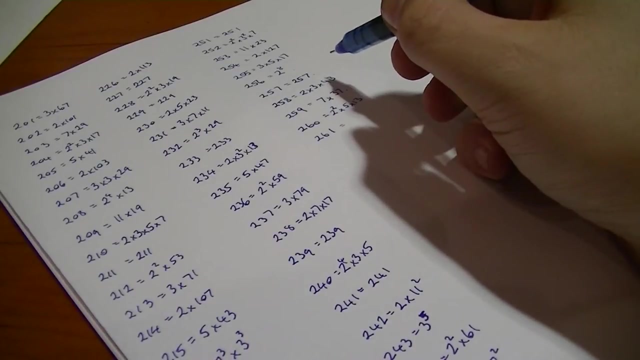 Go away, dream 4, 65s. so that's 2 squared by 65s, 5, 13s And 261.. It's divisible by 3.. It's 3, 87s, 87 is 3, 3 somethings 3, 29s. 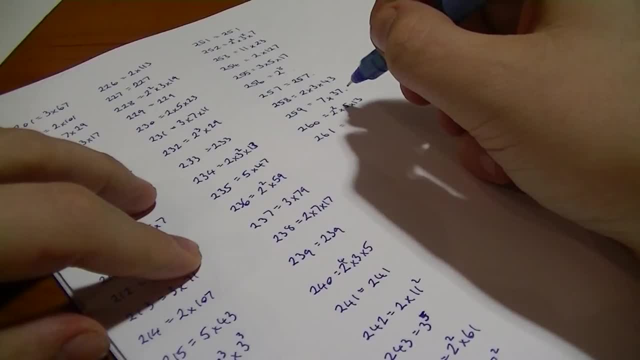 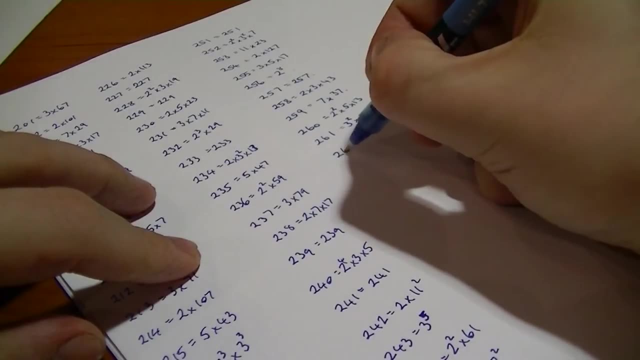 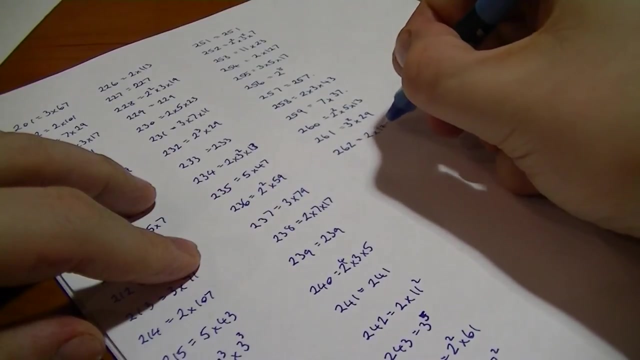 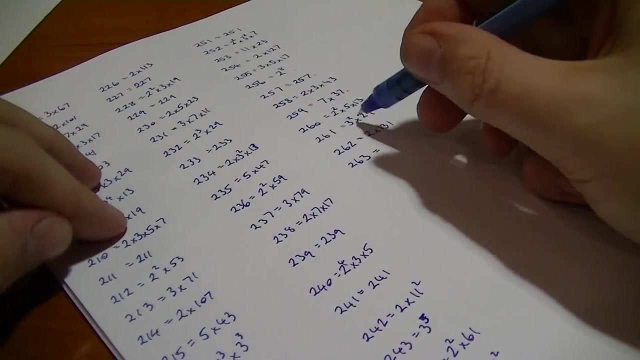 So it's 9, 29s. Yeah, okay, so it's 3 squared 1 by 29.. 262 is 2, 131s, 731s are pretty 263.. Well, it's not divisible by 2, or 3, or 5, or 7, or 11.. 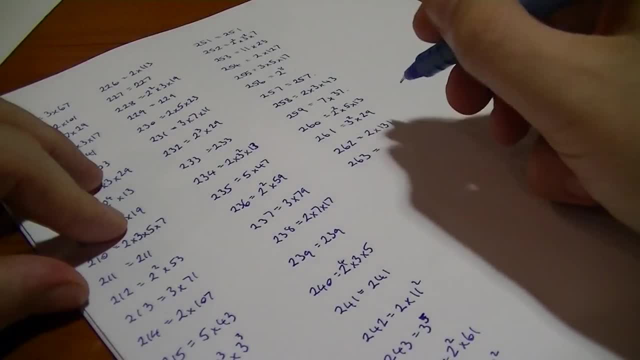 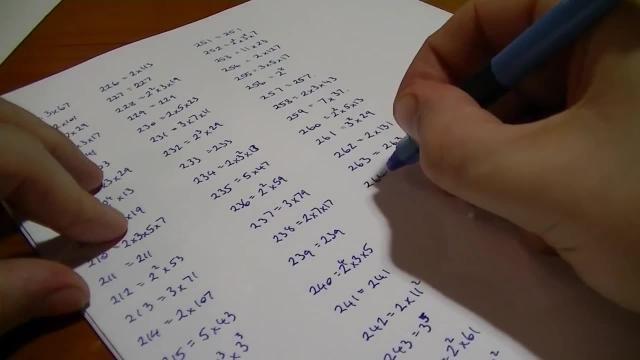 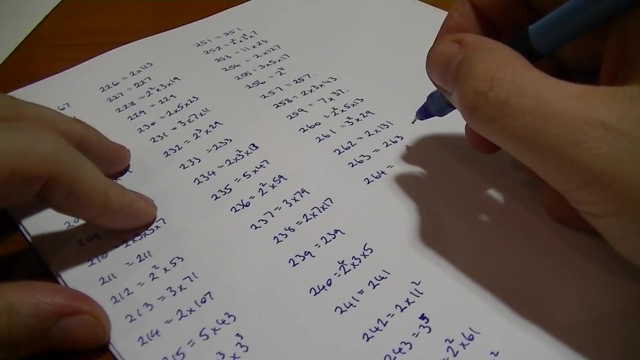 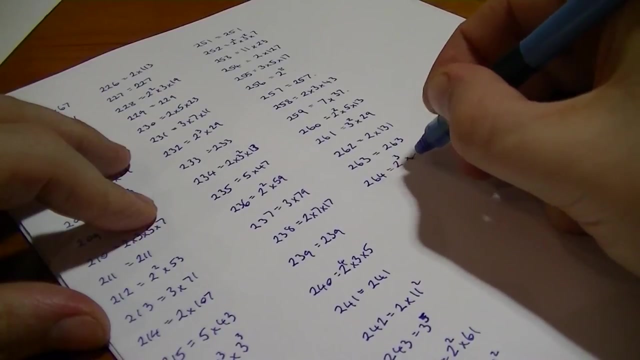 Or 13, or 17.. Or 13, or 17.. So that's a prime And 264.. That's 2 132s. So that is 2 by 2 cubed by 3, by. 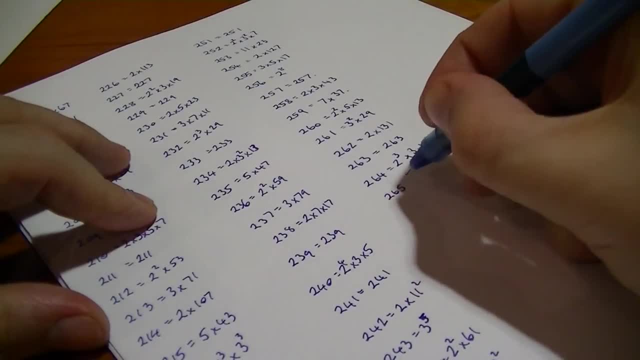 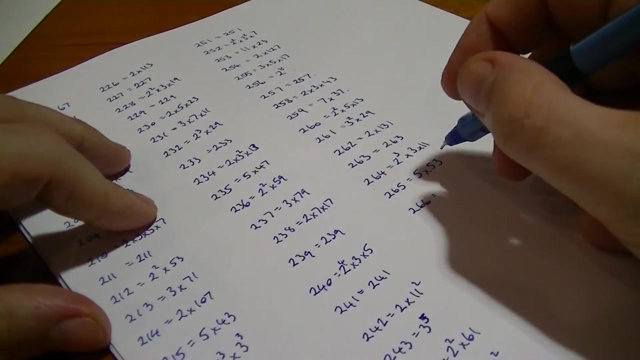 2 cubed by 3, by 265.. 265. 265.. That's five, fifty-threes. Fifty-threes are prime, isn't it? Just to be sure, Five by fifty-three. Two hundred and sixty-six, That's two hundred and thirty-threes. 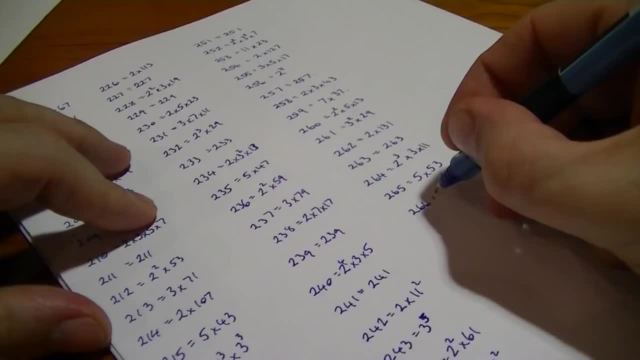 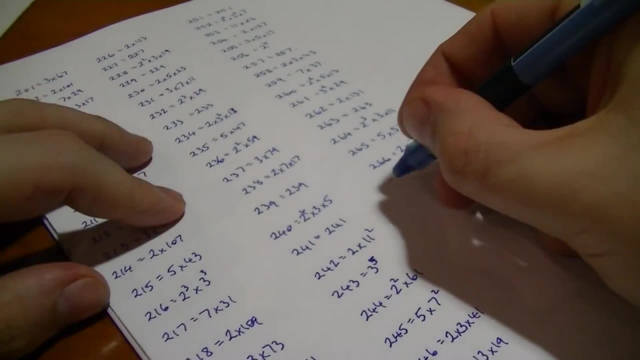 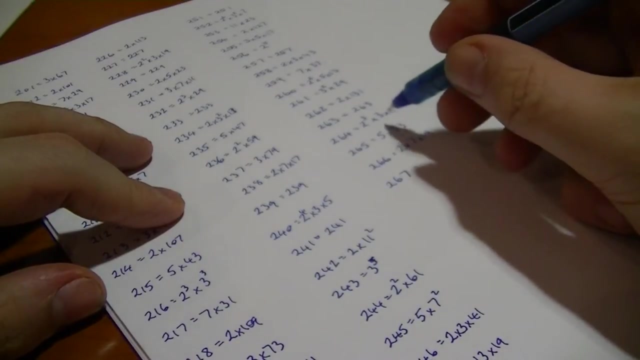 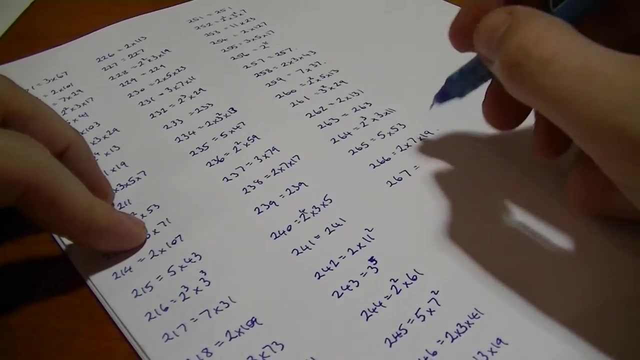 That's twenty-three. seven-nineteens, That's two by seven, by nineteen. Two hundred and sixty-seven, That's not divisible by two, That's divisible by three. Three goes into that. Eight times eighty-nine, That's three. eighty-nines, Eighty-nines are prime all day long. 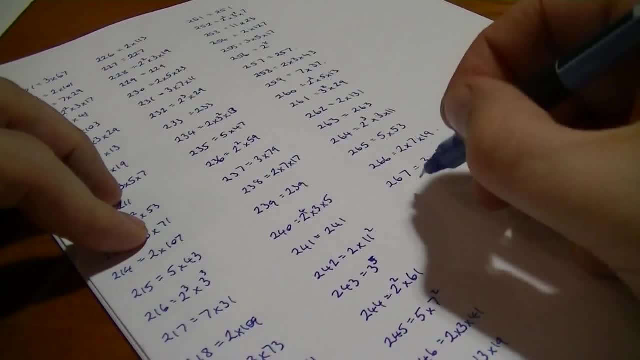 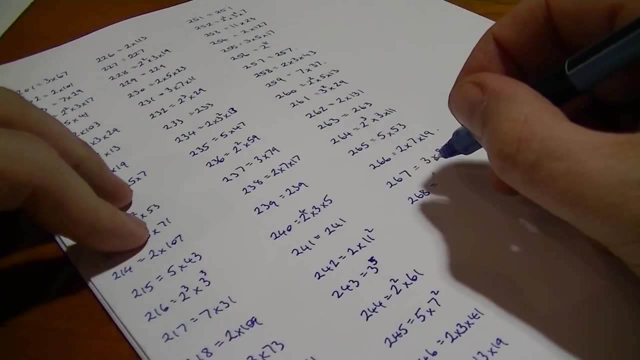 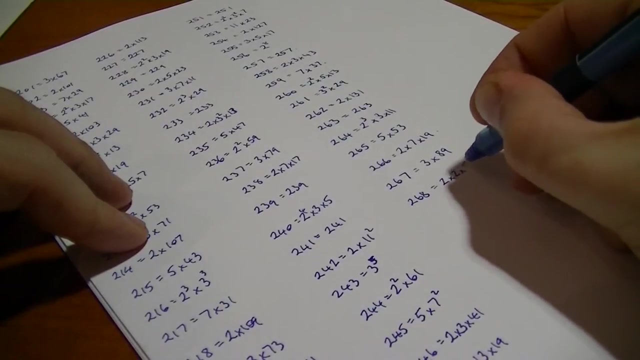 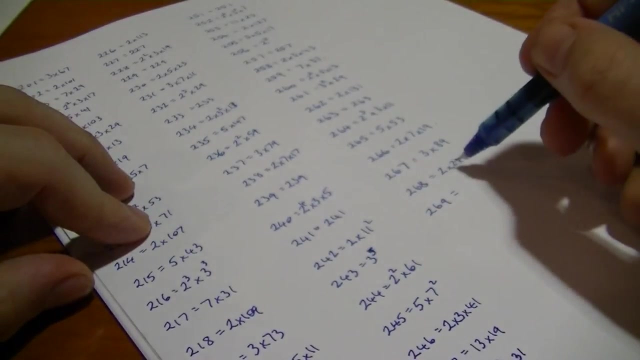 Three by eighty-nine. Two hundred and sixty-eight is two. one hundred and thirty-fourths, which is two, sixty-sevenths. Sixty-sevenths are prime, That's two by two by sixty-seven. Two hundred and sixty-nine. That's not divisible by two or three or five or seven or eleven. 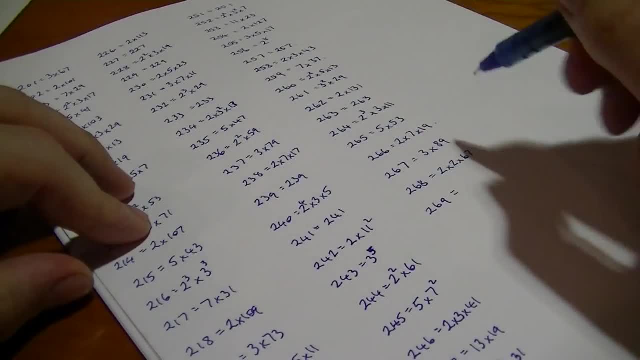 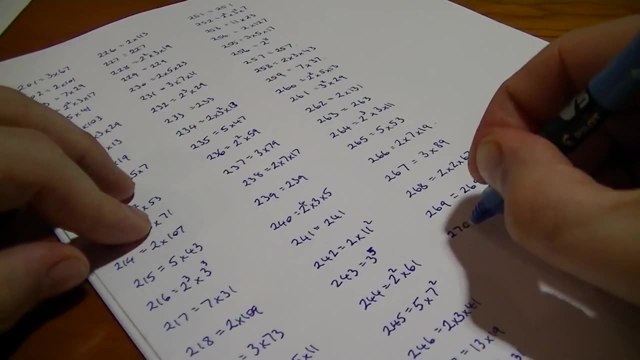 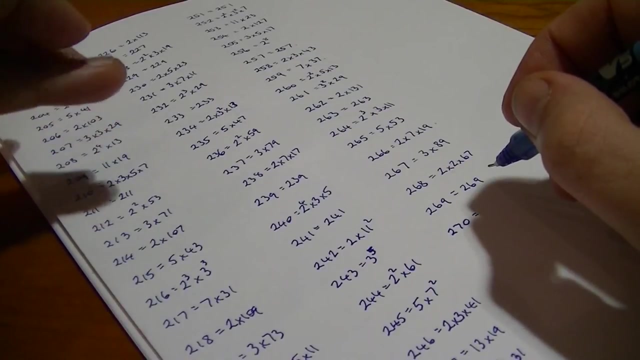 Or thirteen, So there are four. That's a prime. Two hundred and seventy is two. one hundred and thirty-fifths. One hundred and thirty-five is nine-fifths. No, it's not nine-fifths, It's twenty-seven-fifths. 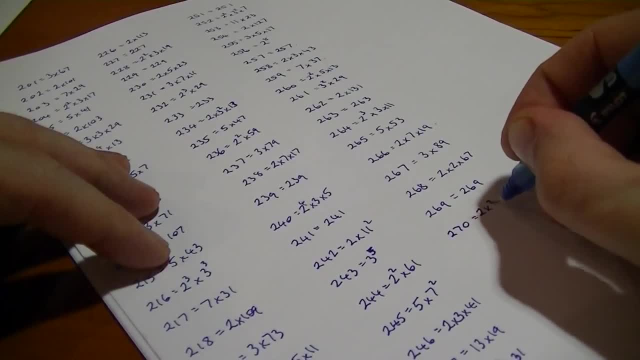 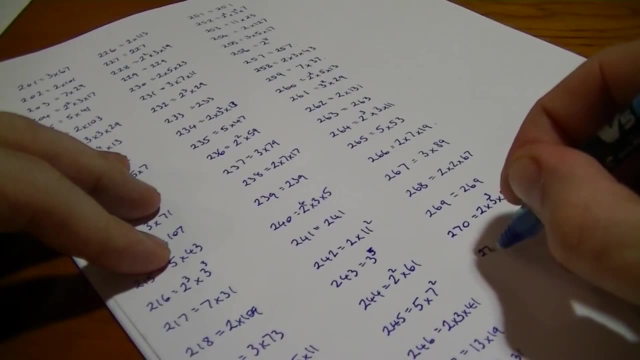 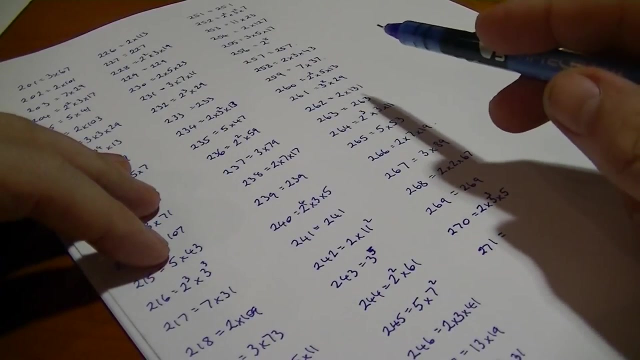 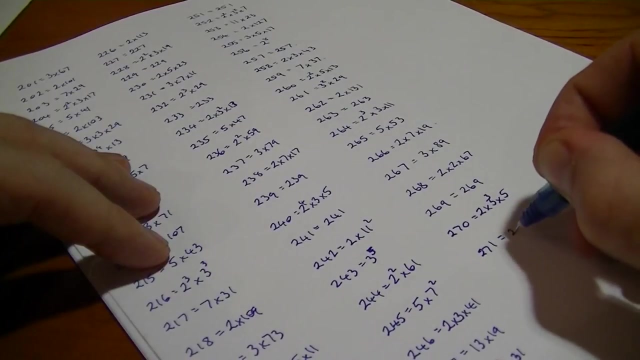 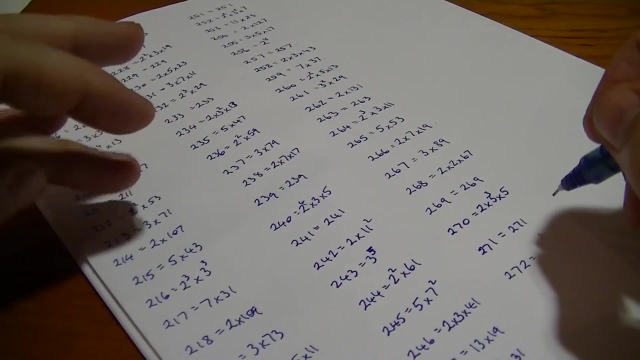 So that's two by three cubed by five. Two hundred and seventy-one, That's divisible by two or three, or five or seven, or eleven or thirteen, So it's a prime. Two hundred and seventy-two is two. one hundred and thirty-sixths. 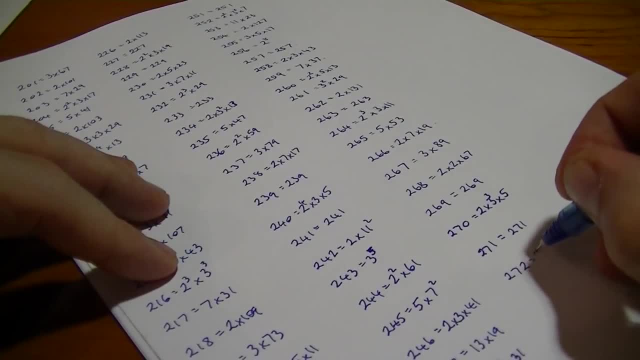 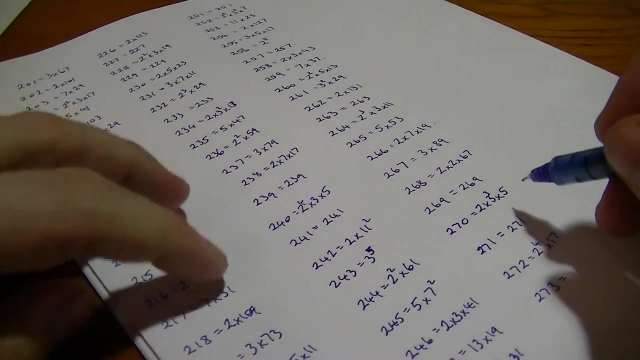 One hundred and thirty-sixths is eight-seventeenths, So that's two Or four times seventeen. Two hundred and seventy-three It's divisible by three, That's three ninety-ones, And ninety-one is seven thirteenths, I believe. 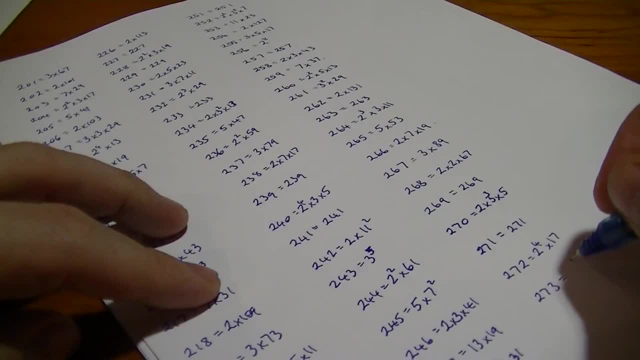 So three by seven, One by thirteen, Seven, thirty-eighths. Yep, okay, I thought for a second there. I just looked a wee bit too high, but that's right, Two hundred and seventy-four is two, one hundred and thirty-sevenths. 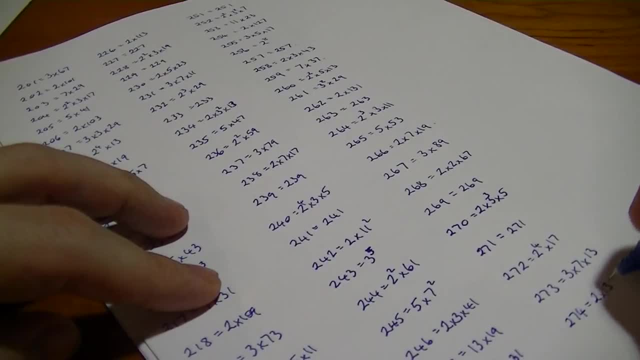 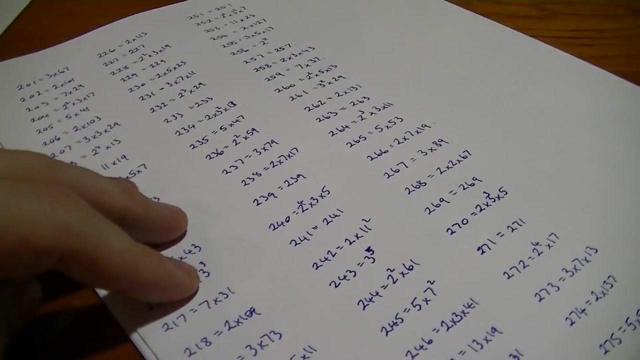 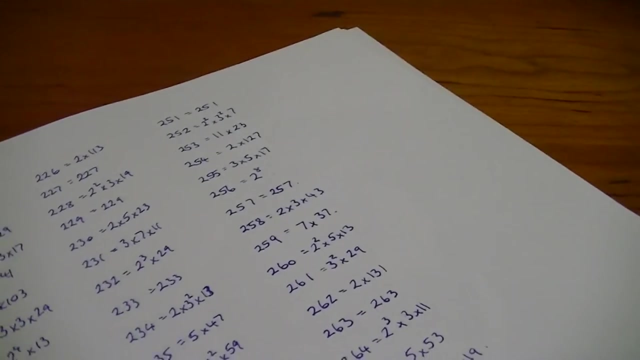 One hundred and thirty-sevenths is a prime, So that's that. And then two hundred and seventy-five, Well, that's eleven, twenty-fifths, So that's five by five by eleven. Okay, duck, So let's see. 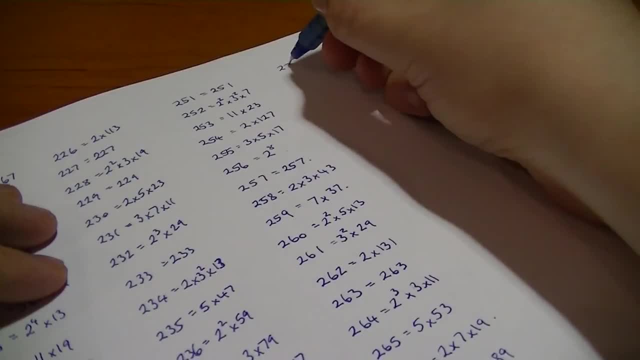 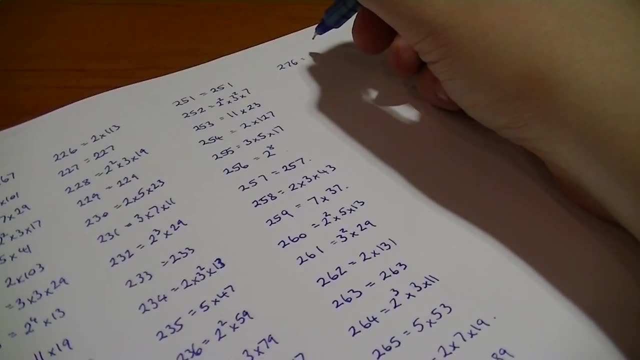 Two hundred and seventy-five, So that's a nine. Two hundred and seventy-six, So that's two hundred and thirty-ninths. One hundred and thirty-ninths, Two hundred and thirty-ninths, two hundred and thirty-eighths. 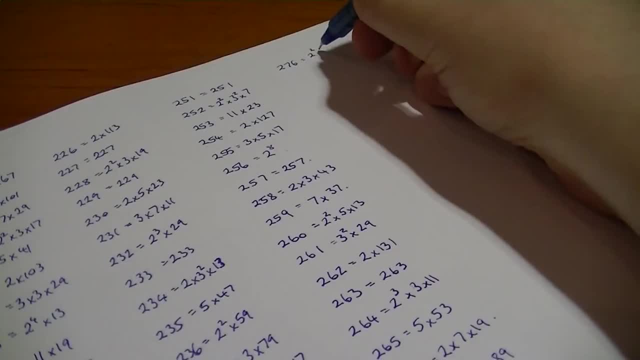 Which is just two squared by three, by twenty-three, Four, twelve, twenty-threes, Ten, twenty-threes, Twenty plus forty-six yep, So three hundred and seventy-seven. That's not divisible by two or three or five, Or seven, or eleven or thirteen. 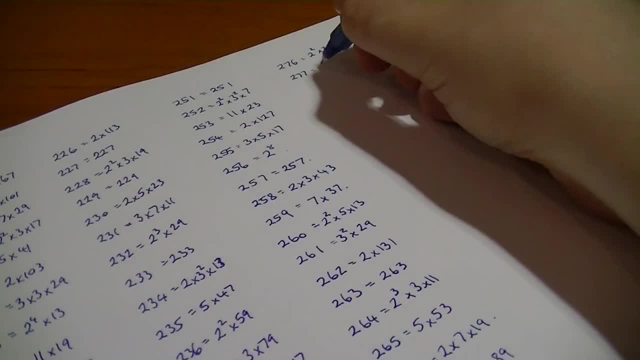 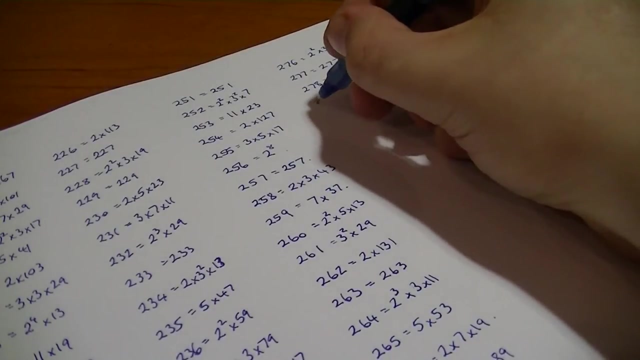 Or seventeen, So that's a prime. Three hundred and seventy-eight, That's two hundred and thirty-ninths. One hundred and thirty-ninths of primes, So that's two by one: three, nine, Two hundred and seventy-nine. 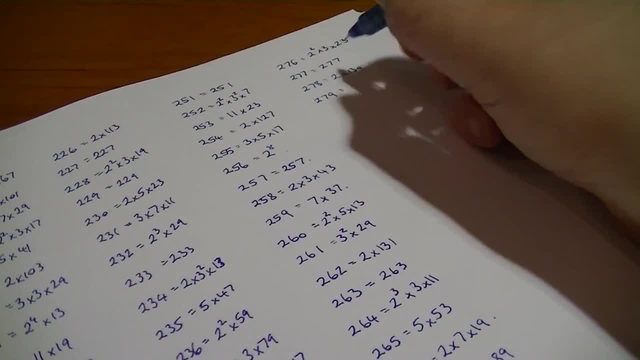 It's supposed to be three, It's three ninety-threes, Which is nine thirty-ones, Thirty-ones of primes. So that's three by three, By thirty-one. Yep, that's right. Two hundred and eighty, That's two hundred and four seven-threes. 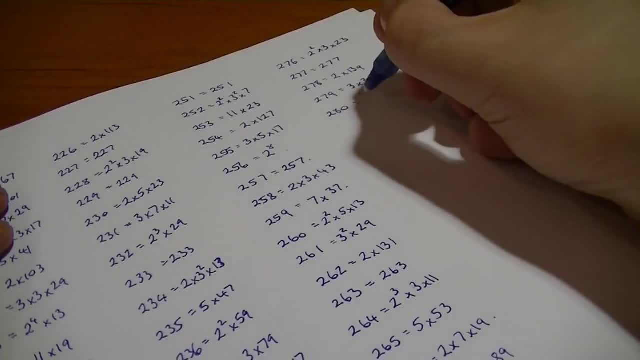 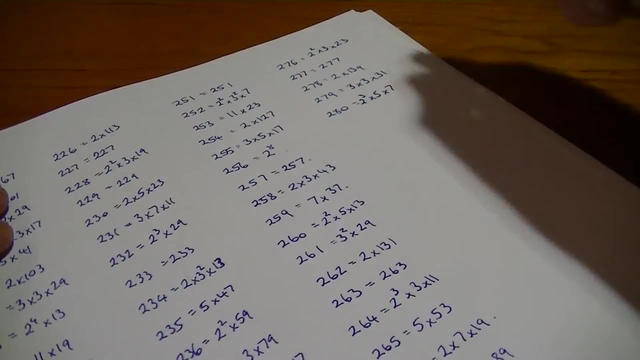 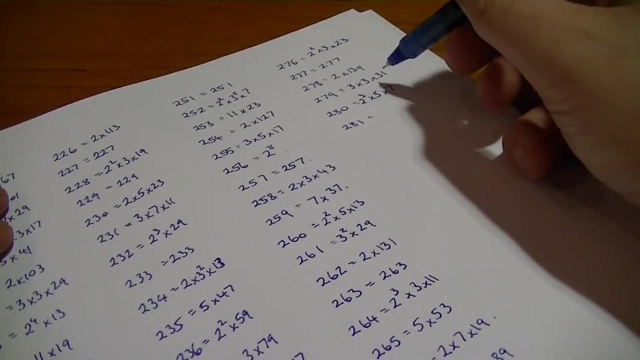 Which is eight thirty-fives, So that's two cubed by five, By seven. Two hundred and eighty-one. That's not divisible by two or three or five or seven, Or eleven Or thirteen, Or It's like a bar. 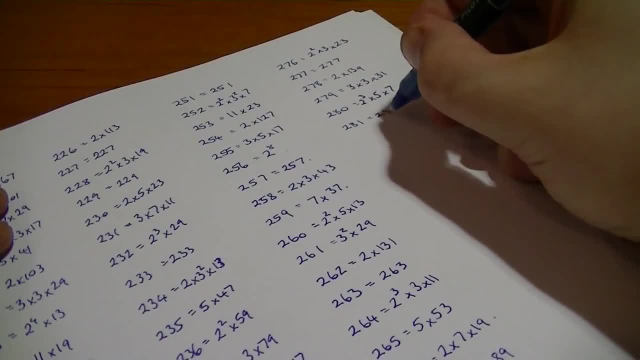 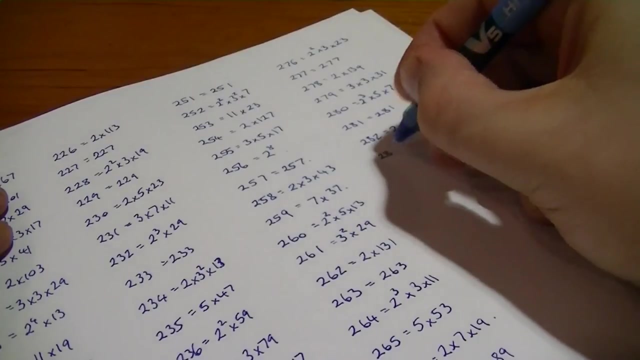 Anyway, or seventeen, So that's a prime. Two hundred and eighty-two, That's two hundred and forty-ones, Which is three, forty-sevenths, So that's two by three, by forty-seven, Seventy-one of primes. 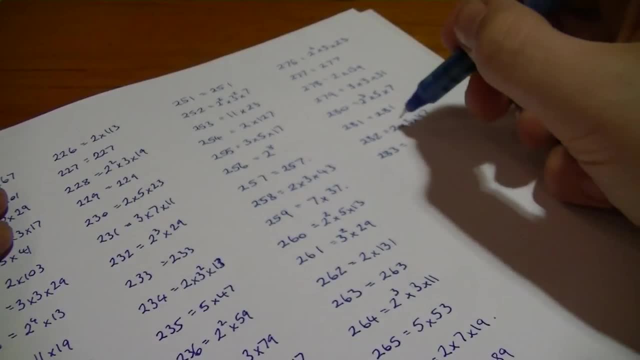 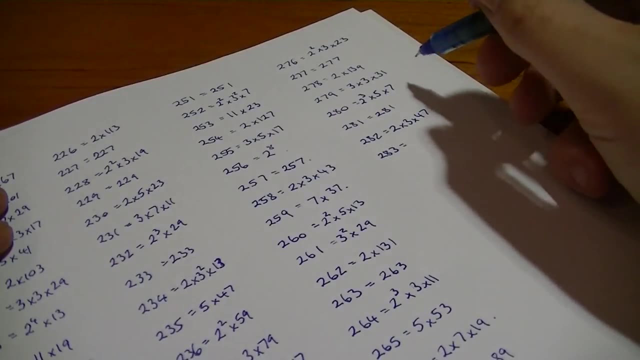 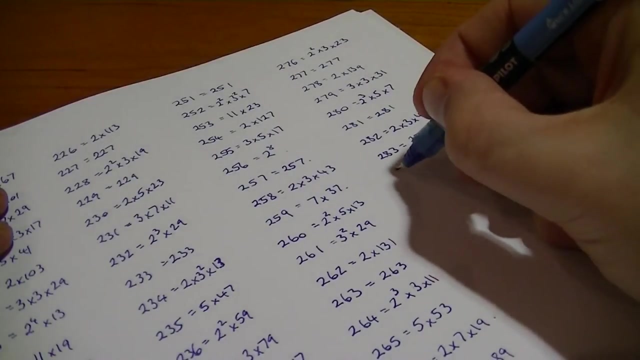 Two hundred and eighty-three, Which is, Let's see, that's supposed to be two or three or five or seven, Or eleven, Or thirteen, Or thirteen Or thirteen, So that's a prime. Two hundred and eighty-four. 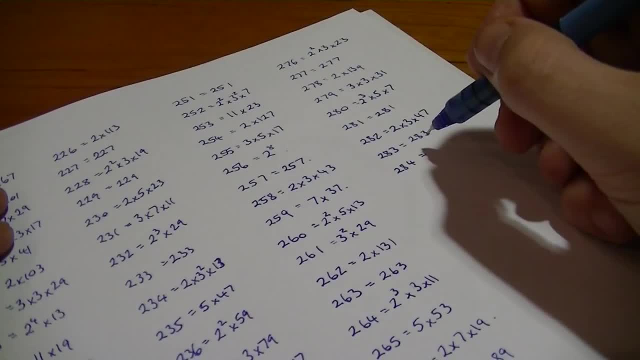 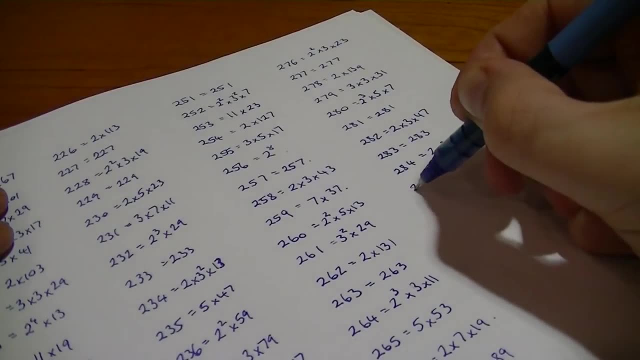 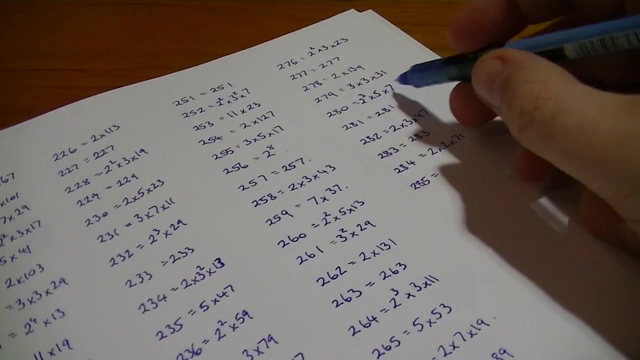 That's two hundred and forty-two, Which is four, seventy-ones, So that's two by two, by seventy-one. Two hundred and eighty-five, That's- Let's see, that's Fifty-six, So that's fifty-seven fives. 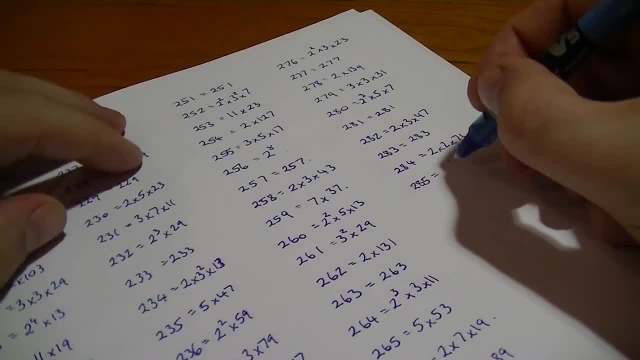 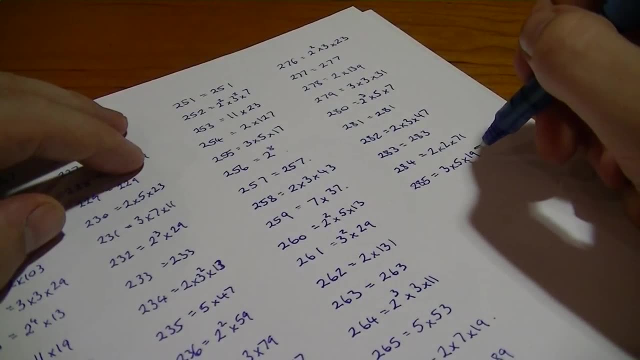 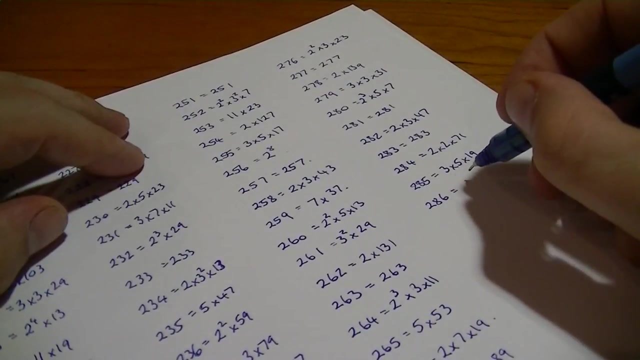 Yeah, fifty-seven, fives, Fifty-seven is three, nineteen, So that's three by five, by nineteen. Yeah, Okay, Three hundred and eighty-six, That's two, one hundred and forty-threes, And one hundred and forty-three is eleven. thirteenths. 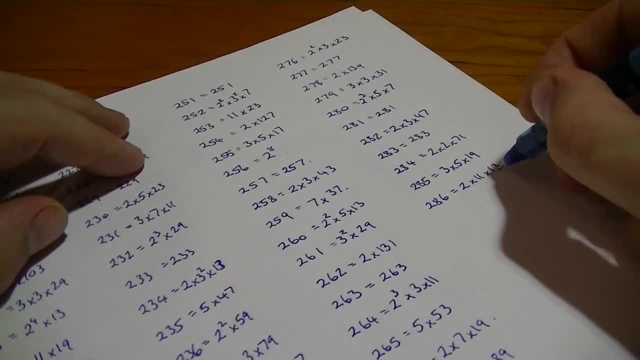 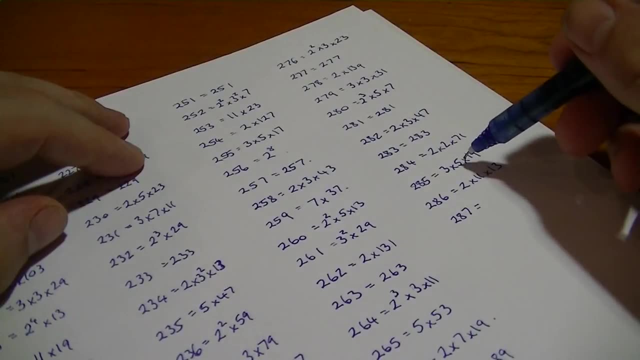 So that's two by eleven by thirteen. Two hundred and eighty-seven, That's right stomach and eye. So not divisible by two, It would be divisible by eleven. No Thirteen Divide thirteen, Would you say four. 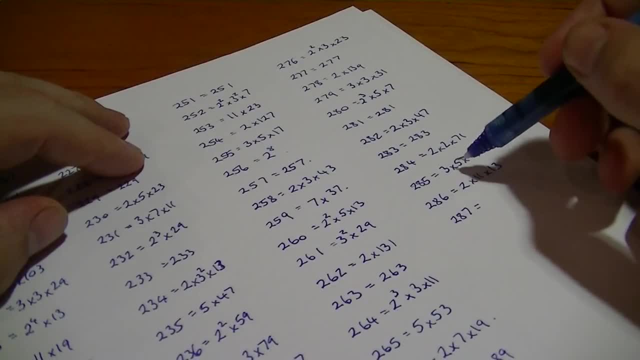 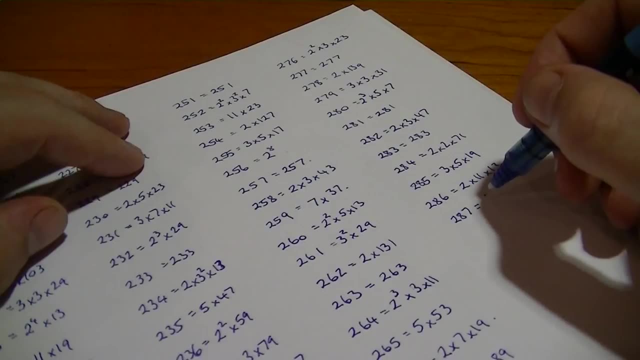 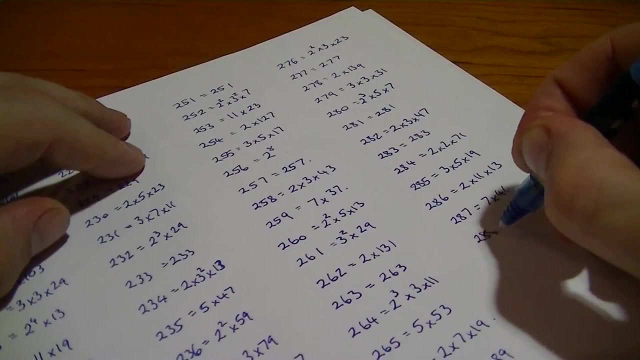 Yeah, No, Not divisible by two or three or five. Oh, it's divisible by seven. That's seven forty-ones, And forty-one is a prime. So that's So, that's just seven by forty-one. Two hundred and eighty-eight. 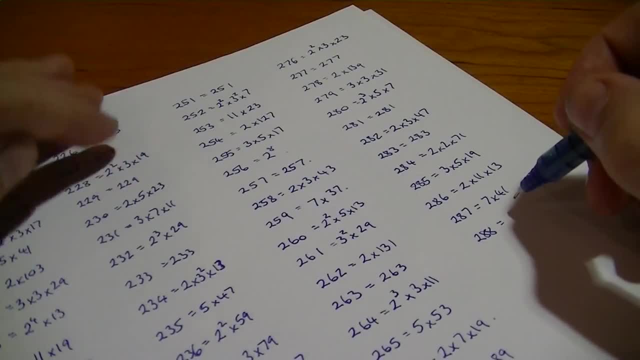 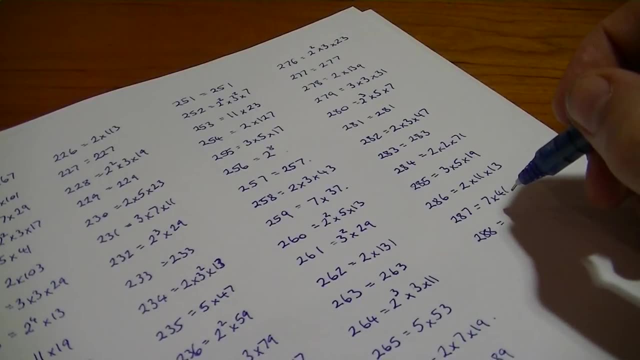 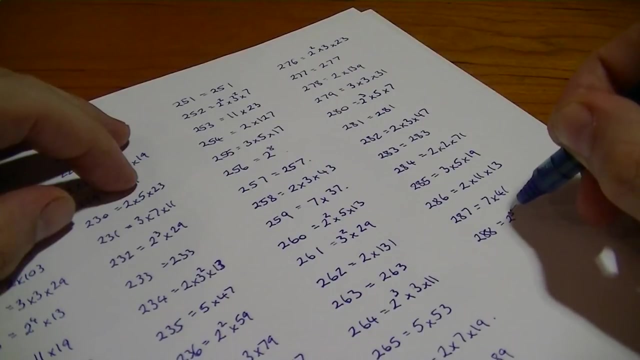 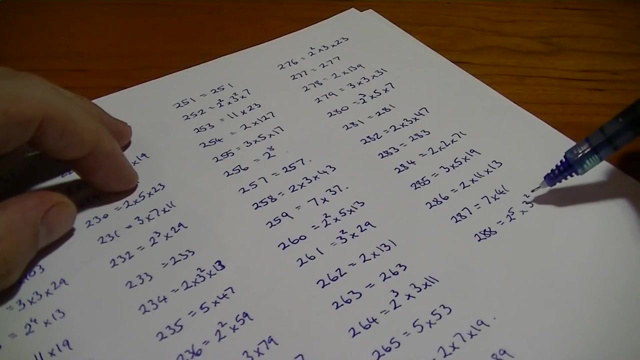 That's four, seventy-twos, Which is eight, Thirty-six is sixteen, Eight, tenths, Which is thirty-two, ninths. So that's two to the power of five Times three squared: Thirty-two ninths. Yeah, that's right. 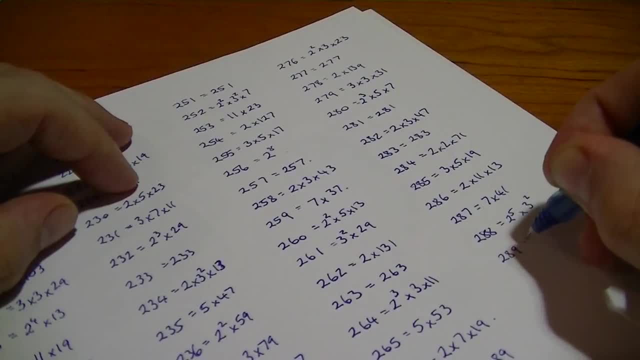 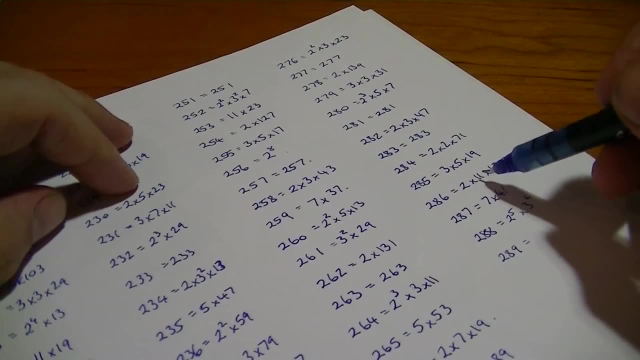 Okay, Thirty-nine, Right, So not divisible by two or three or five or seven, or eleven or thirteen, That's seventeen squared. Anyway. Two hundred and eighteen, That's two. one hundred and forty-fives. One hundred and forty-five is five, twenty-ninths. 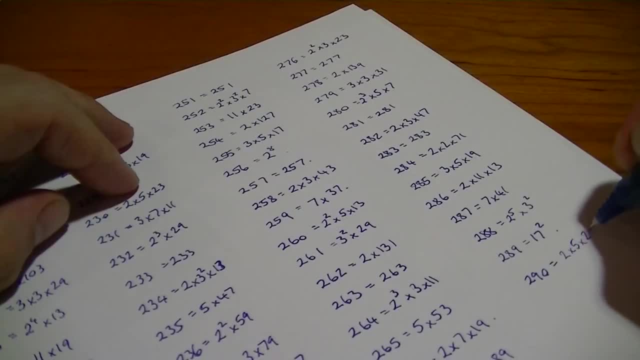 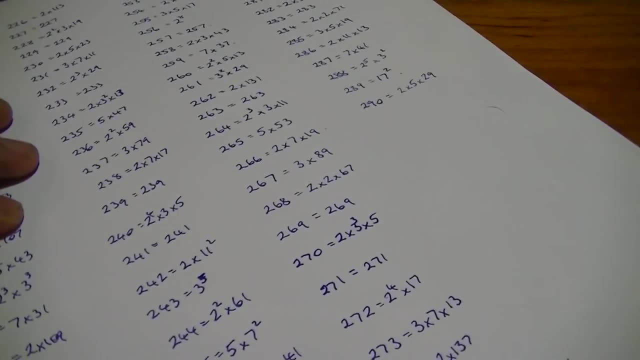 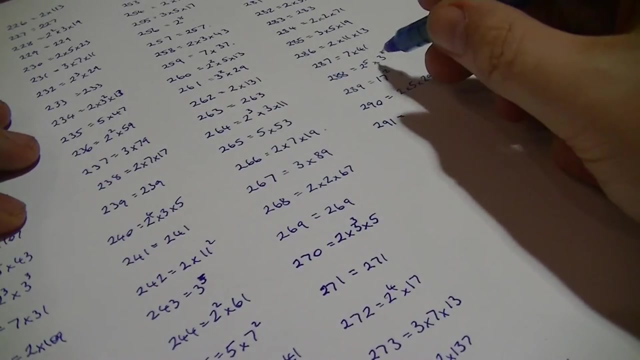 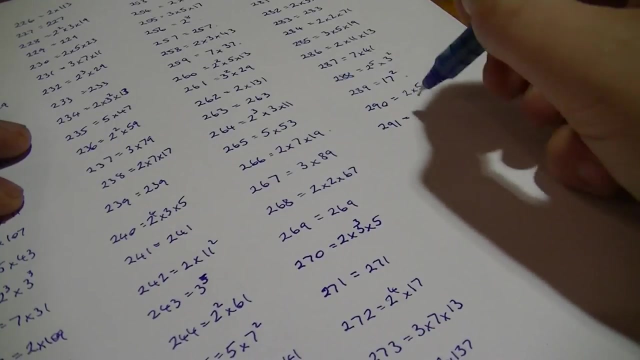 So that's two by five, Five, twenty-nine, Two hundred and ninety-one. Not divisible by two, Divisible by three, The money that goes out of that Two to the power of five is thirty-two, Ninety-six, That's three, ninety-sevens. 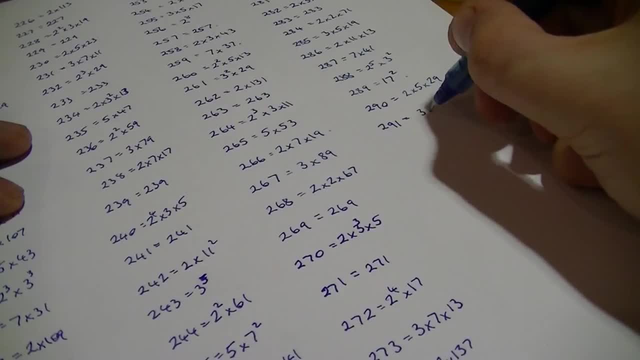 That's ninety-seven. Ninety-seven is a prime. Two hundred and ninety-two is two. one hundred and forty-six, Which is four. seventy-threes And seventy-three is a prime. So that's two by two, by seventy-three, Two hundred and ninety-three. 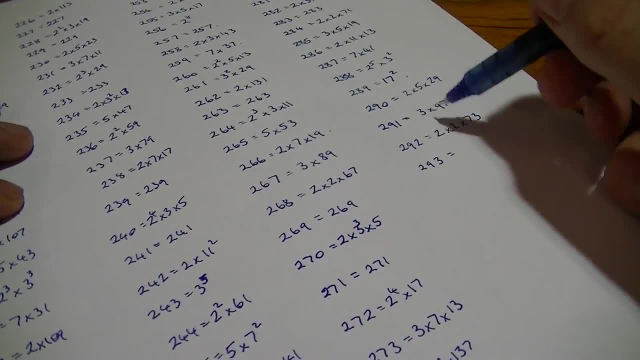 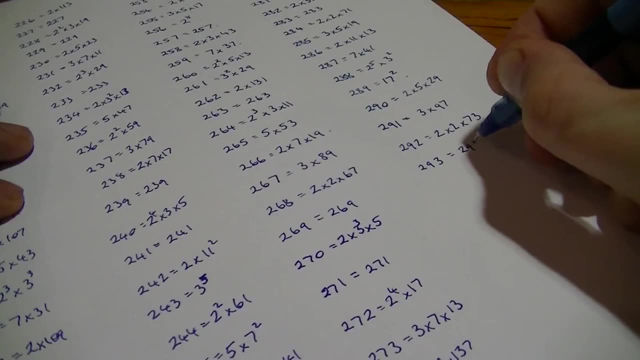 Not divisible by two or three or five or seven or eleven or thirteen or seventeen. So that's a prime. Two hundred and ninety-four, That's two hundred and forty-sevenths, And forty-sevenths, That's two by three, by seven squared. 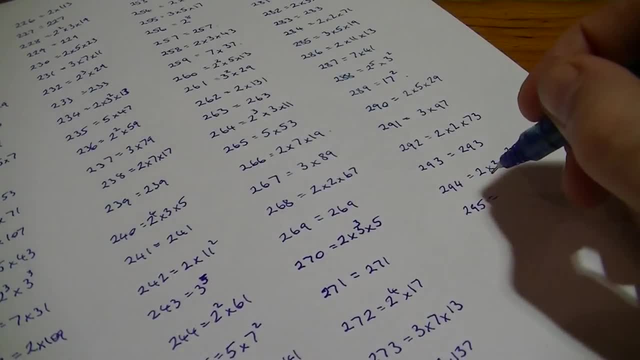 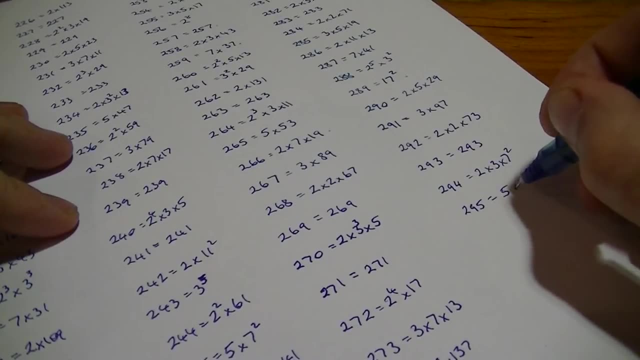 Two hundred and eighty-five, Three hundred and sixty-six, That's five, fifty-ninths And fifty-ninths a prime. Two hundred and eighty-six, That's two hundred and forty-eighths, And that's two cubed. 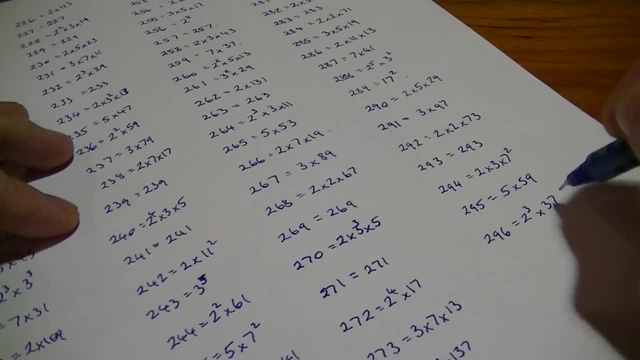 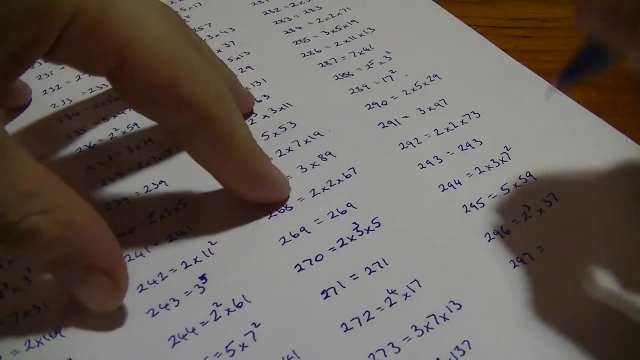 By thirty-seven. Yeah, thirty-sevenths, Yep, So two hundred and ninety-seven. It's not divisible by two, It's divisible by three. That's three ninety-ninths, Which is nine thirty-threes, Which is twenty-seven elevens. 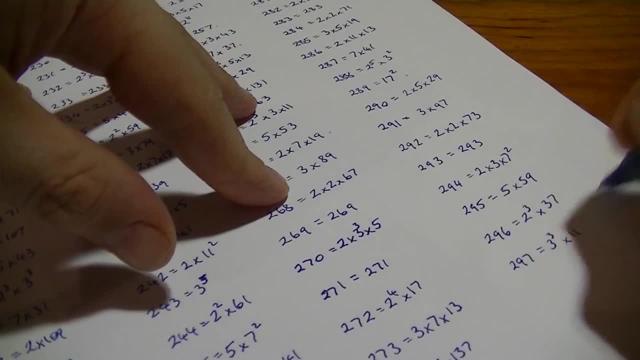 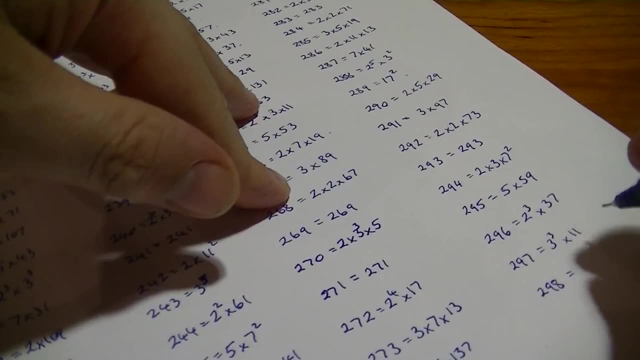 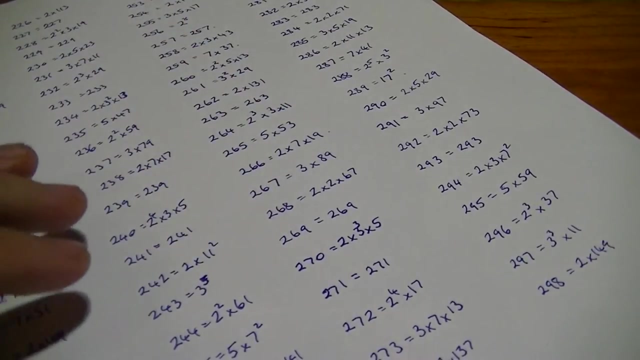 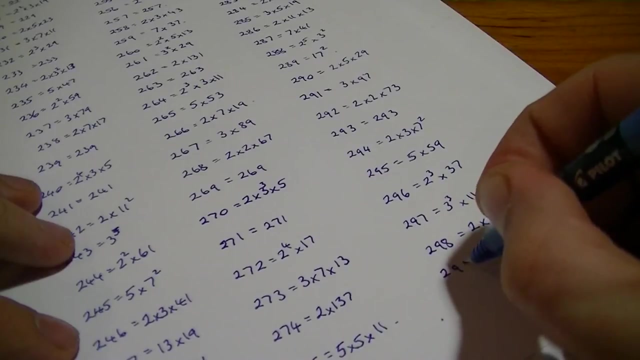 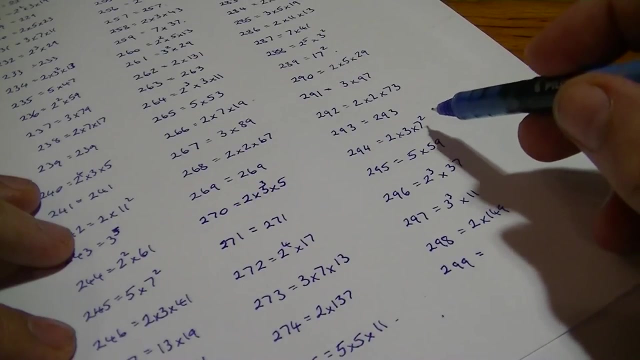 So that's three cubed by eleven, Yep Two hundred and ninety-eight, That's two hundred and forty-ninths, Forty-ninths, a prime, That's two by one, four, nine, Two hundred and eighty-nine, Not divisible by two or three or five or seventeen. 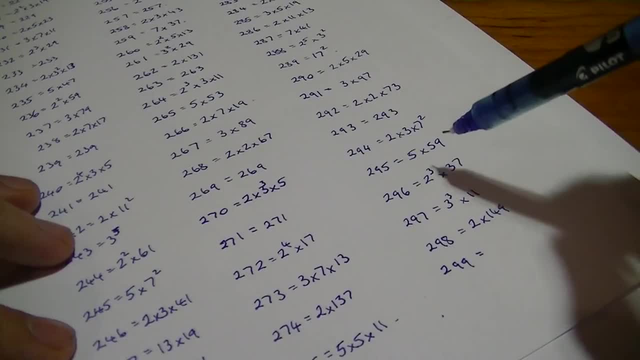 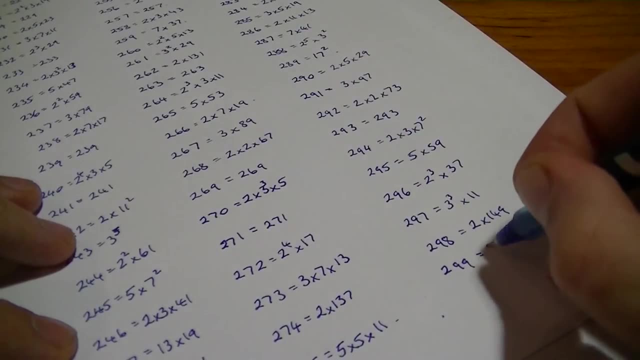 No eleven, No thirteen, Eighty-six, It is So thirteen. That was twenty-two thirteens, So it's supposed to be twenty-three thirteens, So that's thirteen times twenty-three. 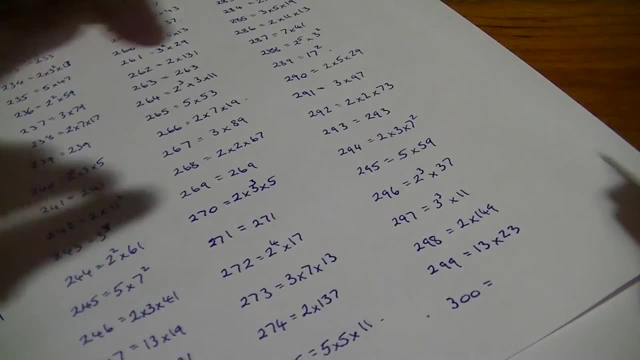 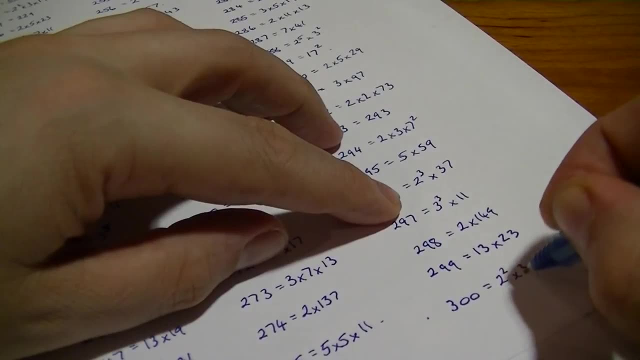 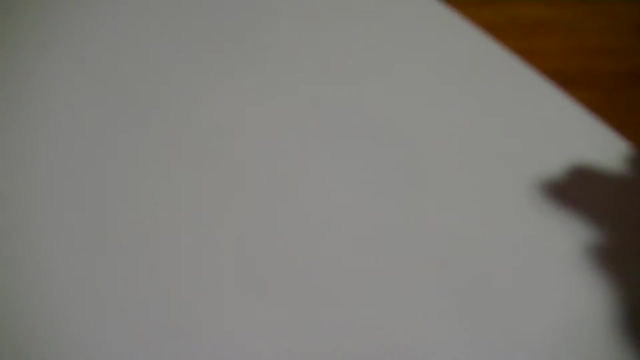 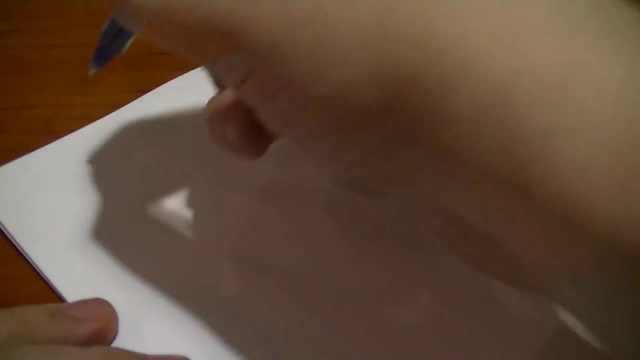 And then finally three hundred, Not barely, And this page is two hundred and fifty-sevenths, That's four, seventy-fives, So that's two squared by three, by five squared Right. Here's all the material. So we are on to three hundred and one. 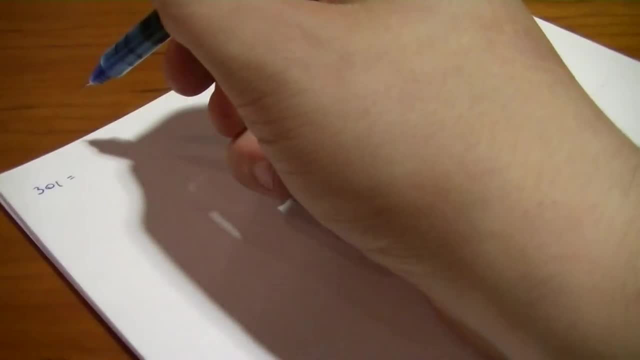 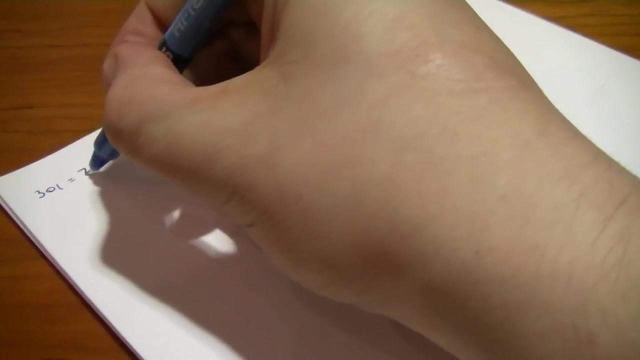 So it's not divisible by two or three or five, It is divisible by seven. And this seven, six, forty-three, seven, forty-threes, Yep, Forty-threes a prime. So it's seven by forty-three. 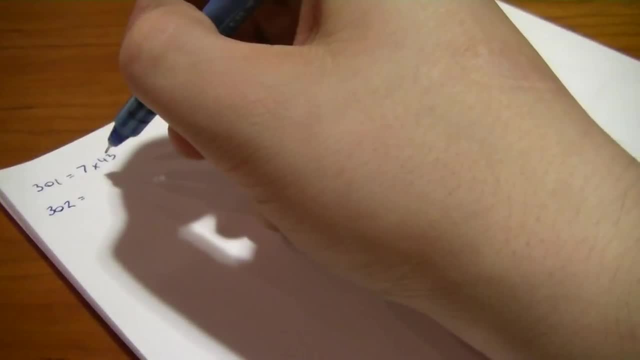 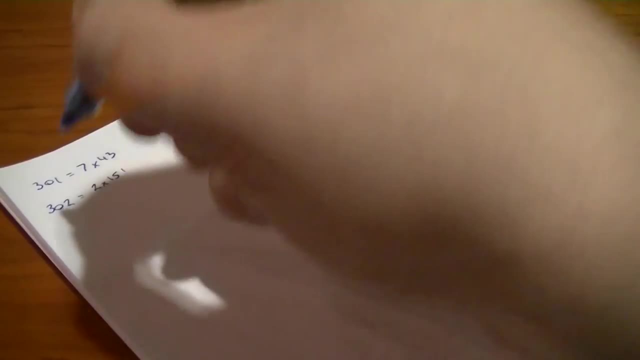 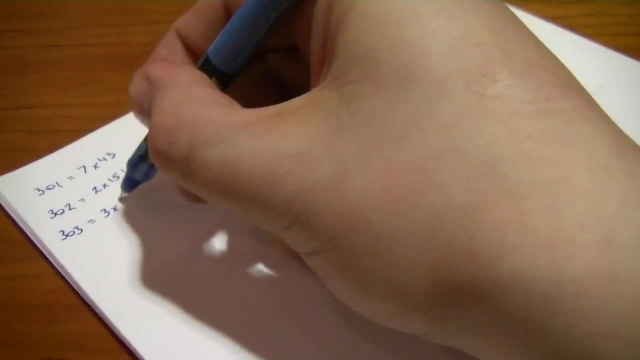 Three hundred and two, That's two hundred and fifty-ones, One hundred and fifty-ones a prime, So that's two by one hundred and fifty-one. Three hundred and three, That's three hundred and ones, Not one's a prime. 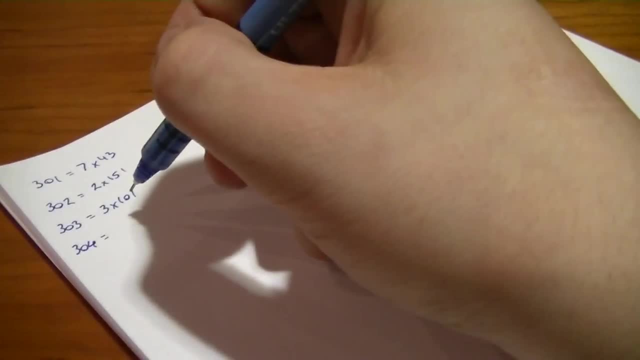 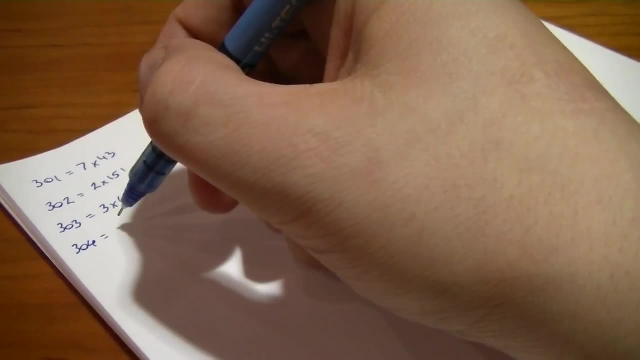 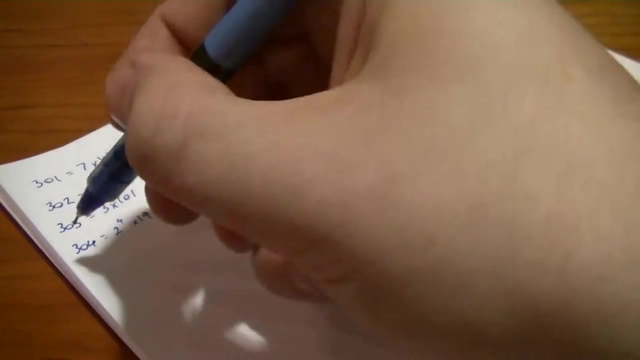 Three hundred and four, That's two hundred and fifty-twos, Which is four, So that's seventy-sixes, Which is eight, Thirty-something others, So what they say. it's two hundred and fifty-twos, Which is two, to the power of four times nineteen. 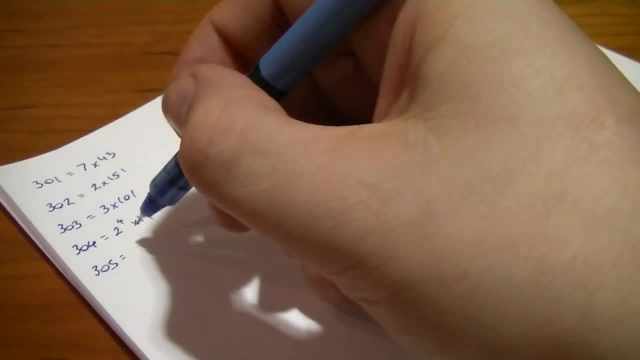 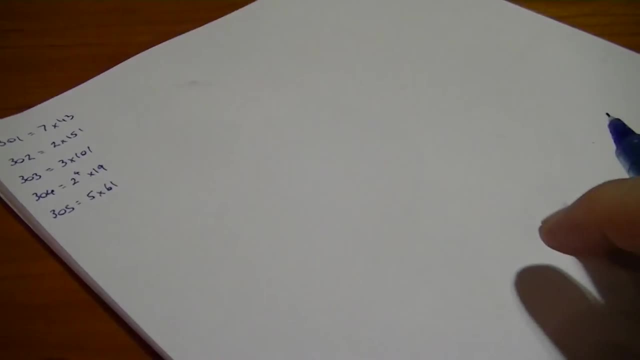 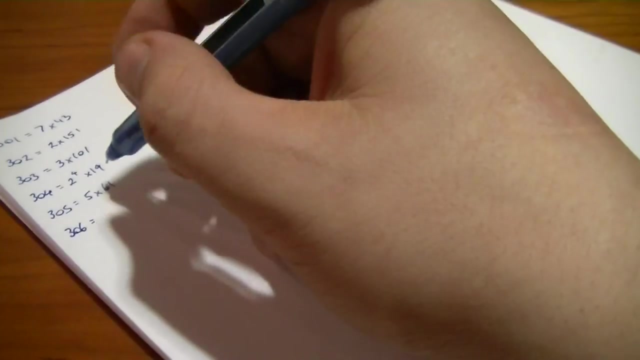 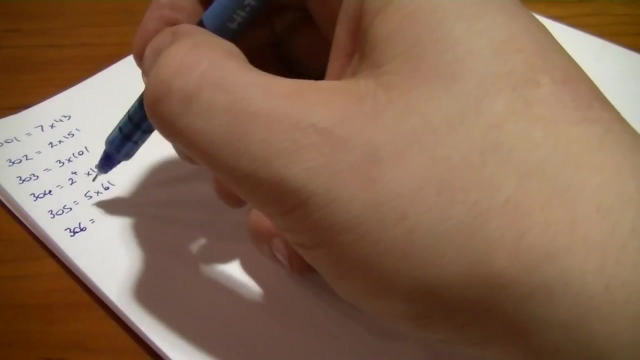 Three hundred and five, That's five, sixty-ones and sixty-ones. a prime. Three hundred and six, That's two hundred and fifty-threes, Which is two by three by fifty-one, Two by three, by three by seventeen. No wait. 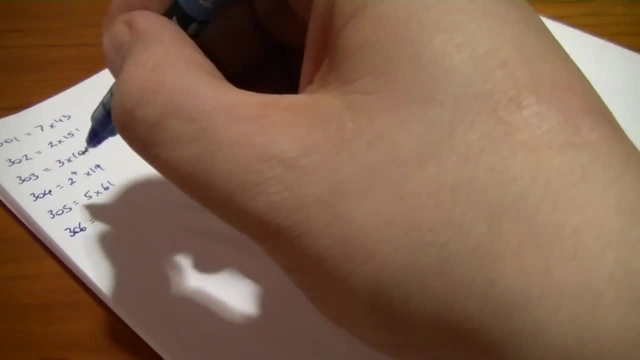 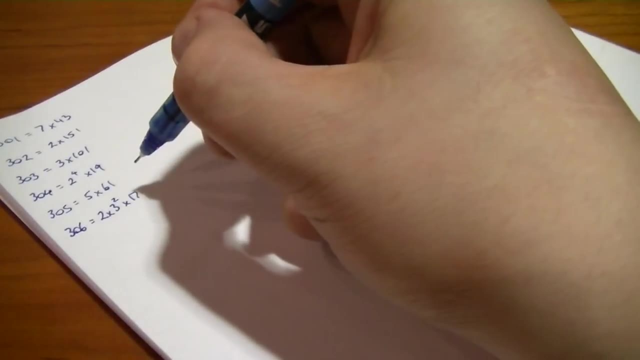 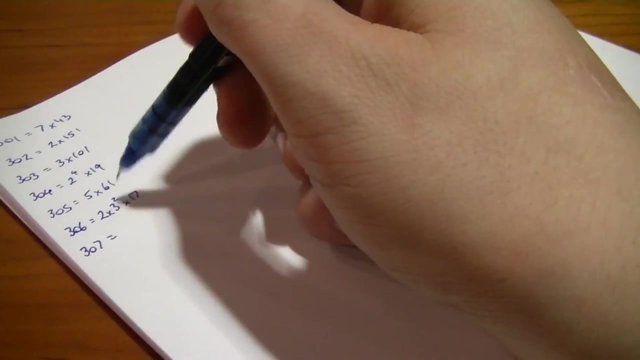 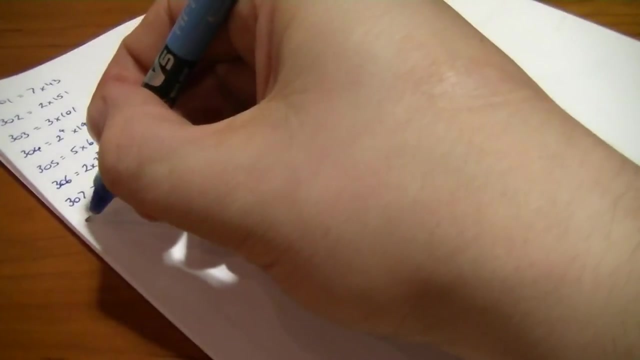 Three hundred and fifty-threes, So that's two by three squared by seventeen. Three hundred and seven, That's built with two or three, or five, or seven, or eleven, Or thirteen, Or is thirteen, No, Or seventeen, So it's a prime. 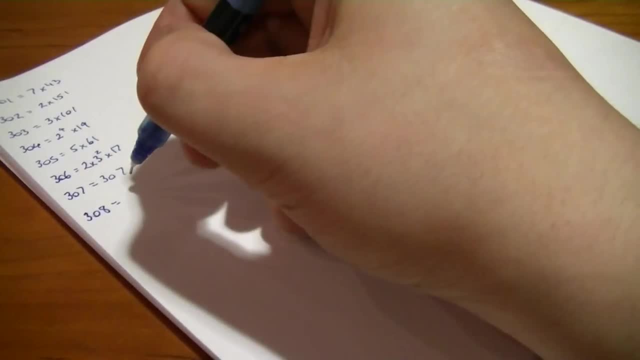 Three hundred and two And eight, That's two hundred and fifty-fours, Which is four seventy. No, two hundred and fifty-fours, Which is four seventy-sevenths, So that's two squared by seven, by eleven, Three hundred and nine. 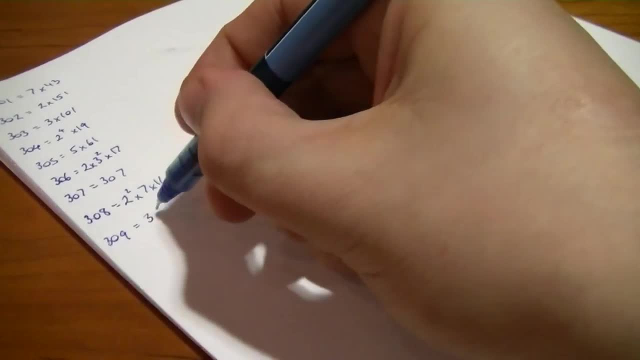 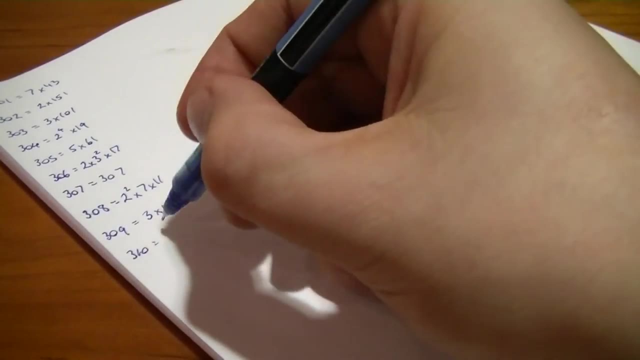 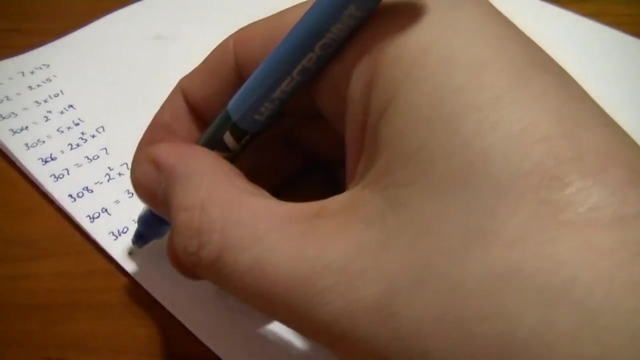 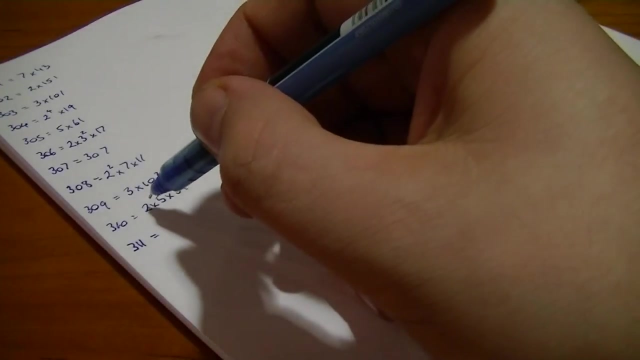 That's three hundred and three. So three's a prime. Three hundred and ten, It's two hundred and fifty-fives. That's two by five by thirty-one, Three hundred and eleven. Not sure how that's divided across in. 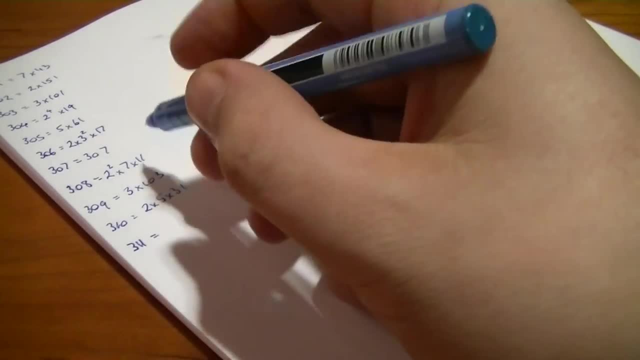 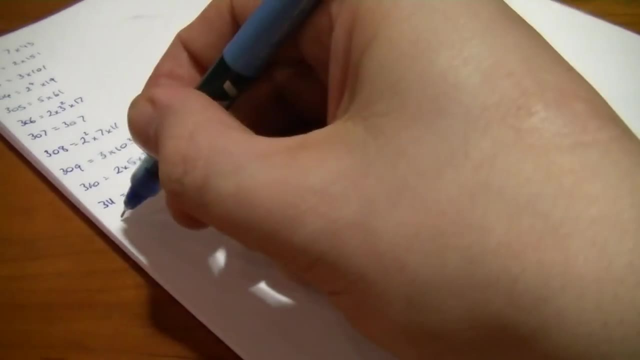 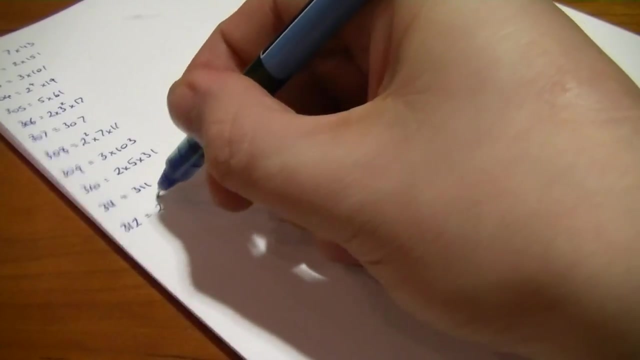 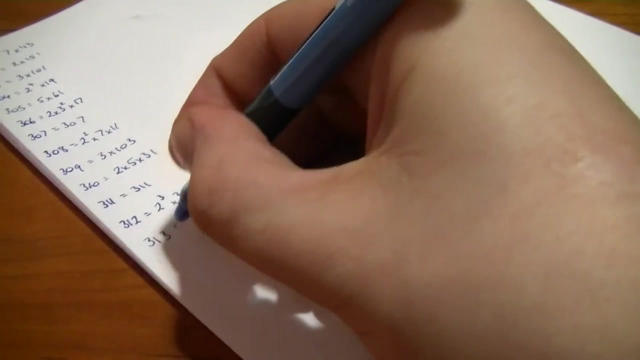 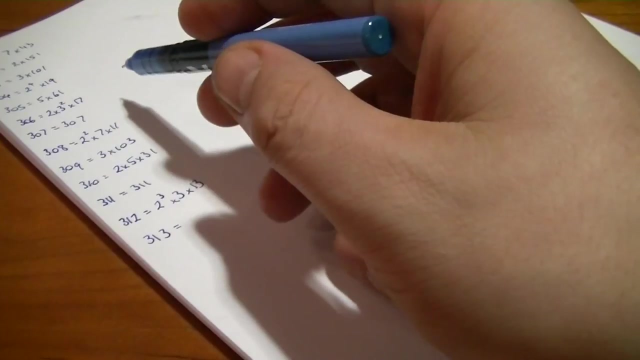 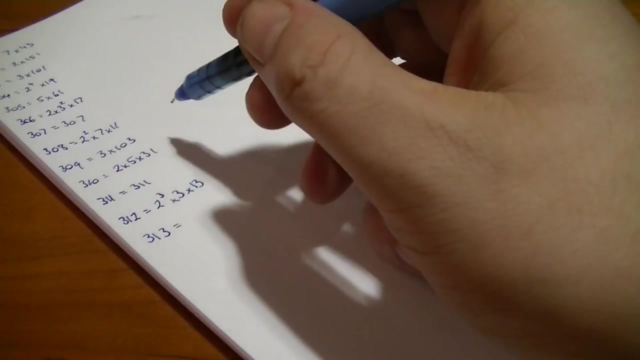 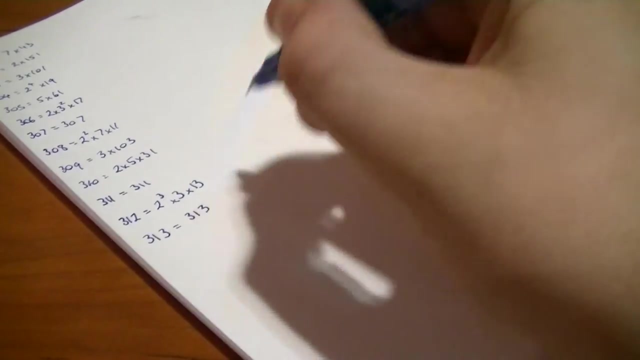 What do we have on the left? Three by three, or five or seven or 11.. There's thirteen again. No, not thirteen by seventeen. So that's a prime. Three hundred and twelve by 13,, 313,. not if it's by 2 or 3 or 5 or 7 or 11 or 13 or 17,. it's not a prime: 314. 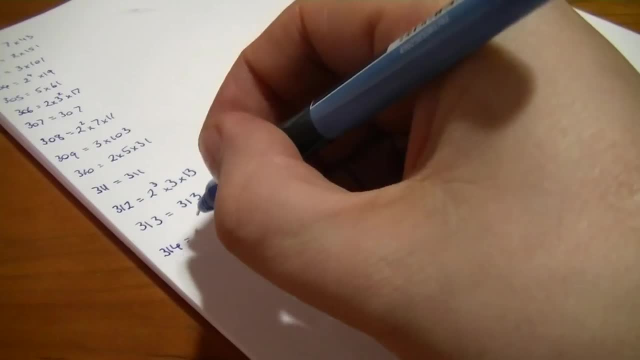 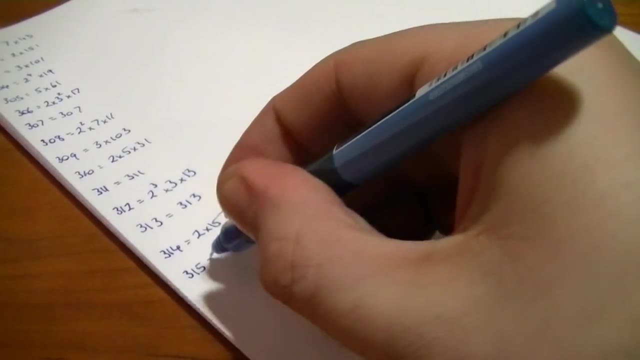 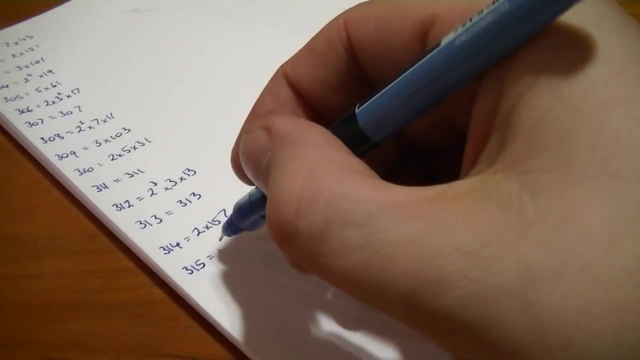 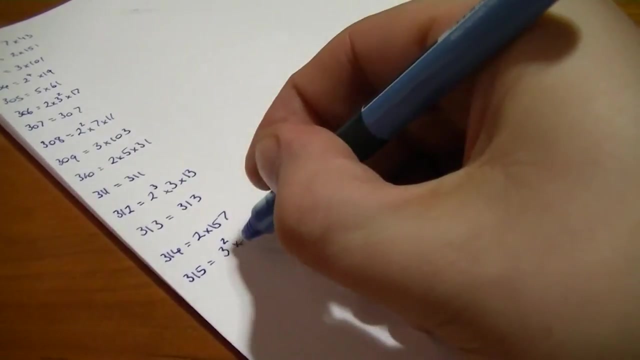 is 2, 157,, that's a prime, so that's 2 by 1, 5, 7, 314, that's 5, 63, and that's 10, so that's 3, 5, 63, so that's 3 squared by 5, 5, 7, 360.. 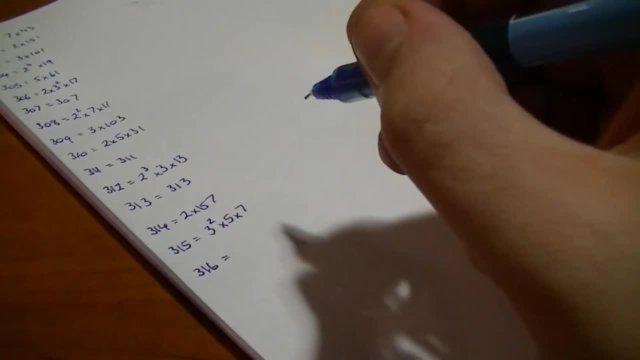 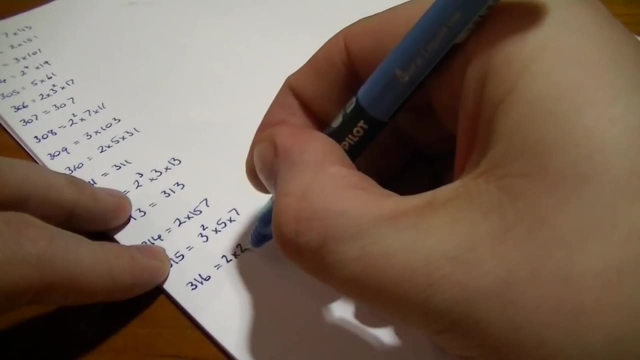 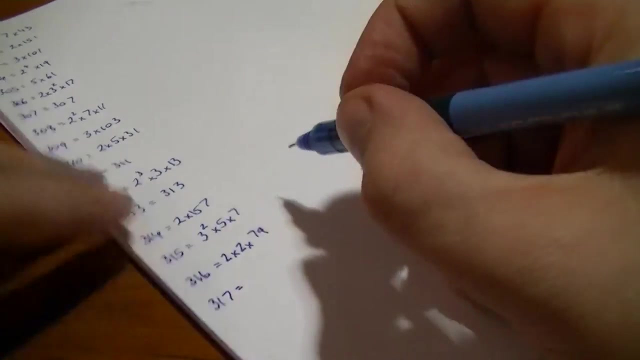 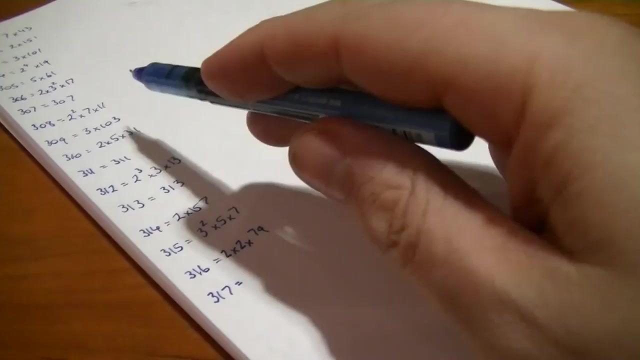 That's 2, 158, so that's 2 by 2, by 79, 317, and that's supposed to be by 2 or 3 or 5 or 7 or 11 or 13 or 17,. so that's a prime. 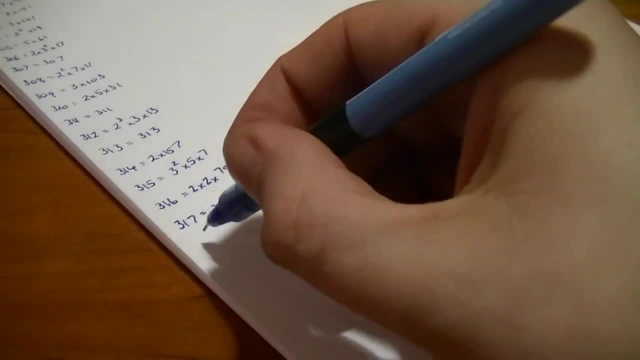 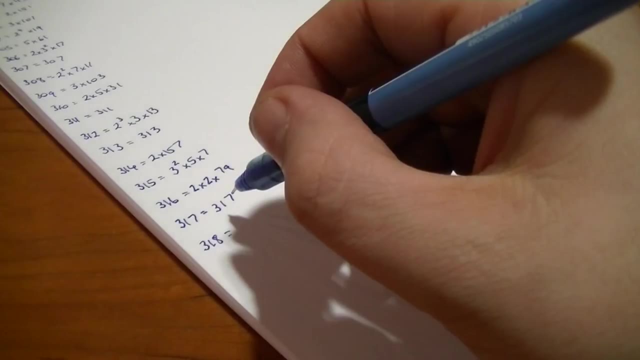 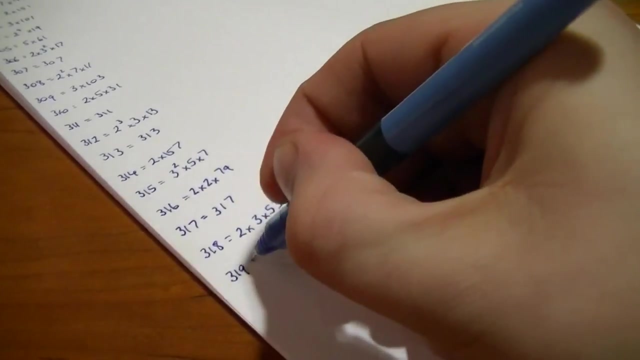 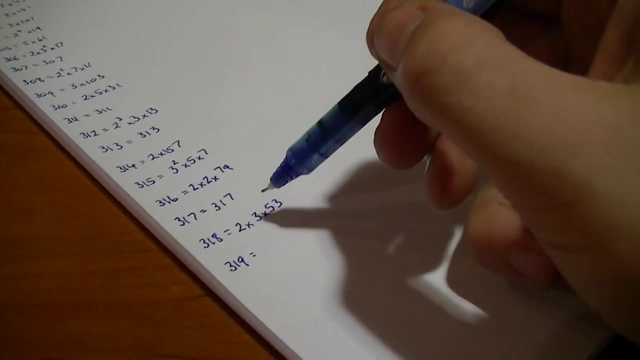 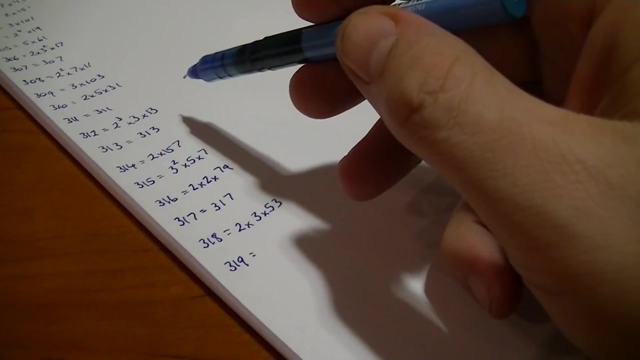 318,, that's 2, 159,, which is 2 by 2 by 159,, 2 by 3,, by 53, 319.. That was by 2, or 3, or 5, or 7,. 318,, which is just by 11,, so that was 28,, so it's 29,. 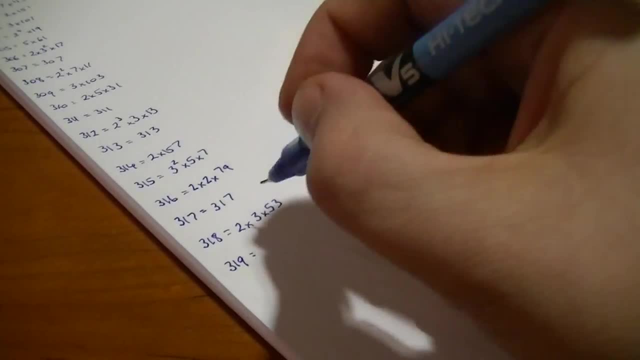 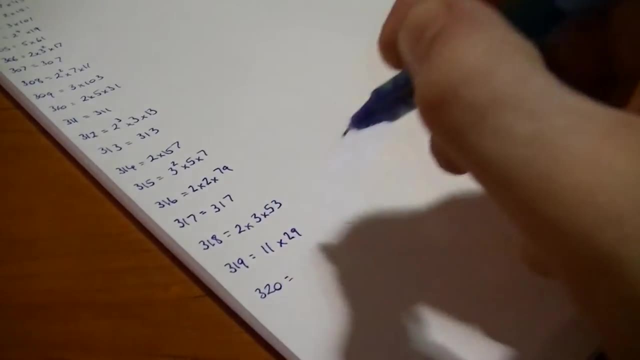 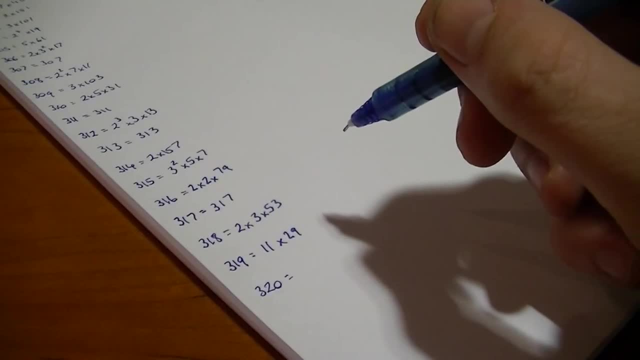 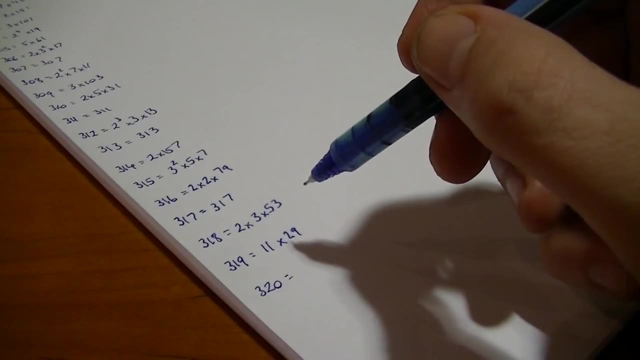 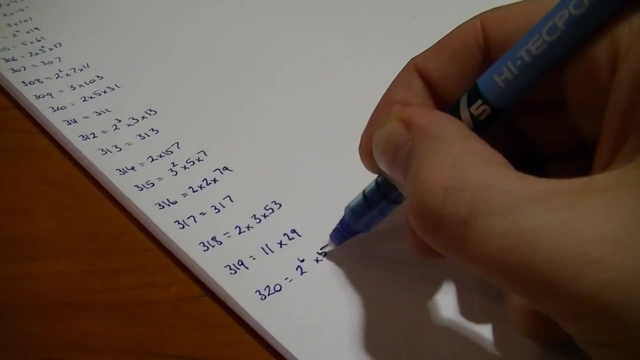 64,. is that right? No, it's not. Kevin, shut up. It's 10, 32's, which makes it 5, 64's. so that's 2 to the power of 6, and that's 5.. 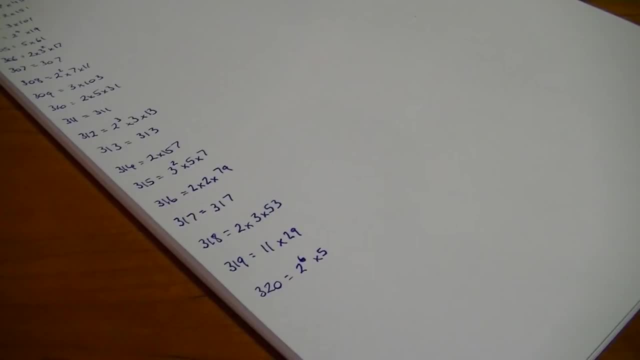 That's not right, Kevin. I'm sure it's not. It's 10.32s, I think it's something towards my eyes now, right, Right, it's 2.60s, 2.60s. I don't know why. that seems wrong to me. 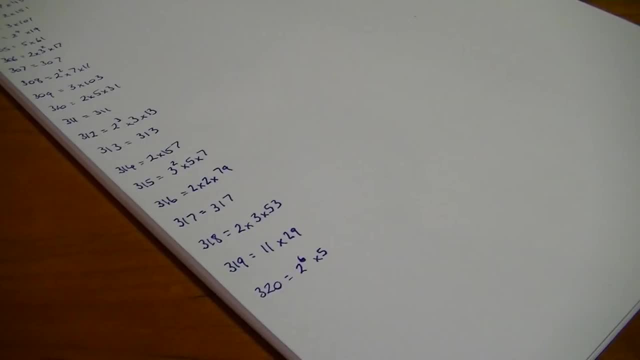 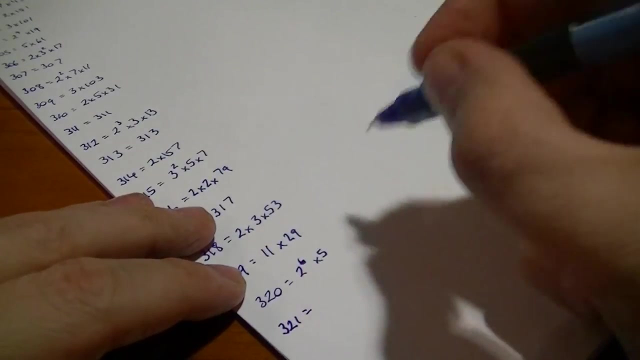 For some reason in my head that should be 72.. 5.35s- 3.60s- Right, okay, never mind, you're more wrong. Okay, 321.. That's 3.107s. 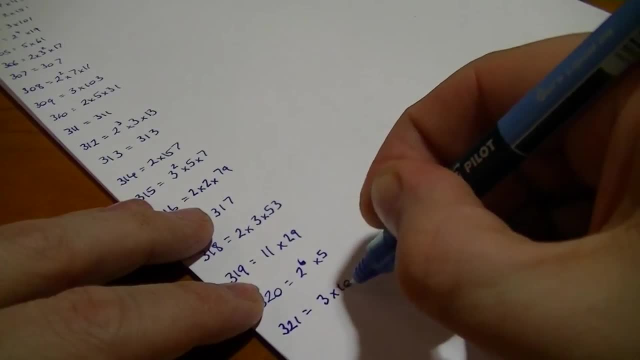 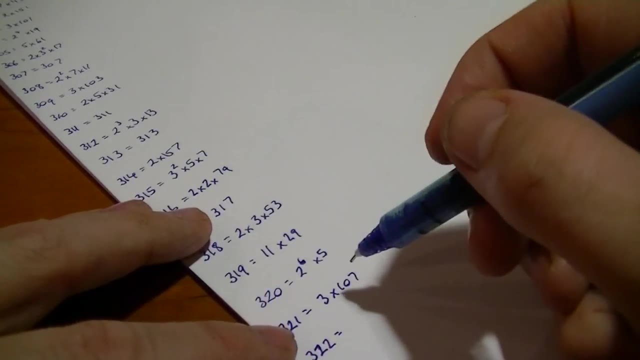 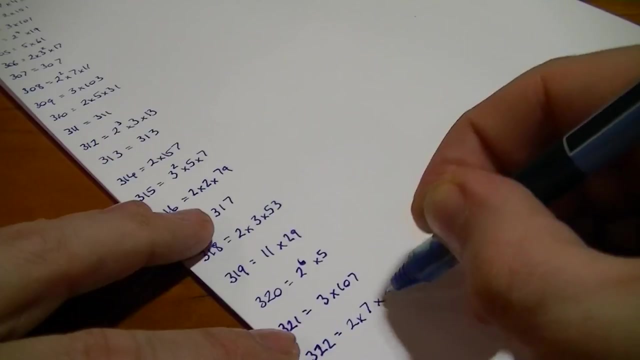 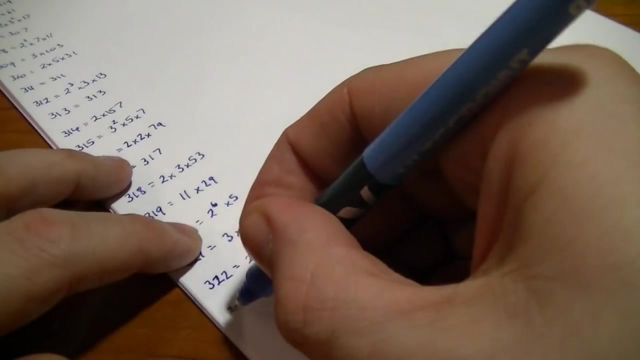 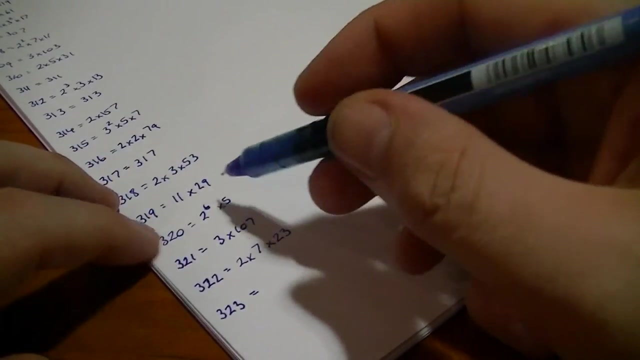 107 is a prime 312, sorry, 322 is 2.161s. So that's 2 by 7 by 23.. 3 times 223.. It's not divisible by 2 or 3 or 5 or 7 or 11.. 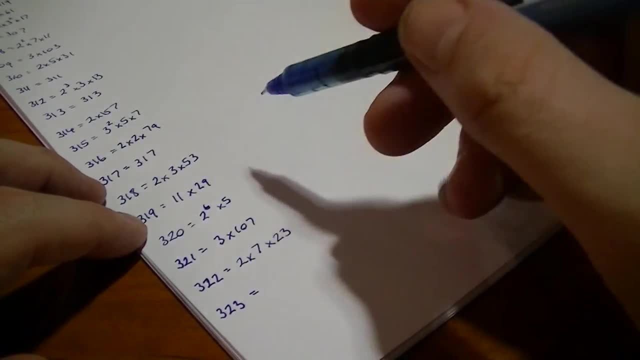 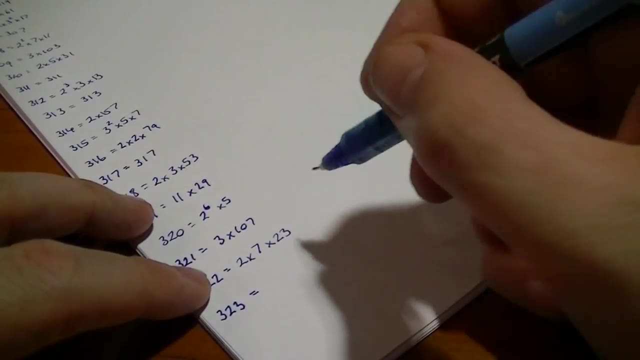 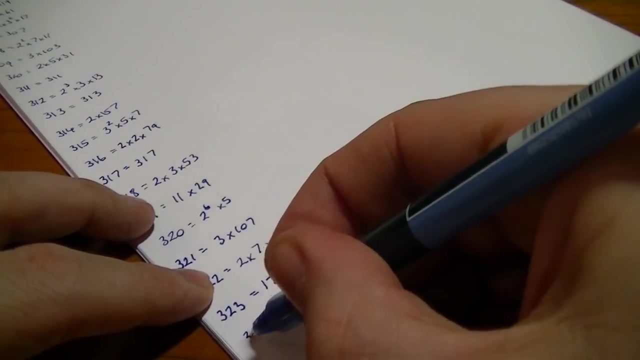 Right, 13. No 17.. Yes, it'd be 17.19s, wouldn't it? Because 17.20s is 3.40s, So that's 17.. By 19., So 324.. 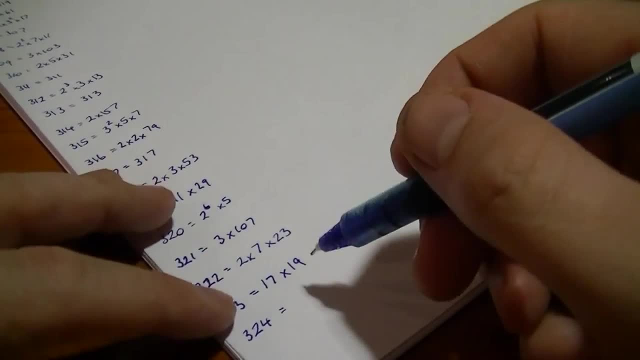 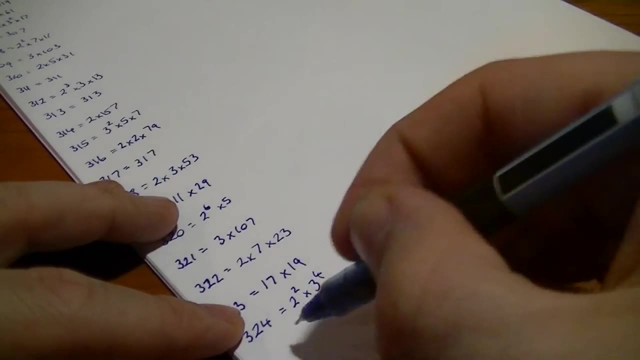 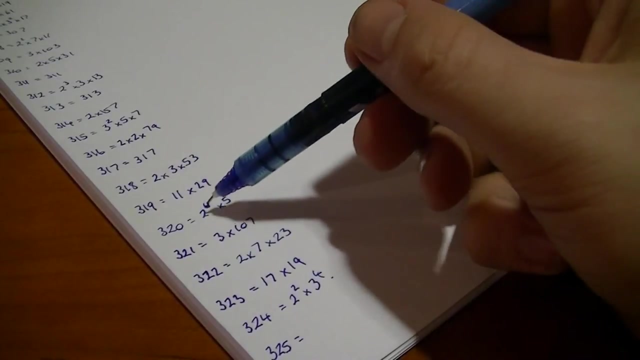 That's 2.. 4. That's 481s. So that's 2 squared by 3 to the power of 4.. And then 325.. That's 5.. That was 32.. So that's 5.33s. 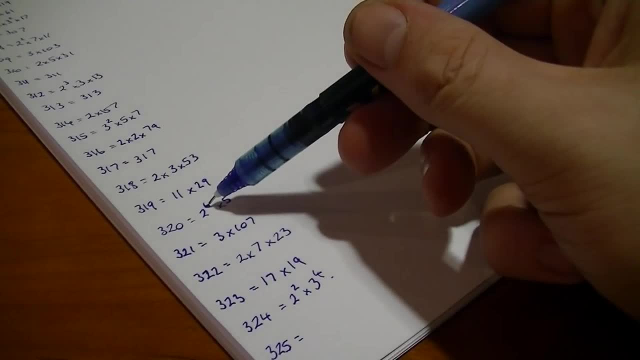 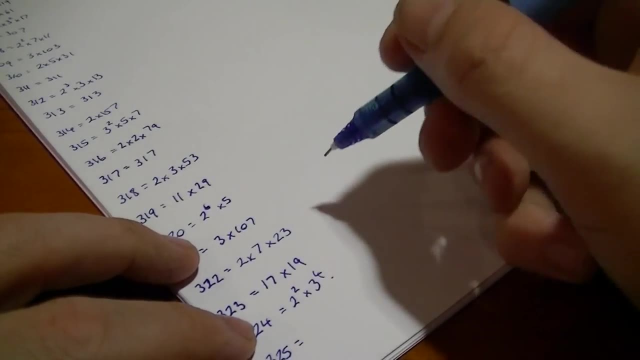 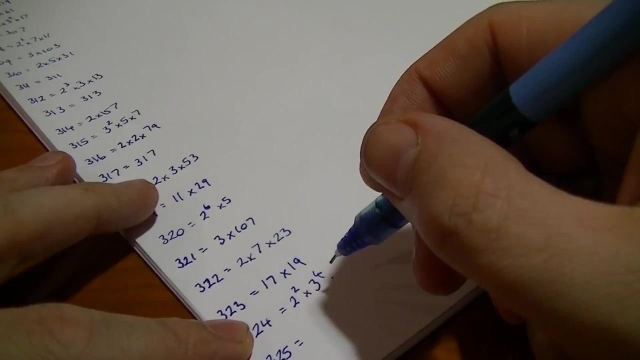 No, that's not, That's 5.64.. So that's 5.65s. 5.65s, So that's 13.. That is a fifth, So 13.25s, 13.25s. 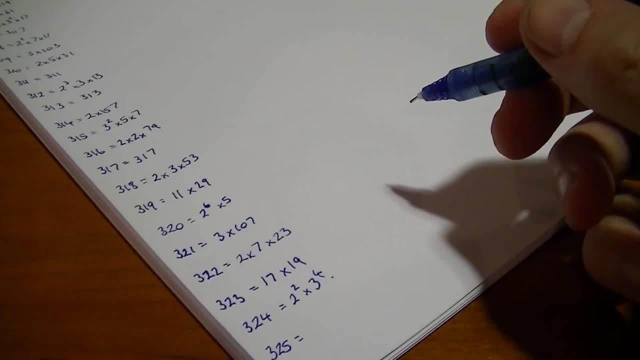 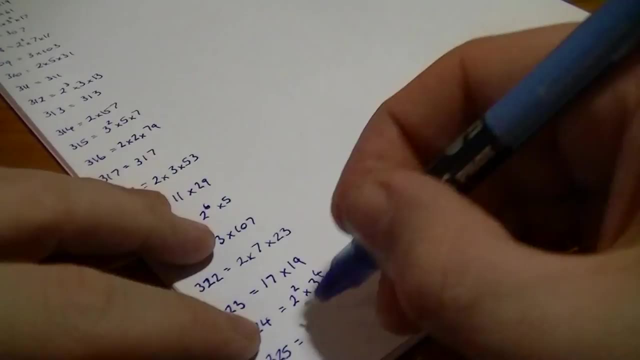 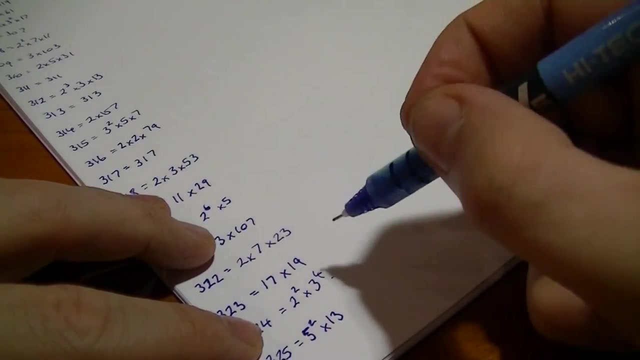 13.25s, 13.25s, 13.25s, 13.25s, 13.25s. So that's 5 squared. So that's 5 squared times 13. times 13. Yep. 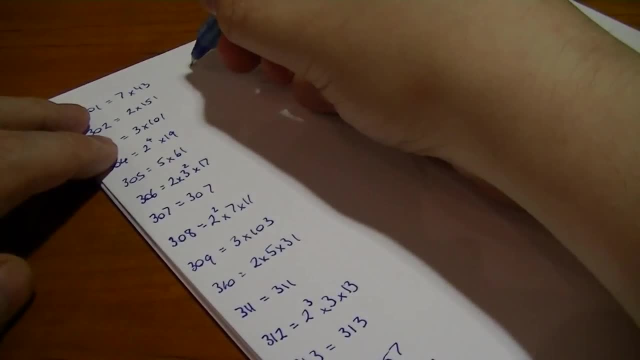 Okay. 326.. 326.. That's 2 162s, That's 2 163s, That's 2 163s. 163s a prime, 163s a prime. 327.. 327.. It's not divisible by. 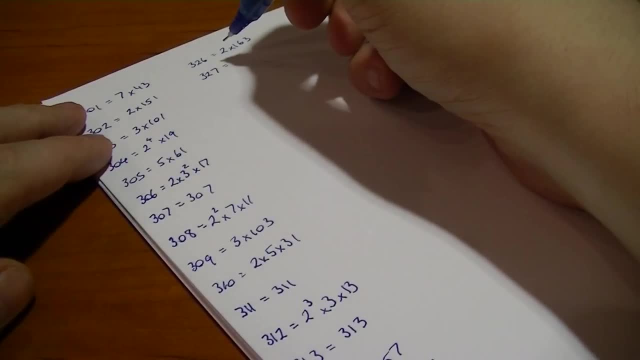 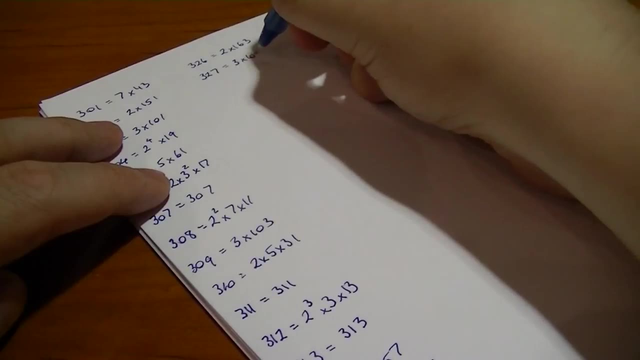 It's not divisible by, It's just divisible by 3.. It's 3, 109s, 109s, a prime 109s, a prime 328.. 328.. That's 42. 41. 44. It's 2 to the power of 3.. 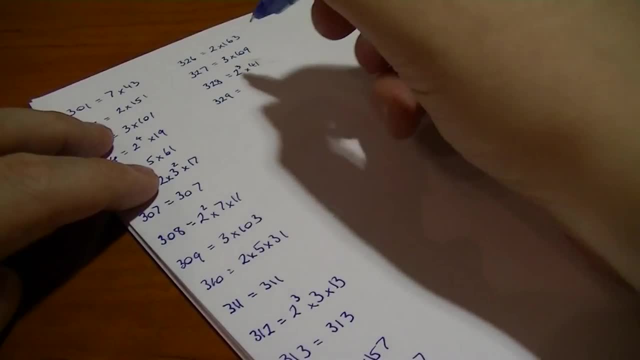 That's 41.. 349.. Let's see. Let's see: Not divisible by 2 or 3 or 5.. Not divisible by 2 or 3 or 5.. Not divisible by 2 or 3 or 5.. 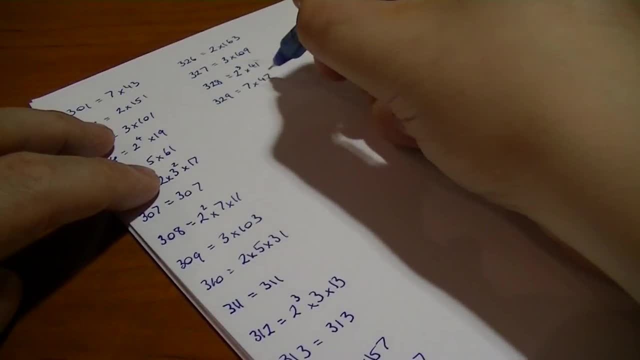 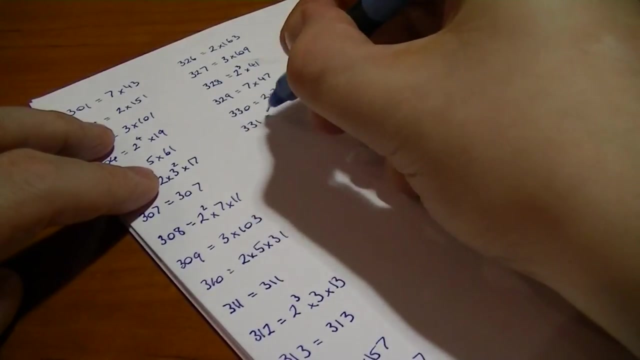 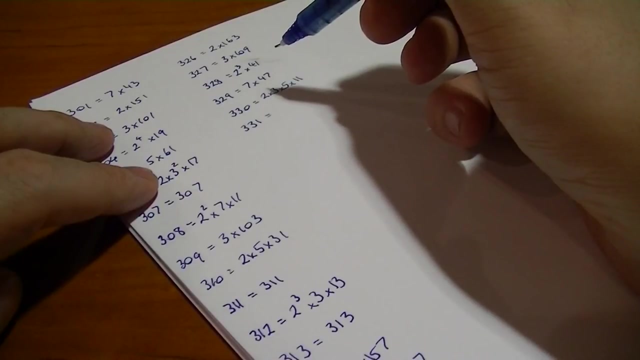 That's 7.. That's 46.. That's 47.. 7.. That's 310.. Another 10 is 2 by 5 by 11.. So it's 2 by 3 by 5, by 11.. 331.. It's not divisible by 2 or 3 or 5 or 7 or 11.. 13,, no 17,, no, So that's a prime. 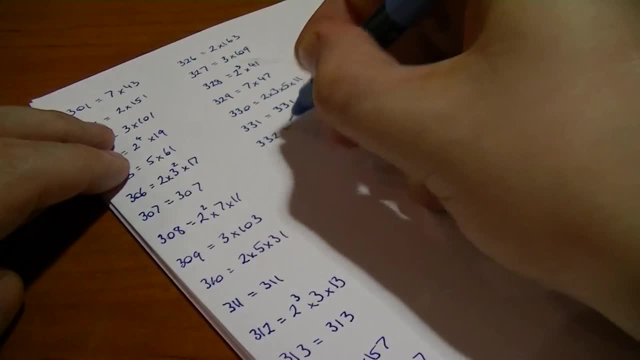 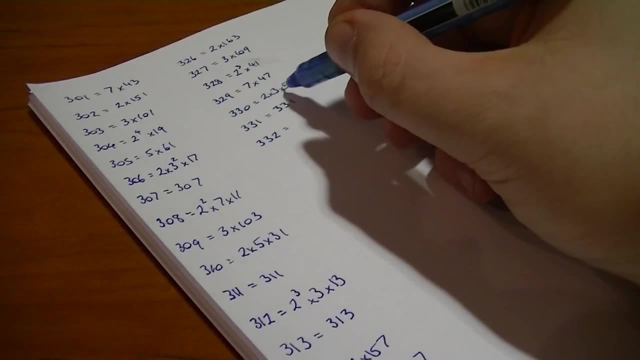 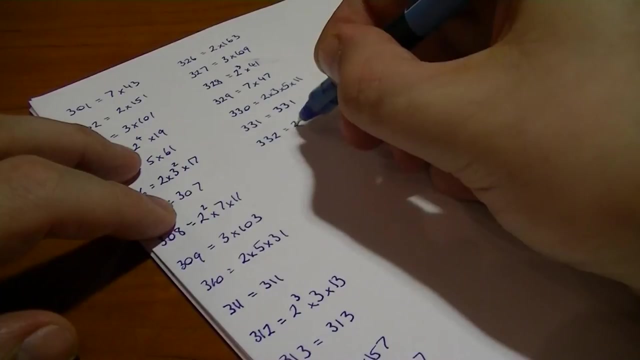 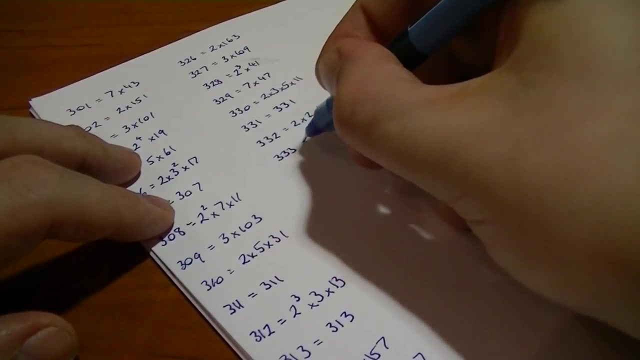 332.. That's 2.. Let's see that was 265, 266.. 266.. So that's 2 by 2 by 83.. 3, 3, 3 is 3 times 111, which is 332.. 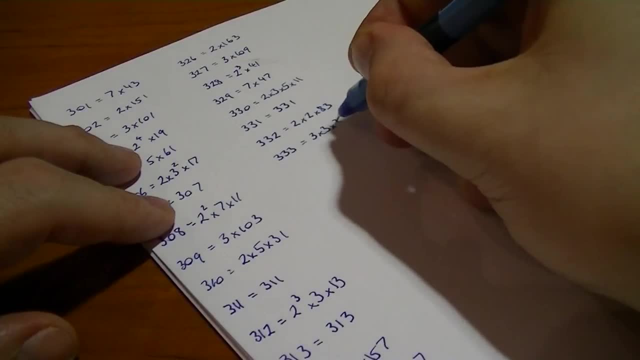 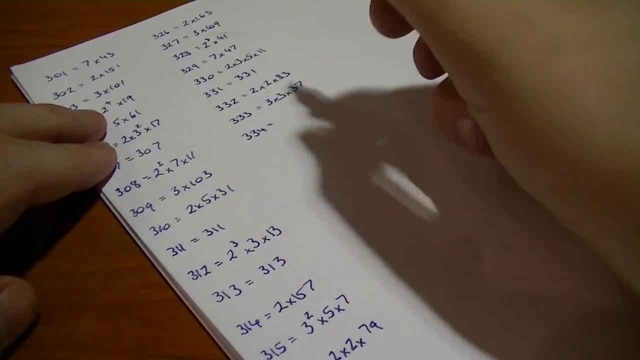 That's 3 by 3 by 37.. 334.. Well, let's see that was 166, so that's 167.. And 167 is a prime, so it's 2 by 1 by 6 by 7.. 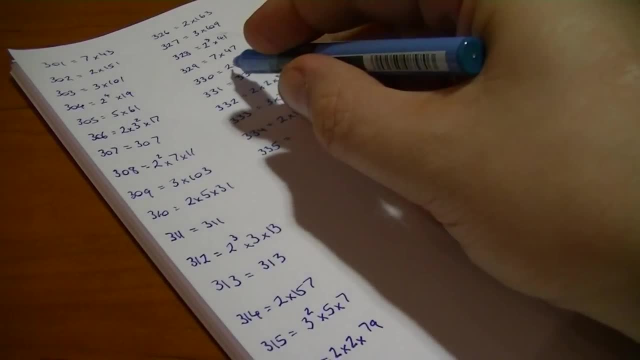 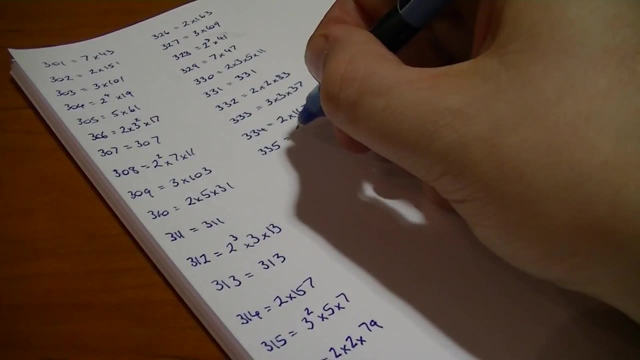 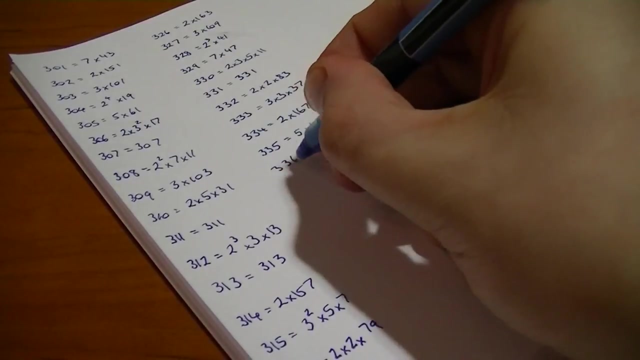 335.. Well that was, That was 3 by 3 by 37.. That was 6, 66,, so that's 67.. So that's 5, 67.. 67 is a prime 336.. 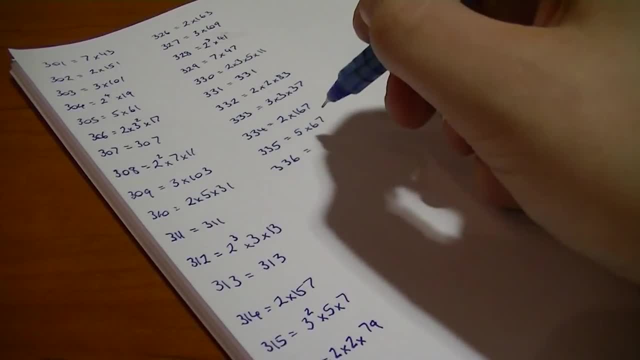 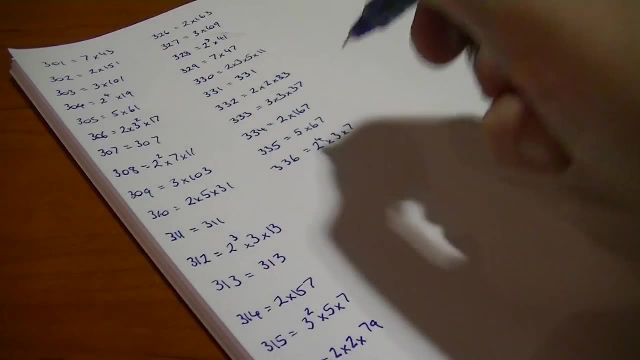 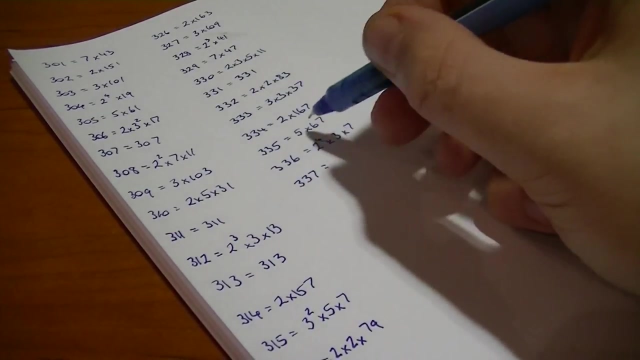 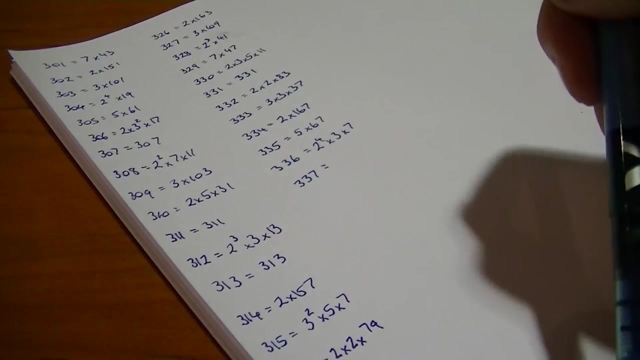 That's 268.. 168 is this, That's 2 to the power of 4 by 3 by 7.. 337.. That's not divisible by 2 or 3 or 5 or 7 or 11 or 13 or 17 or 19.. 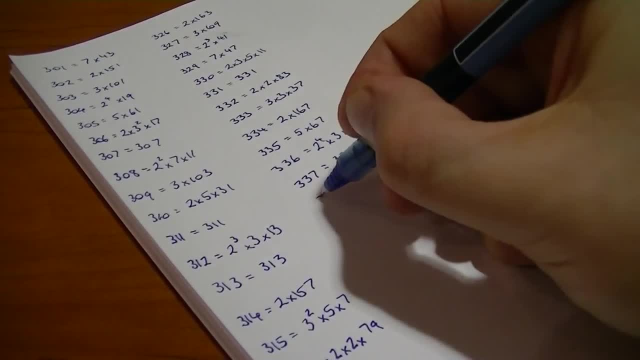 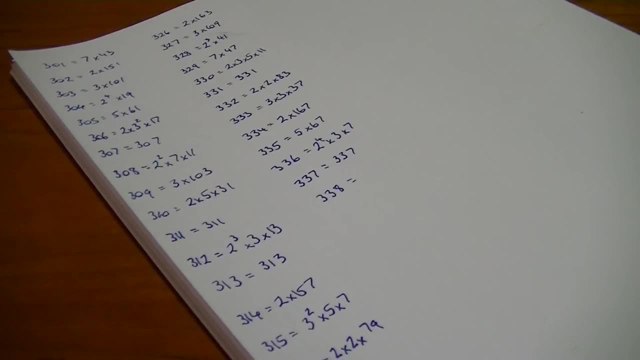 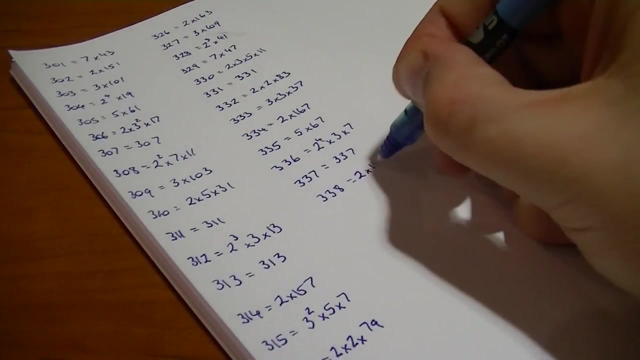 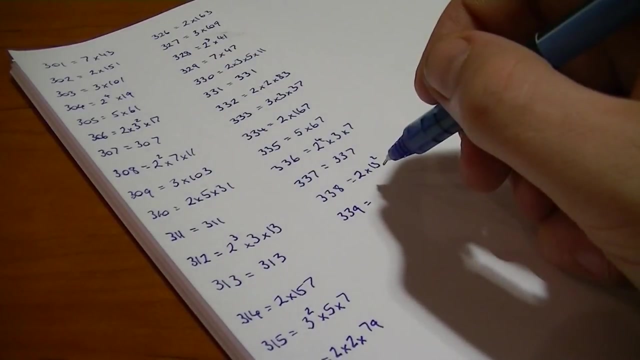 So that's a prime 338.. That's 2.. 169.. That's 13 squared. So that's 2 by 13.. Okay, 339.. That's 3 times 113.. 113 is a prime. 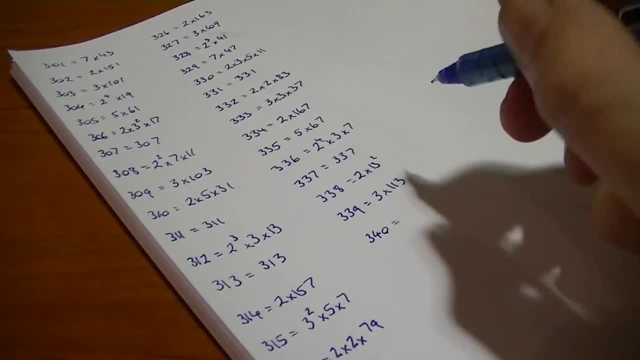 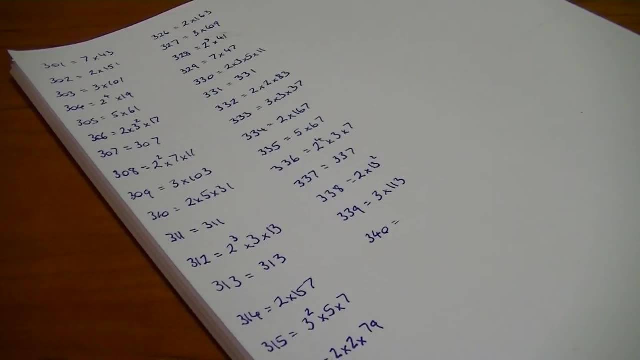 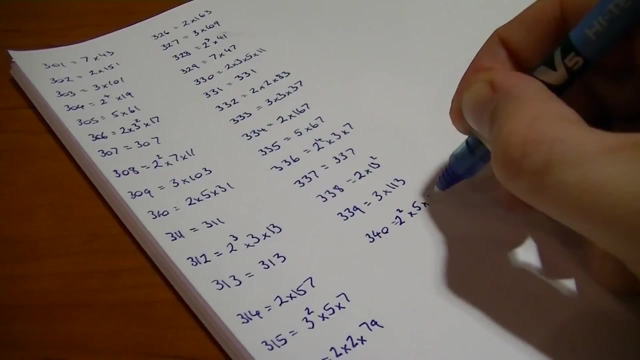 340.. That's 270.. Which is 485.. No, it's not, It is 485.. Yeah, 45.. 485.. And 85 is 5, 17s. So that's 2 squared by 5 by 17.. 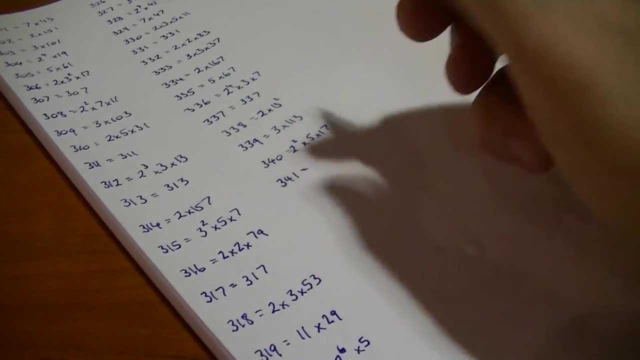 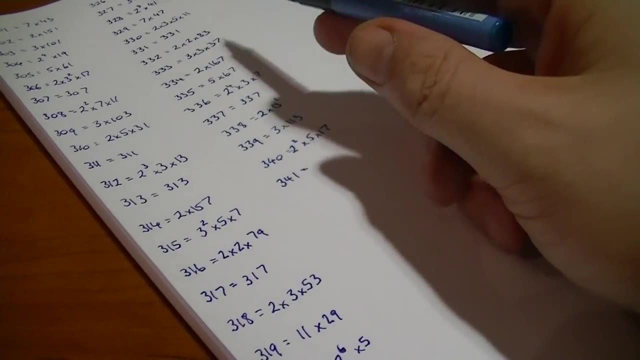 So now you have 341.. Not divisible by 2 or 3 or 5 or 7. It is divisible by 11. So that was 6, 30, 31.. 11, 31. So that's 11 by 31.. 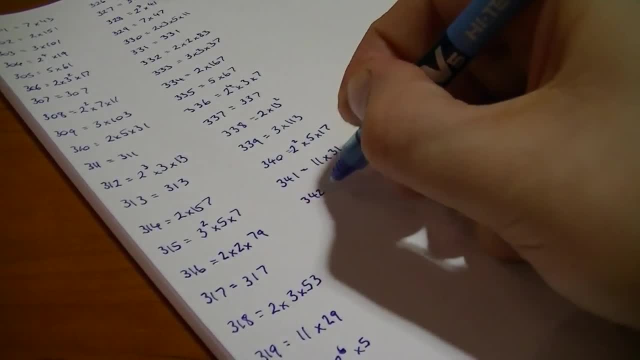 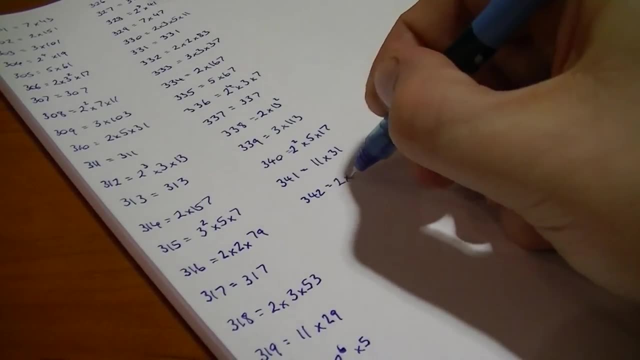 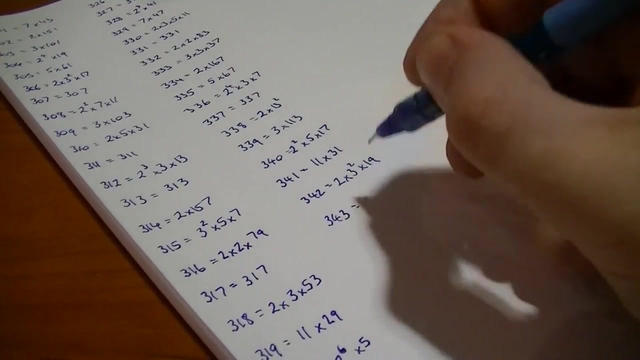 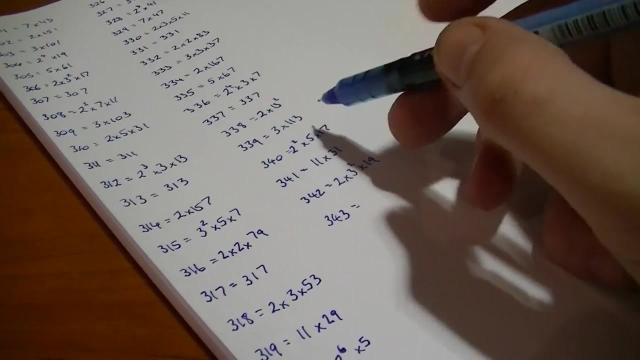 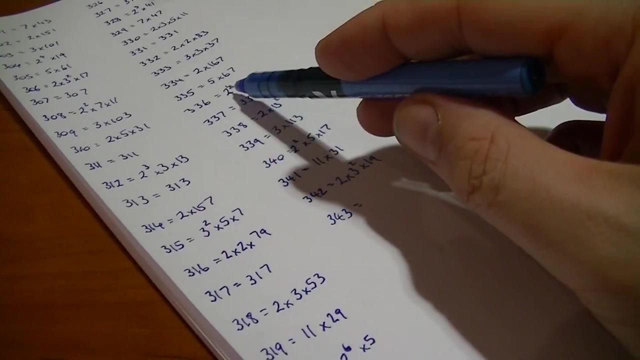 31. 342 gets 271.. 171, now, what is really All that's behind me is 3 divided by 12.. 343, That's 2 or 3 or 5, And this was probably 7. Let me see that was 1648. 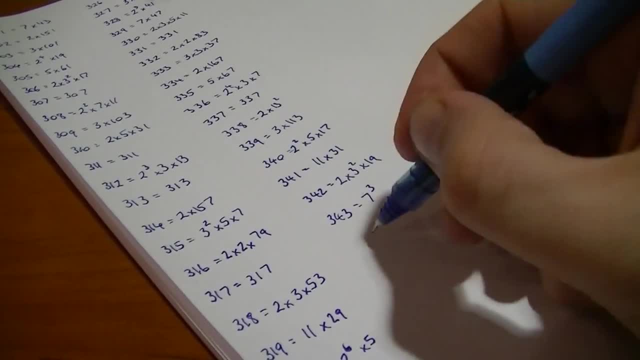 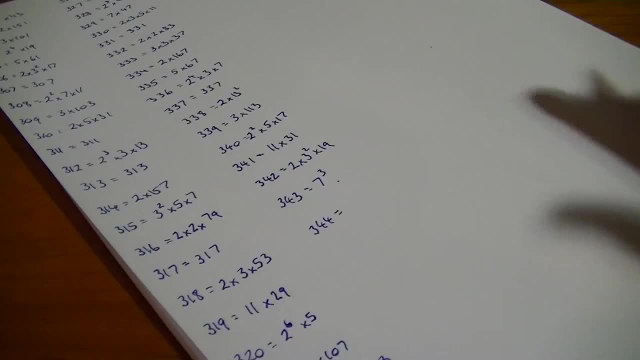 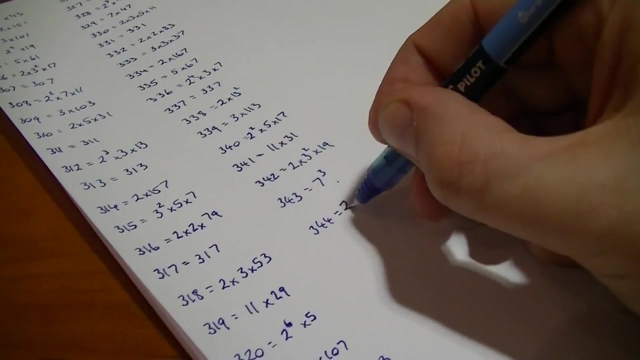 749,. oh yeah, 7, cute 344.. It's like: oh yeah, I remember that. Oh, you're a friend of mine. Anyway, 344 That's doing 172's. 172 is a lot, So that's 2 cubed by 43. 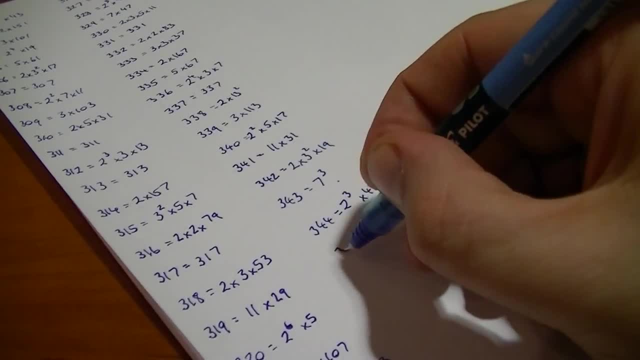 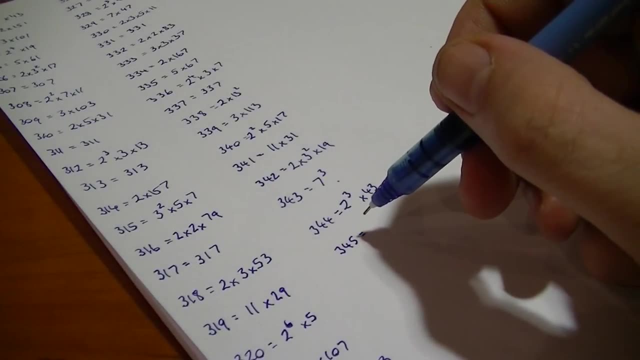 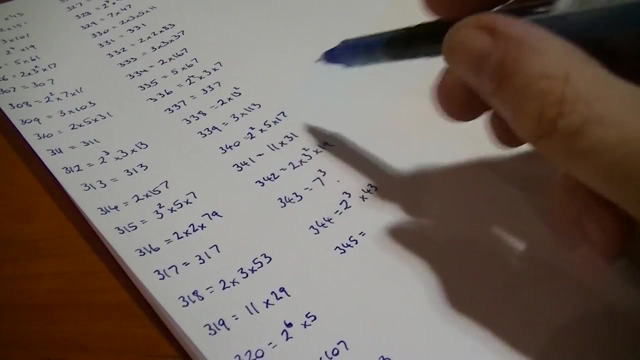 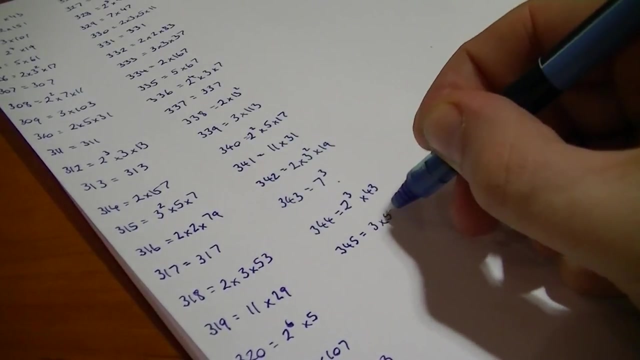 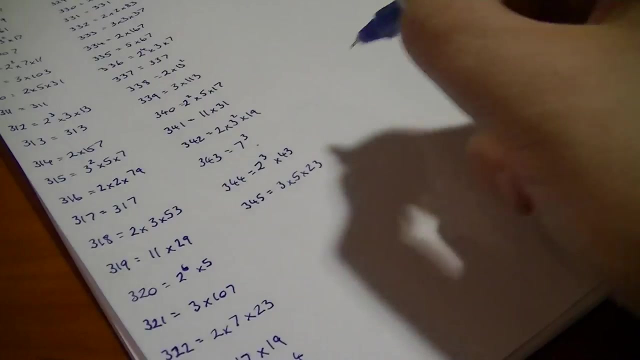 You had 43's, Yeah, that's right. 345, That's 5, 568, 568, 569's, 323's, So that's 3 by 5, by 23, And this is actually starting to get rather mentally taxing. 346. 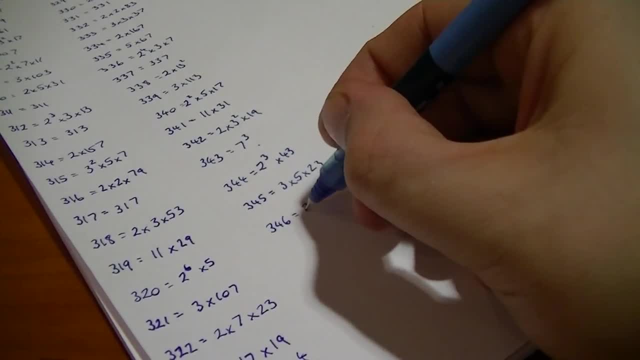 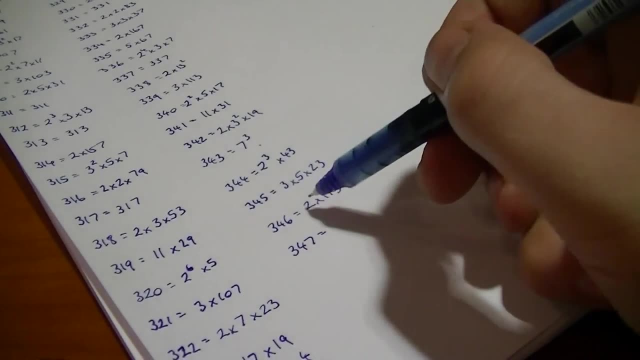 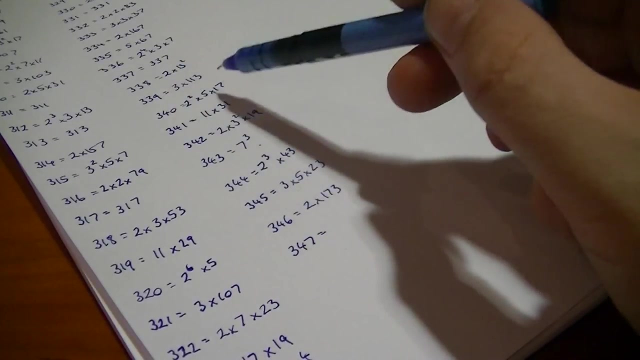 That's 2, 173's, 173 is a prime- 347, 347, So that's about 2 or 3 or 5 Or 7 or 11 Or 13 or 17 Or 19, So that's a prime 348. 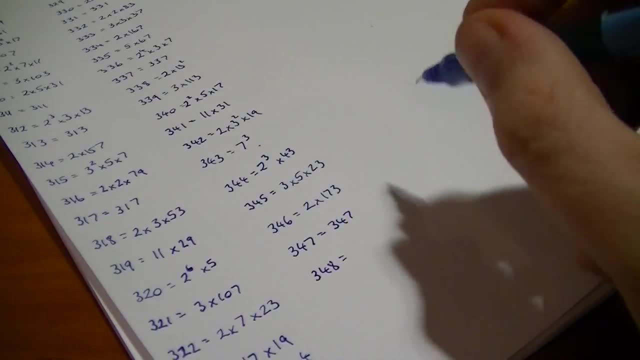 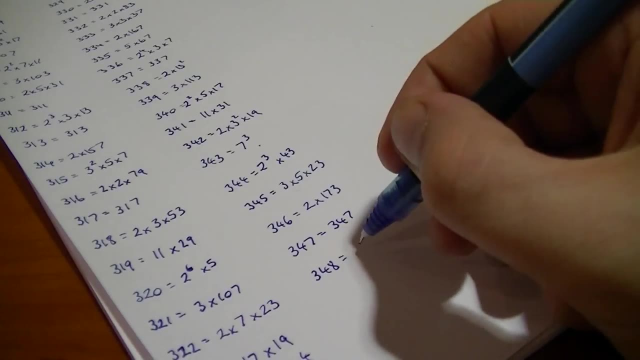 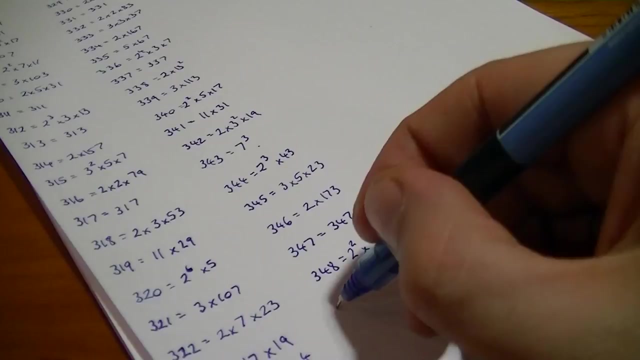 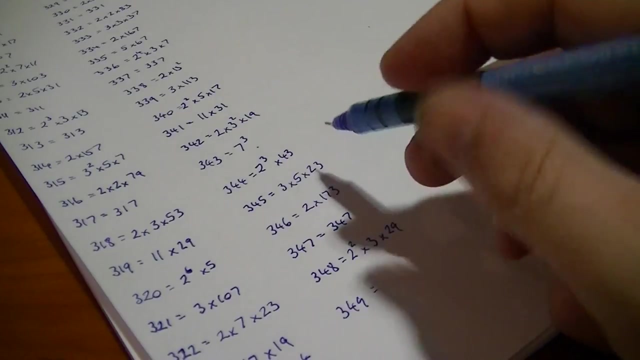 348, That's 4, something's That's 274's, 274's 174, is that? So that's 2 squared By 3, By 29, 349, 349, And not divisible by 2 or 3 Or 5 or 7. 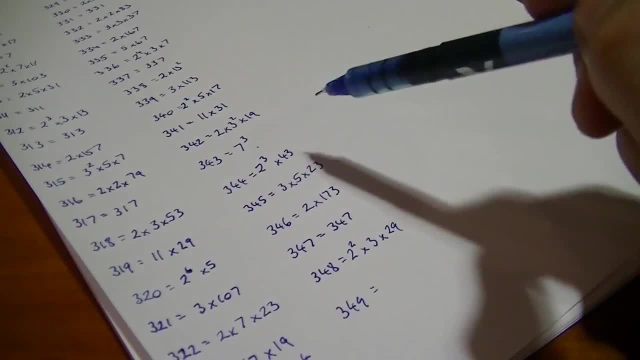 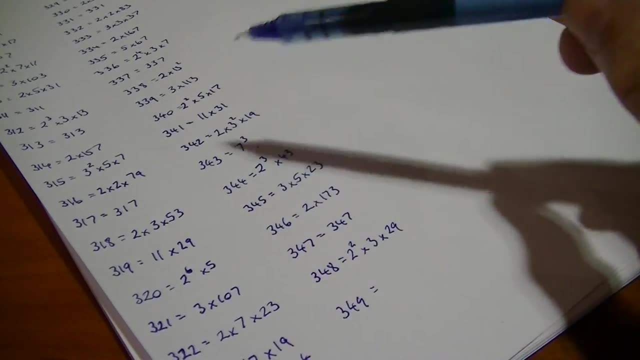 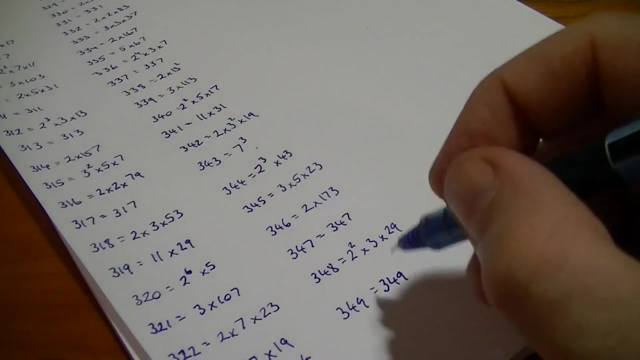 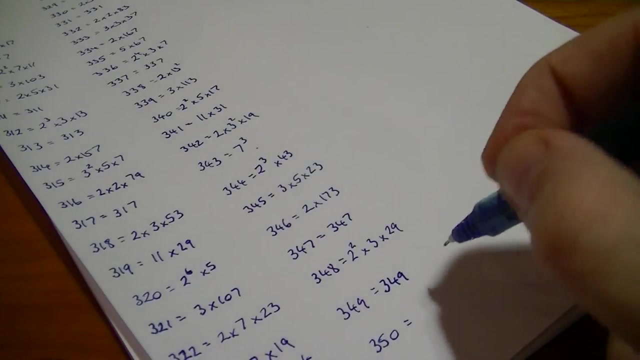 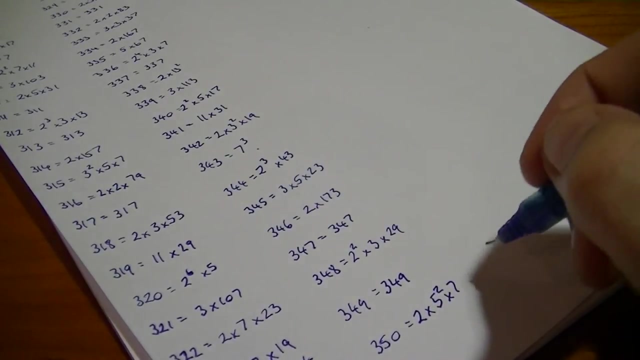 Or 11 Or 13, Or 13 Or 13 Or 17, Or 17 or 19, So that's a prime, Okay, Okay. 350, That is 1075's, 1035's, So that's 2 by 5 squared By 7. 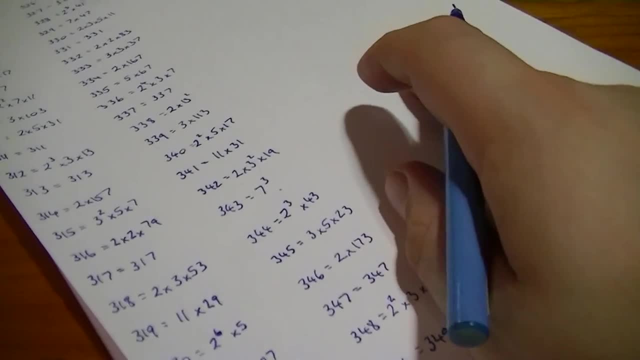 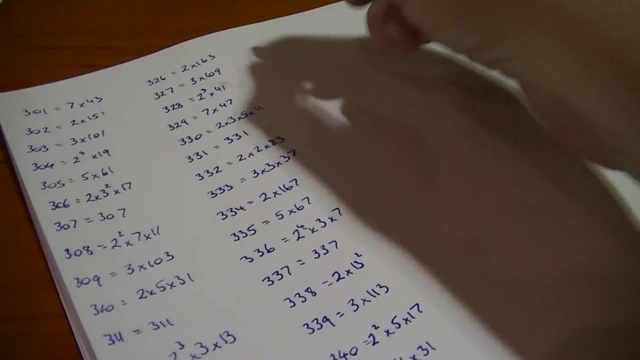 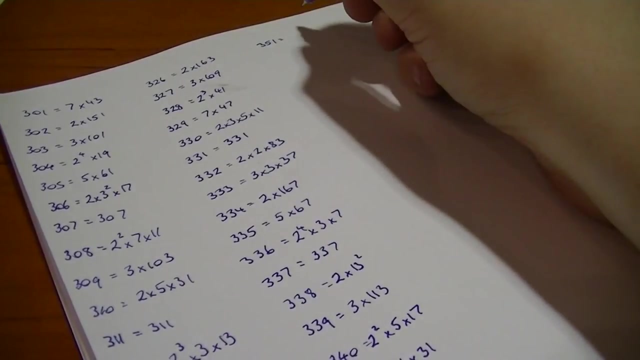 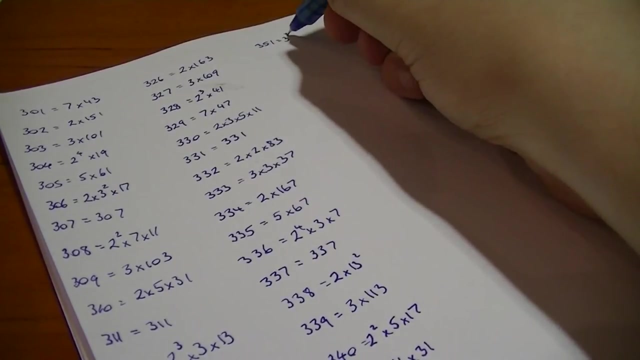 Okay, Okay, Okay. Let's see 351. 351, That's 317's, That's 317's, And 117 is 9- 13's, And 117 is 9- 13's. So that's 3 cubed by 13. So that's 3 cubed by 13. 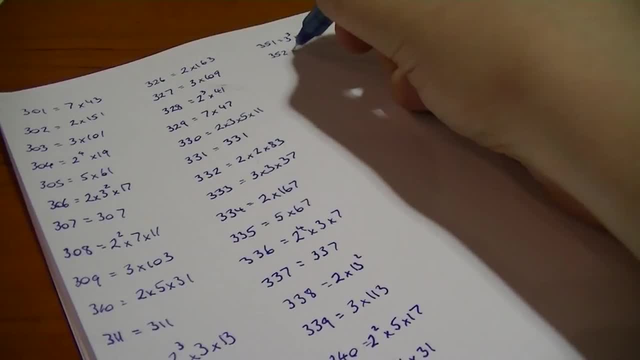 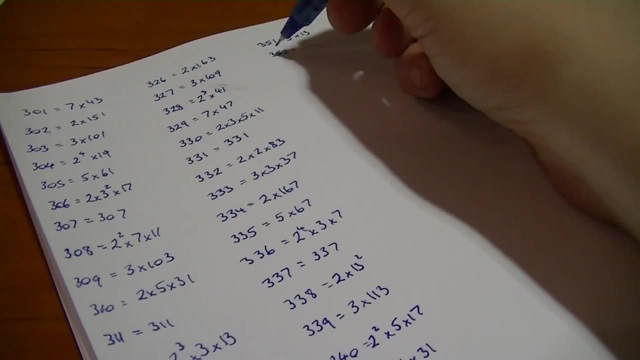 352, 352, So that's 2, So that's 2, 176's, 176's, 176's, 176's. That's 2 to the power of 5, That's 2 to the power of 5 By 11, Alright, 1132's. 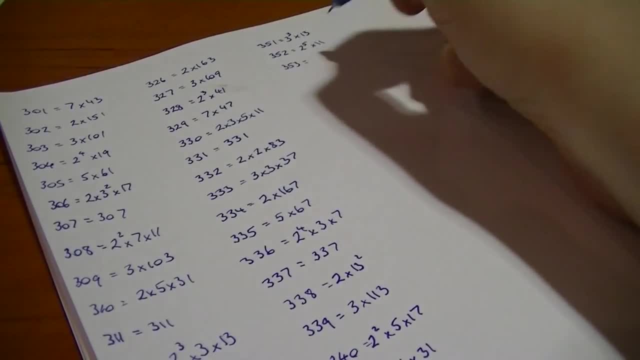 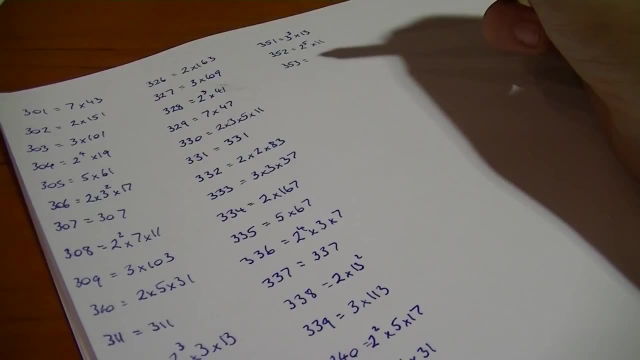 353, 353, Not divisible by 2. Not divisible by 2 or 3 or 5 Or 7 or 11 or 13 Or 7 or 11 or 13 Or 17 Or 17 Or the last 17 There. Okay, so that's a prime. 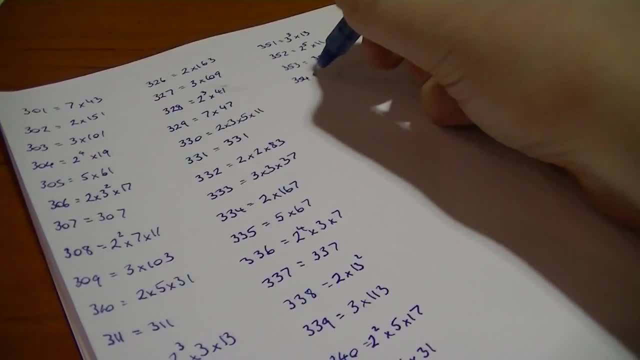 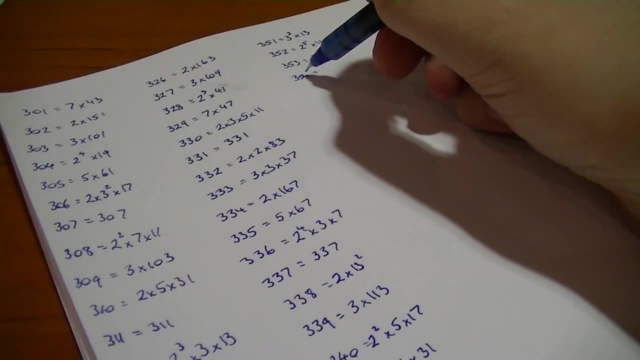 354, 354, 354, And that's 2, And that's 2, 160, 160, 177, 177, So that's 2, So that's 2 by, So that's 2 by 3, by 3 by 59 355. 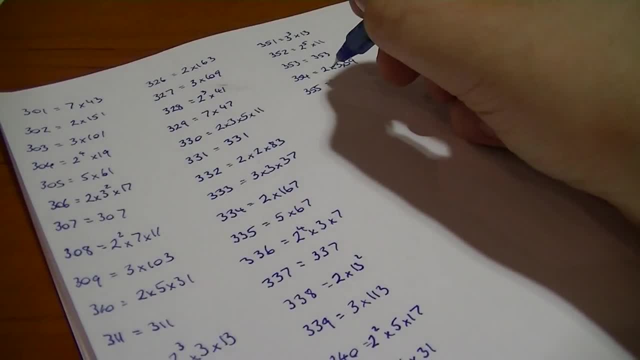 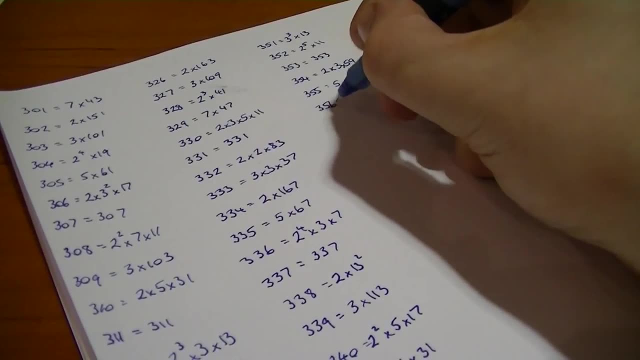 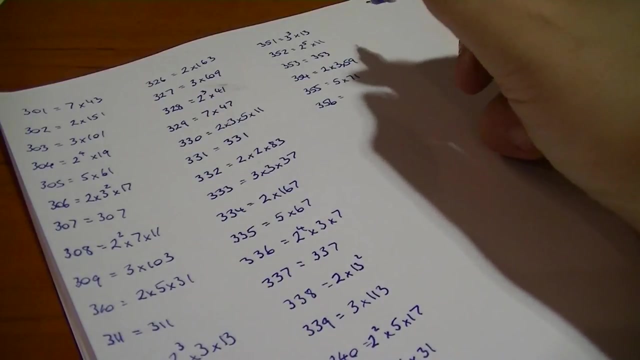 371, 371, 371, 371, 356, 356. That's 2, That's 2 times That's 2 times. That's 2 times 100, 178, 178, 178, 178 Is 2x2x89, Is 2x2x89. 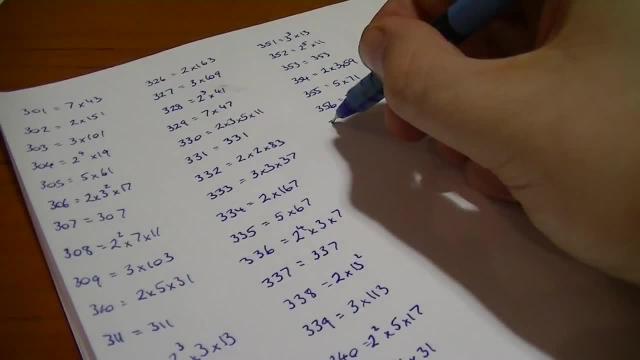 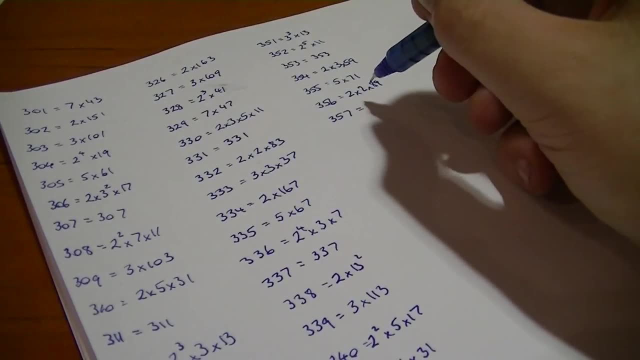 Is 2x2x89 357 357 357. That's 3 times 119. That's 3 times 119. 119 is 7x17. 119 is 7x17 3x7x17 358 358. 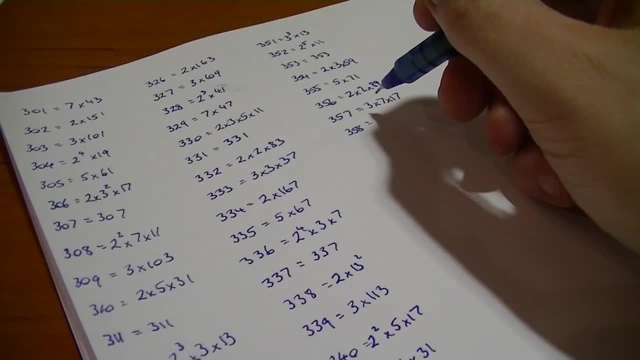 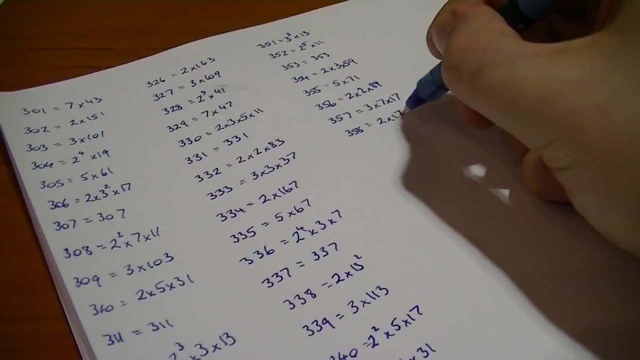 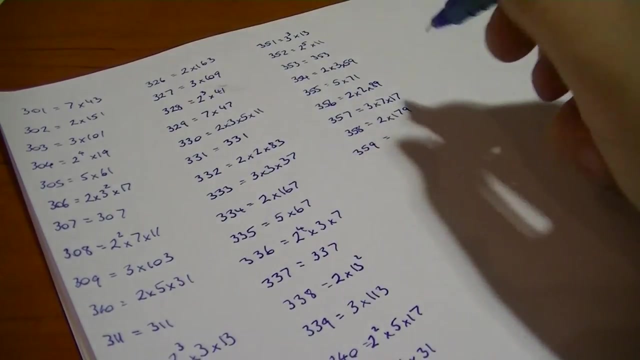 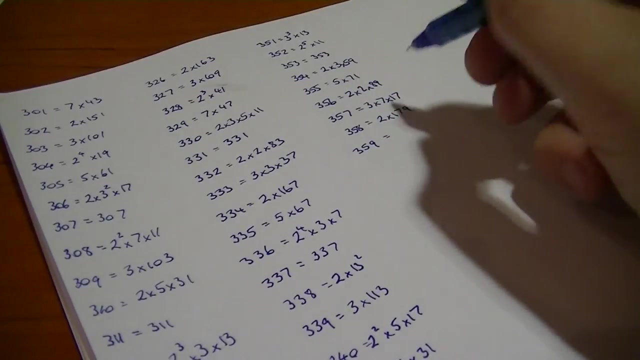 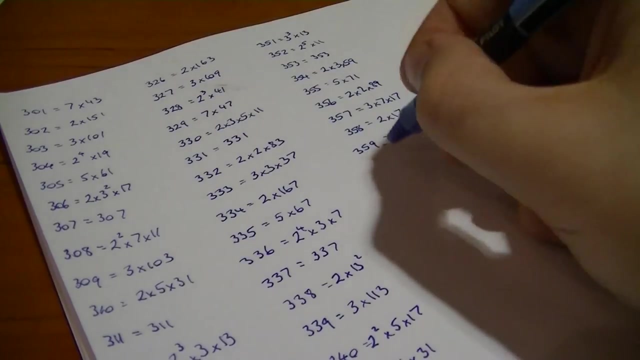 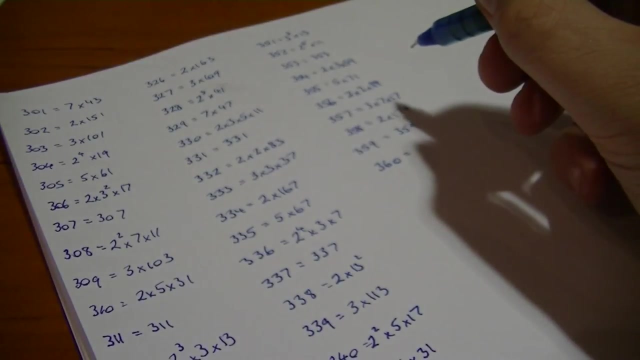 358, 179, that's a prime 359, that depends by 2,, 3, or 5, or 7, or 11, or 13, or 17,. so that's a prime. sorry, that's a prime. 360, the big 360, that's 10, 36, so 36 is 2 squared by 3 squared. 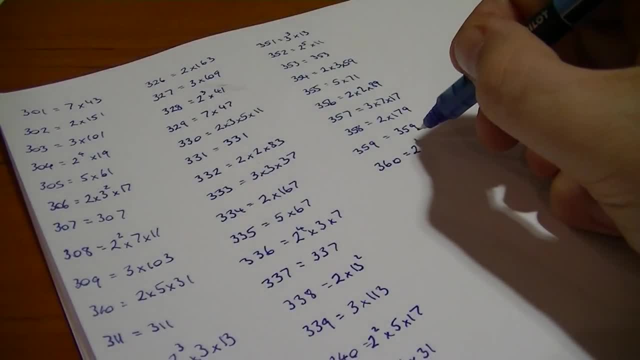 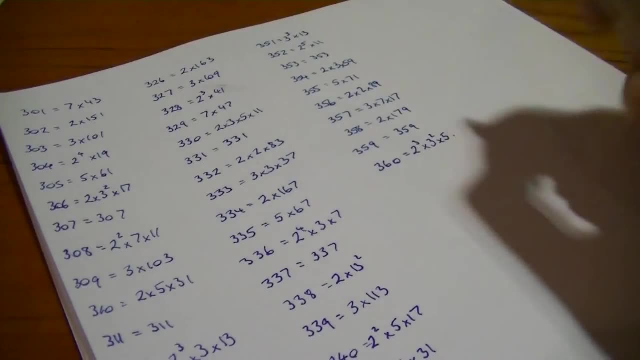 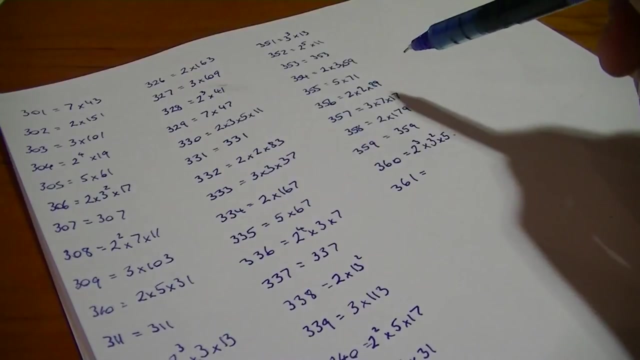 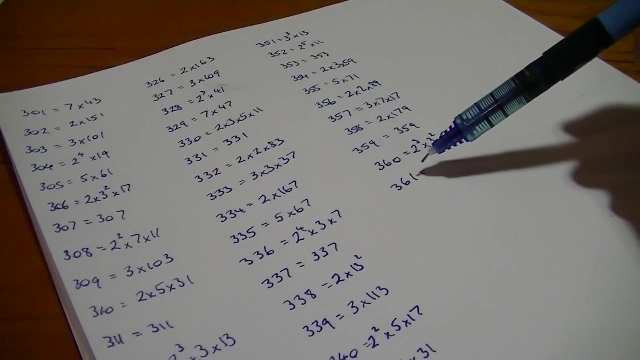 so that's gonna be 2 squared by 10, so that's 2 to the power of 3, by 3 squared by 5, 361, that depends by 2, or 3, or 5, or 7, or 11, or 13, or 17,. 3,, 3,, 4, 2, but it's supposed. 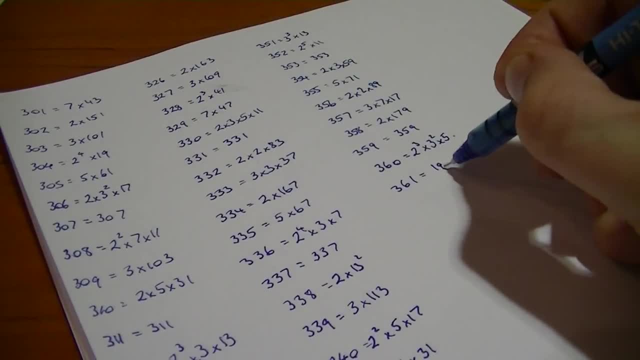 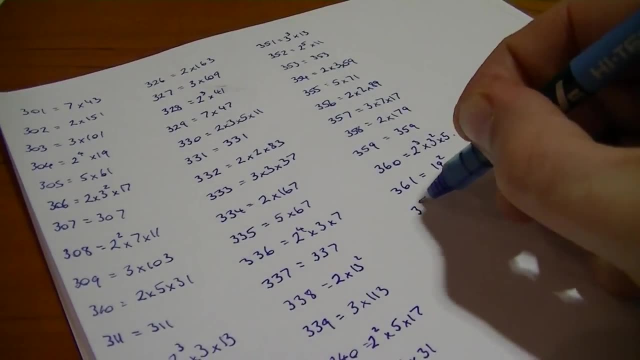 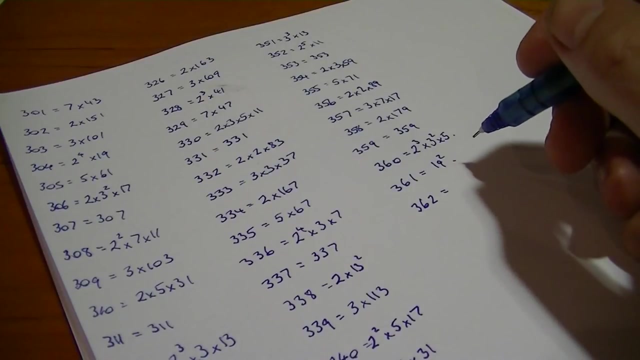 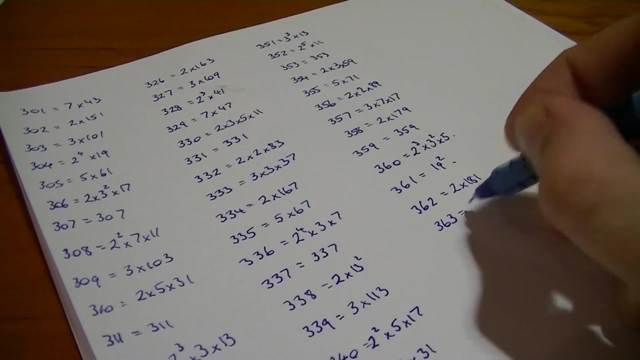 to be 19,. that's 19 squared 362, divided by 2, is 2, 181, that's a prime 3 by 1, 8, 1, 363, well, that's 3 by 121,, that's. 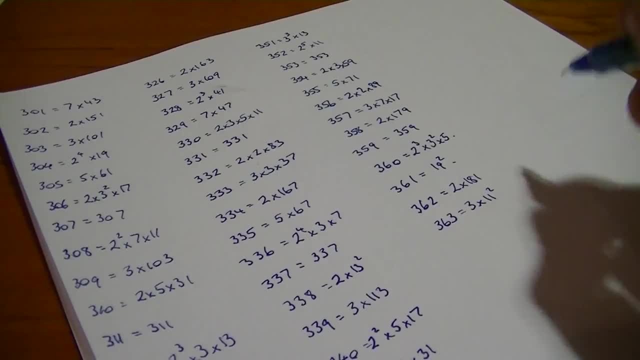 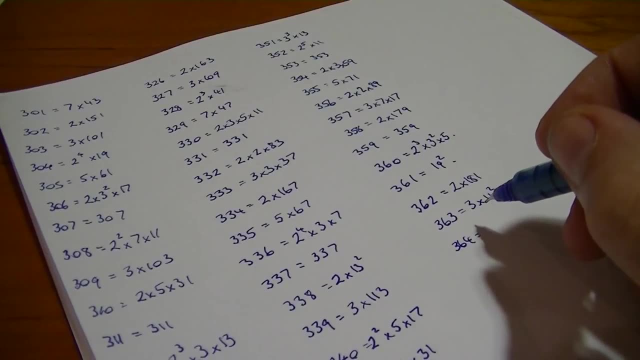 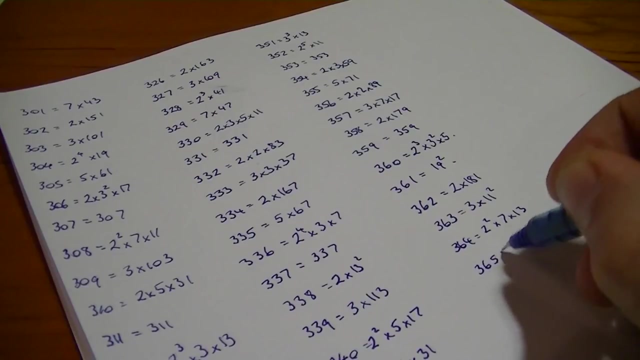 3 by 11 squared 364.. That's 4, 91s. 91 is 7, 13s. so that's 2 squared by 7, 1 by 13,, 365, that's 5,, 15,, 5, 70,, 3s. 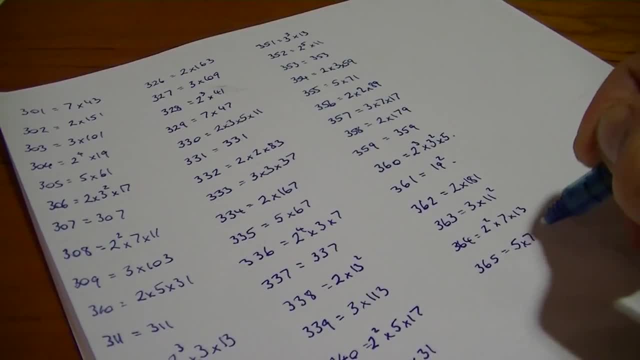 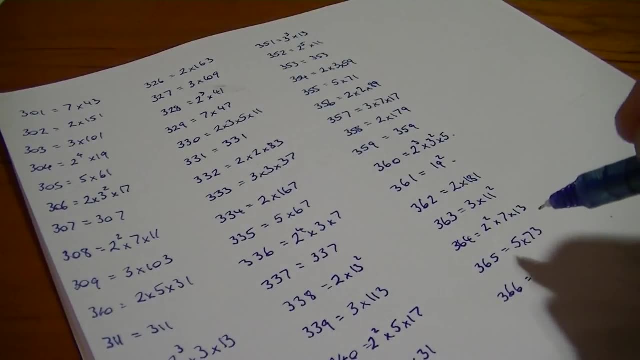 that's 2, 183s, that's 2 by 3, by 61, 367, that's not divisible by 2, or 3, or 5, or 7, or 11, or 13.. 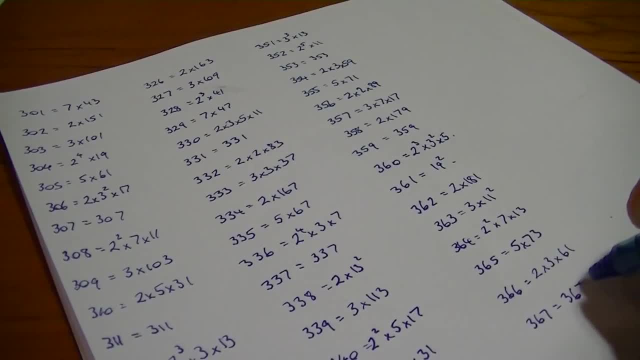 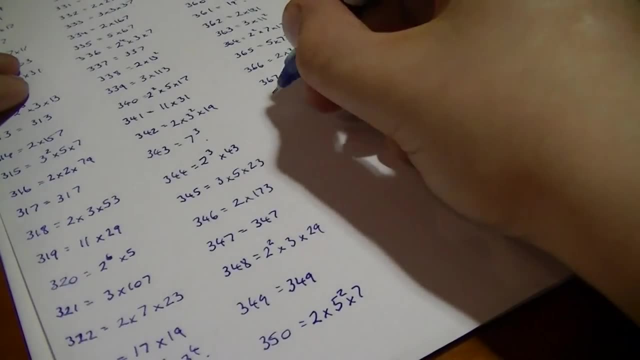 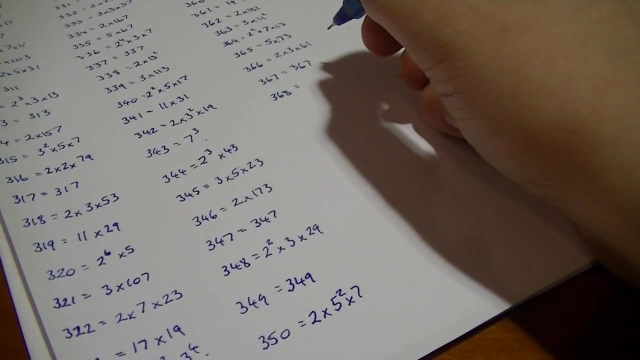 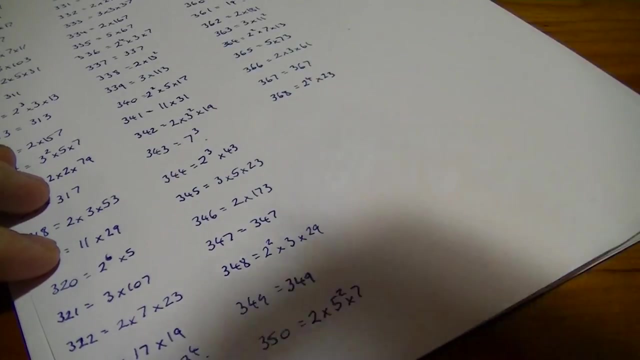 There's 17 and 18,, so that's a prime 368, and that is 2, 184s, so that's 2 to the power of 4, times 23,, 16,, 23s, 320,, 48, yeah. 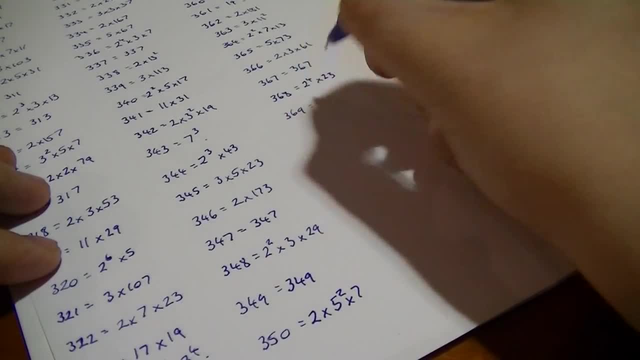 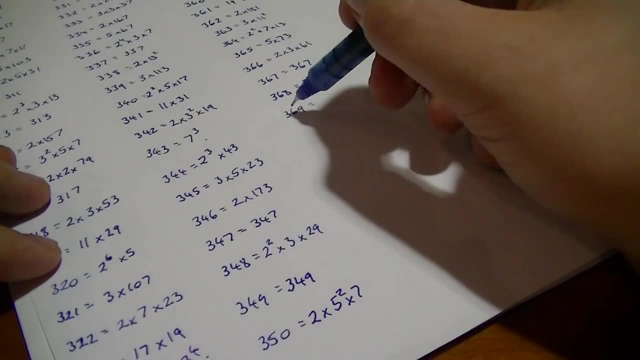 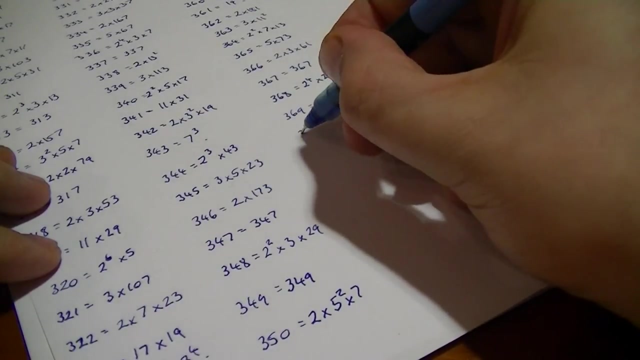 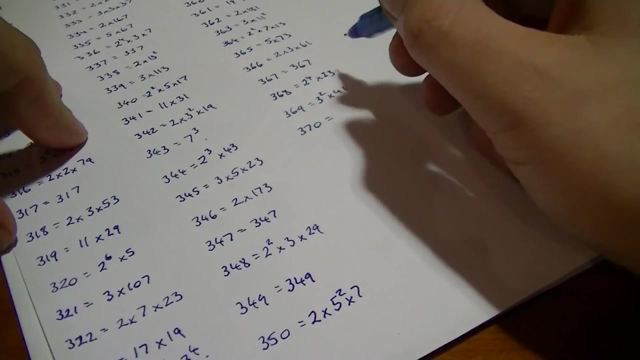 Okay: 369,, that's 3, 123s, it's 9, 41s. 41s are primes, so that's 3 squared by 41, and 370,, that's 5, 74s, and 74 is 2, 37s, so that's 2 by 5, 5, 5, 6, 7, 6, 7,, 8, 9,. 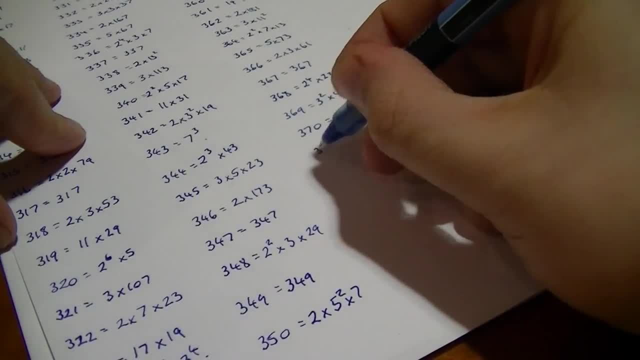 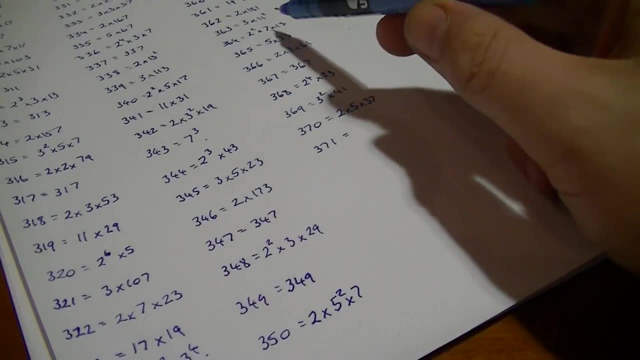 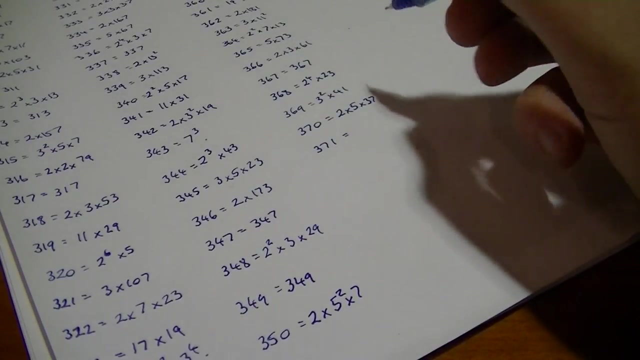 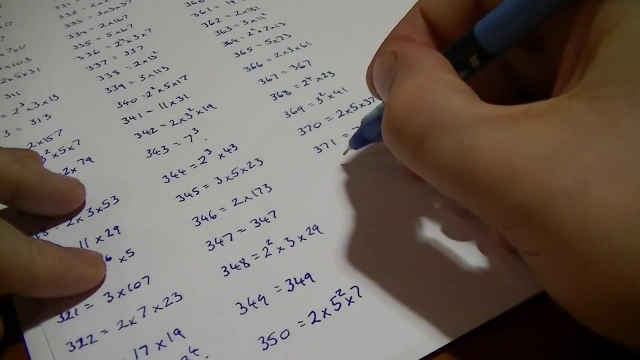 30,, 37,, 371,, that's not divisible by 2, or 3, or 5,, it's divisible by 7,, so that's 4,. 4, 13s or 52s, that's 7, 53s, 53s are primes- 7 by 53,, 350,, nothing more. yep 372,, that's. 2, 172,, 313,, 341,, 341,, 342,, 343,, 342,, 343,, 343,, 342,, 343,, 341,, 343,, 343,, 343,, 343,, 342,, 343,, 343,, 343,. 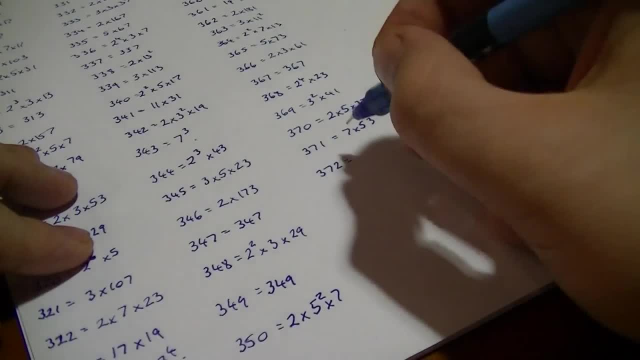 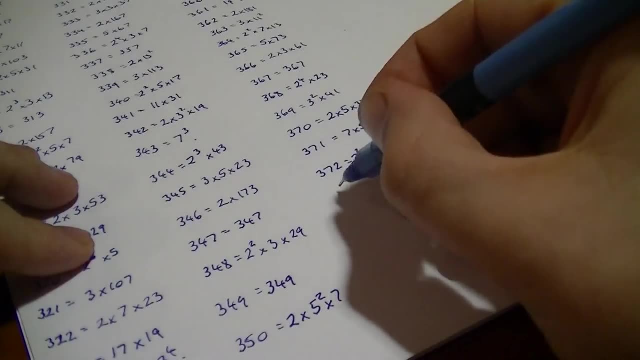 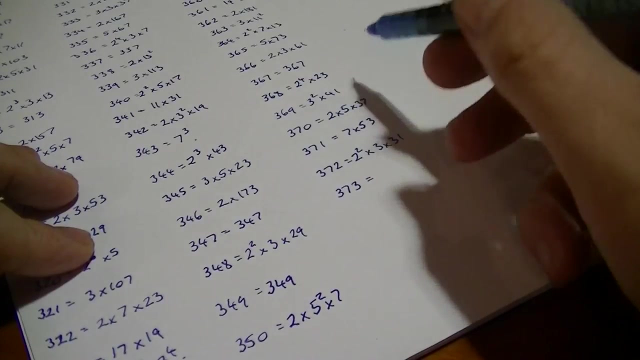 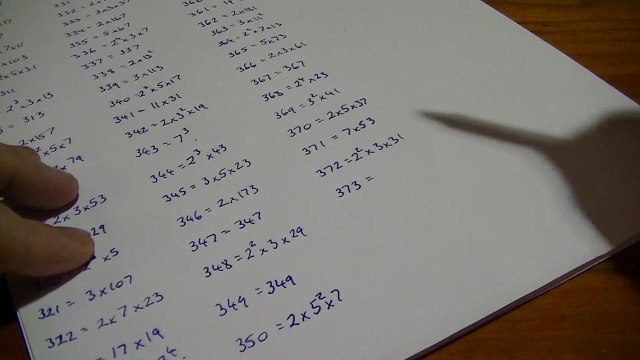 162, 186, so that's 2 squared by 3,, by 31, 373, that's not necessarily 2, or 3, or 5, or 7, or 11, or 13, or 17, or 18,. this is a prime. 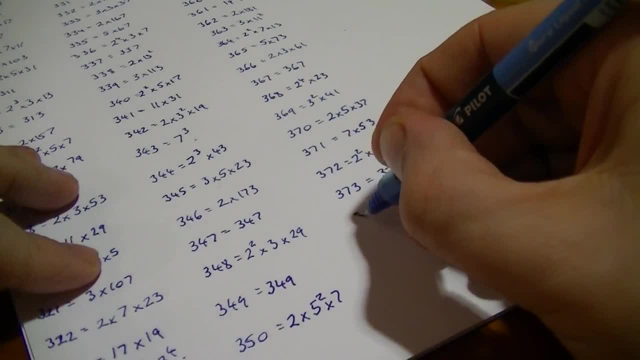 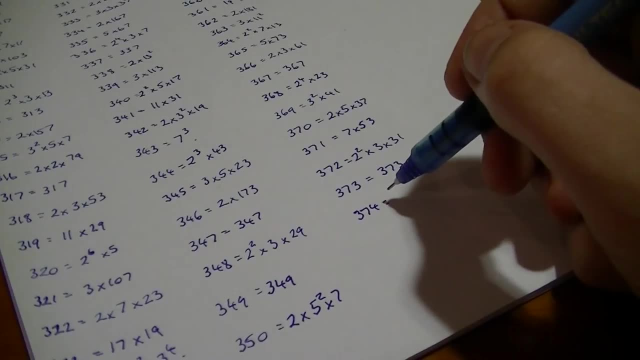 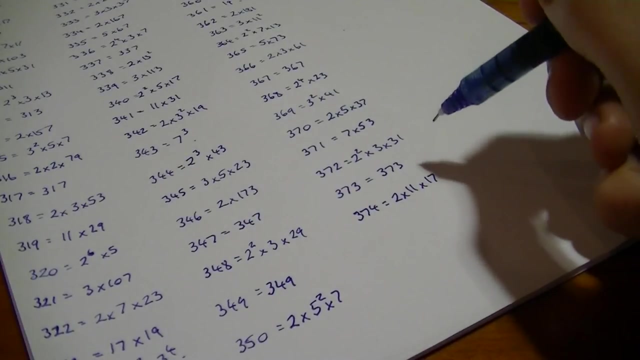 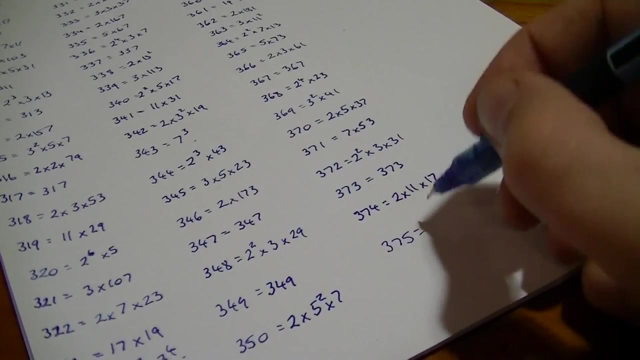 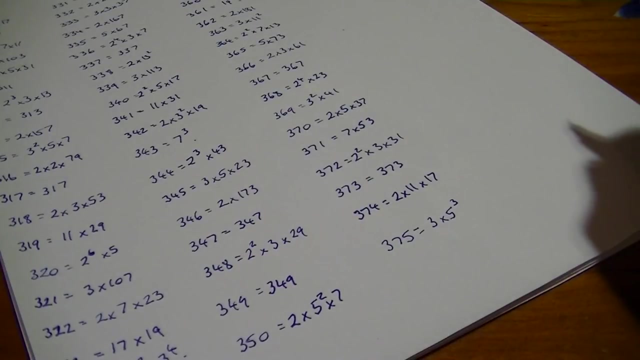 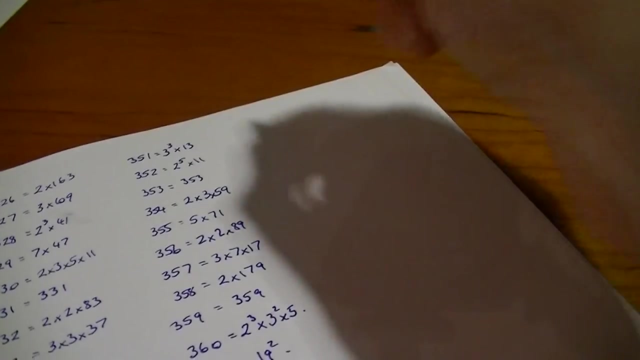 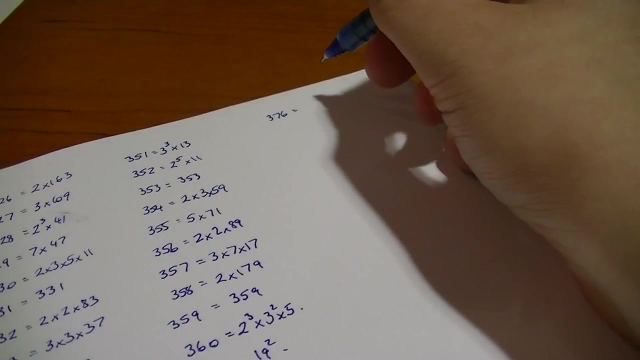 374, that's 2, 187,, that's 2 by 11, by 17,. and 375,, that's 3, 125, so that's 3 by 5 cubed. okay, just in the boundary line, let's do one more column. so 376, that's 2, 188, 288,. 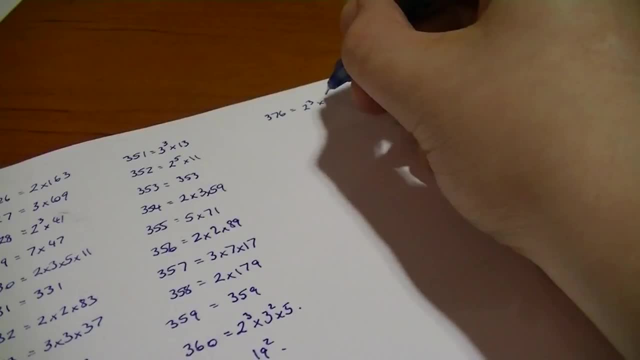 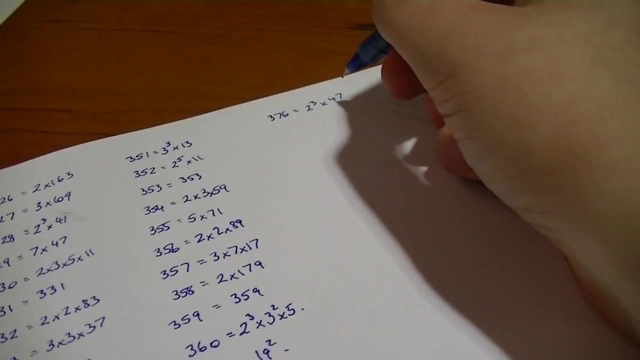 so that's 2 cubed by 47, 847, that's 328,, 356,. yep, that's 377,. that was by 2, or 3, or 5,, 7,, oh 11,. 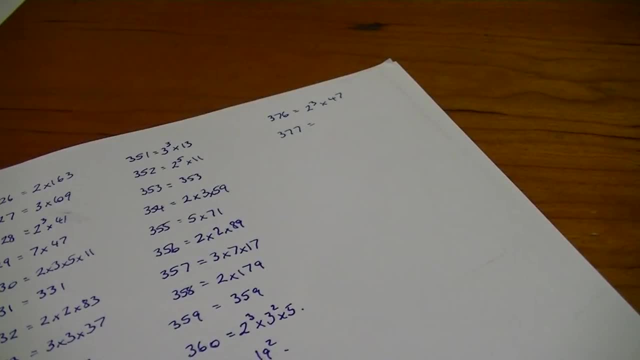 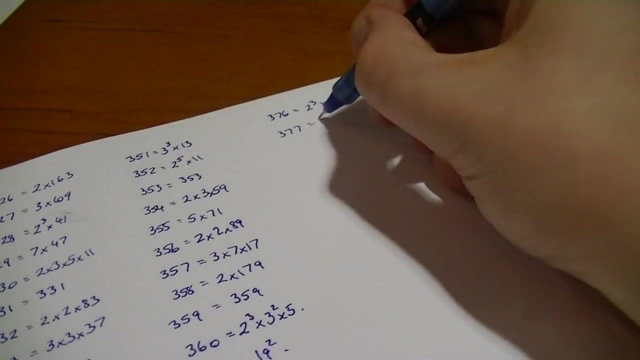 no 13,. yeah, it would be 13, it's, it's 13, 4,, 28,, 13, 29,. that's all 2 primes, so 370,, that's 2, 180,. 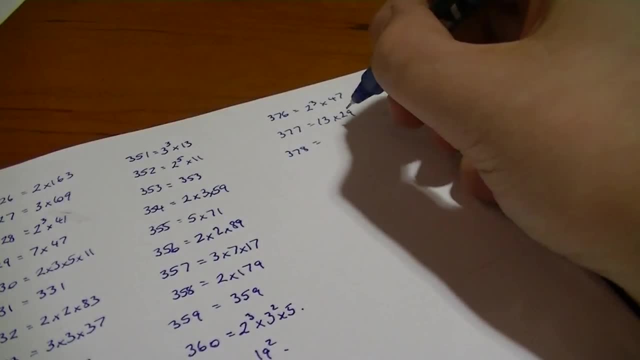 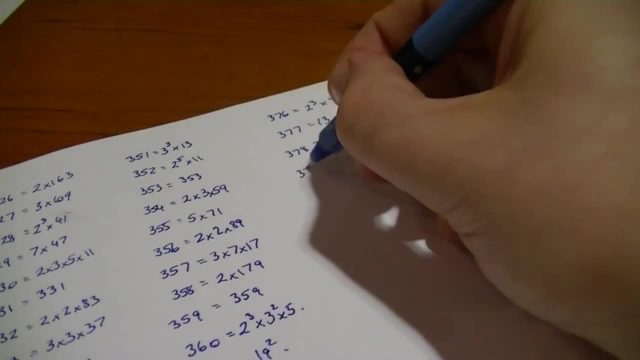 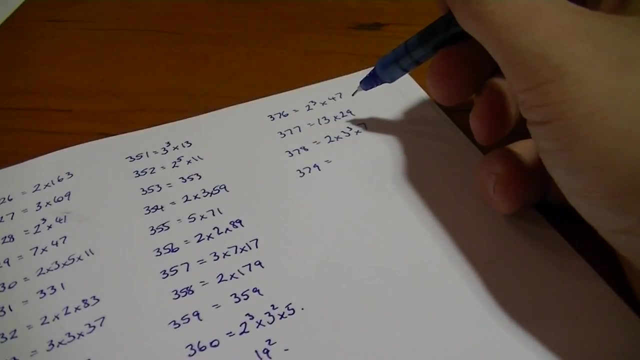 so that's 280, that's 2 by 3 cubed by 7, 379, just a little close: 2, or 3, or 5, or 7,, or 11,, or 13, or 17, or 19,. 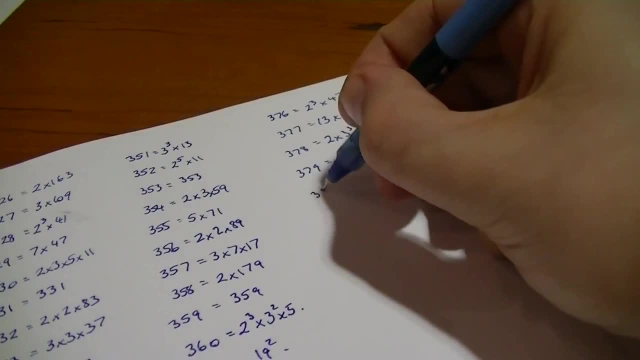 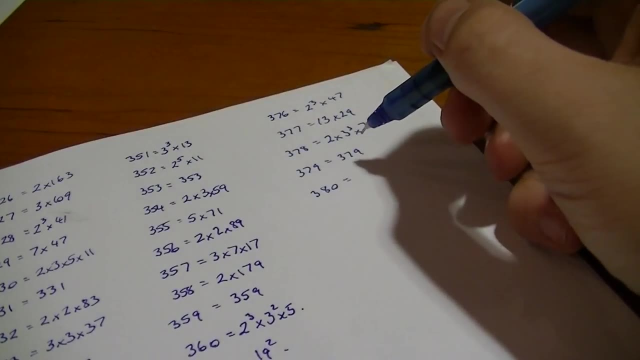 so that's a prime 380, that's 10, 39s, 30, right 10, 38s, 38 is 2, 19s, 2 primes. so that's going to be 2, 19s. 3 primes, so that's going to be 2 19s. 2 primes, so that's going to be 2 19s. 2 primes, so that's going to be 2: 9s, 2 9s. 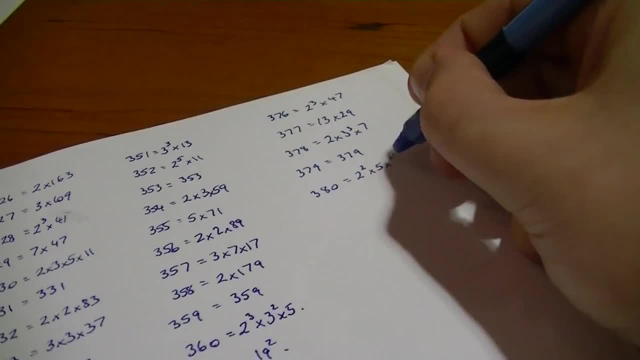 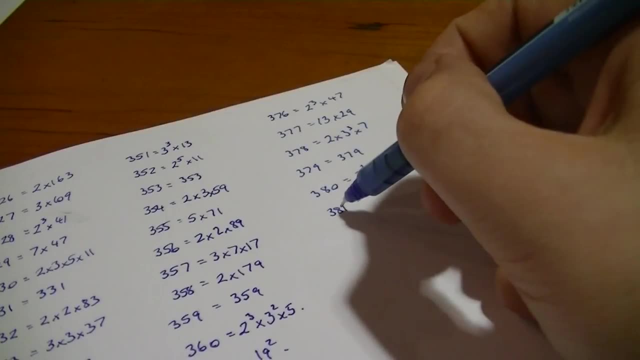 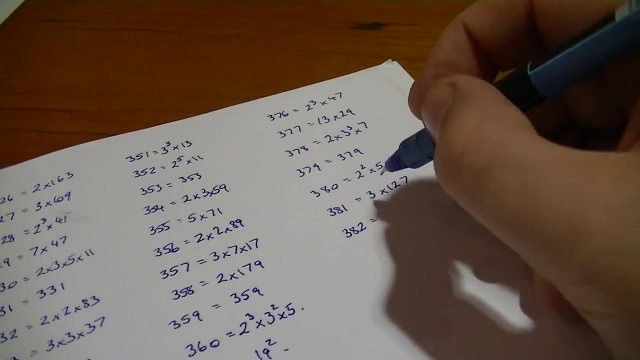 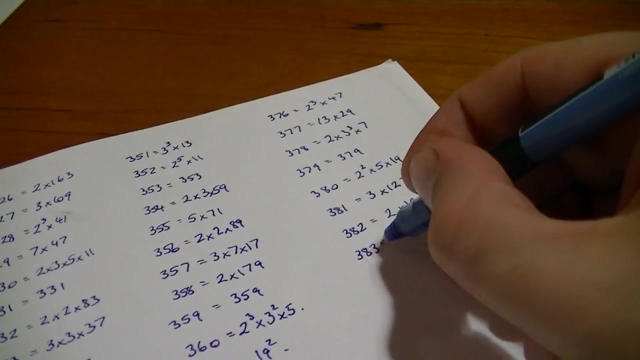 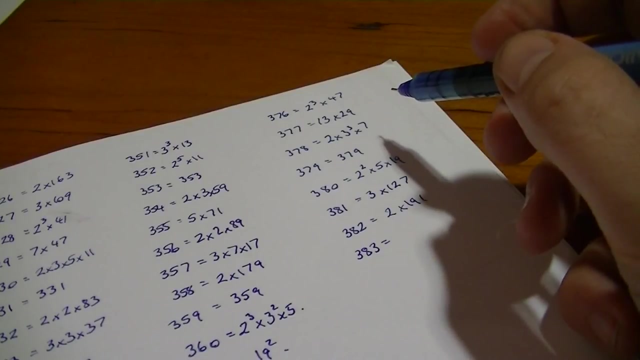 2 squared by 5 by 19.. 381.. That's three, one hundred and twenty-sevenths. One hundred and twenty-seven is a prime. Three hundred and eighty-two is two hundred and eighty-one. That's a prime. Three hundred and eighty-three, That depends on whether you're two or three or five or seven or eleven or thirteen. 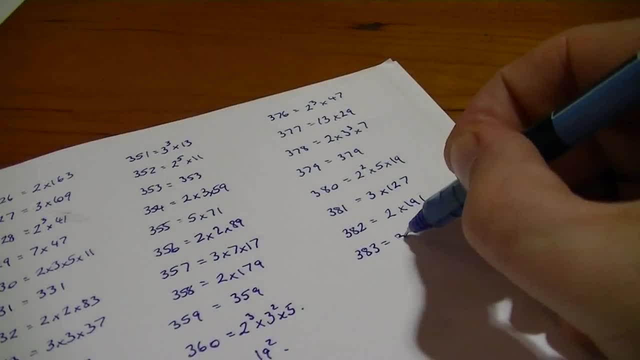 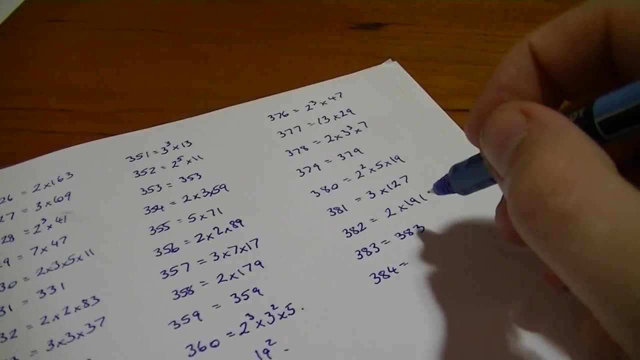 Thirteen or seventeen or nineteen. That's just a prime. I just want to write prime there. My mind's away with it. This is quite mentally taxing Two. one hundred and ninety-twos, That's four. ninety-sixths, which is eight. 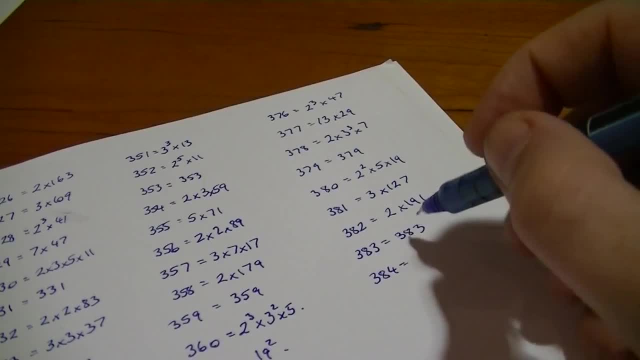 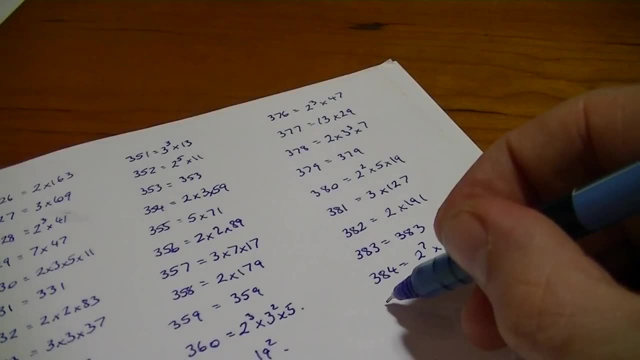 I don't care, It's two hundred and ninety-twos. Let me look at that one. So that's two or seven by three. If it wasn't for looking at the sheets that I've written out previously, then I think my mind would be mental. 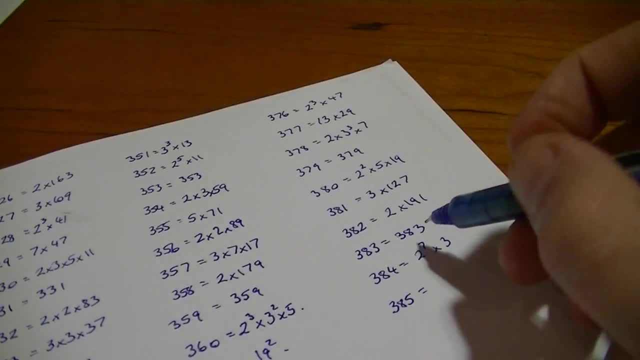 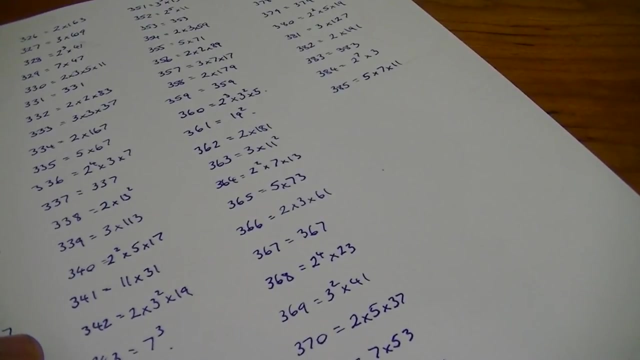 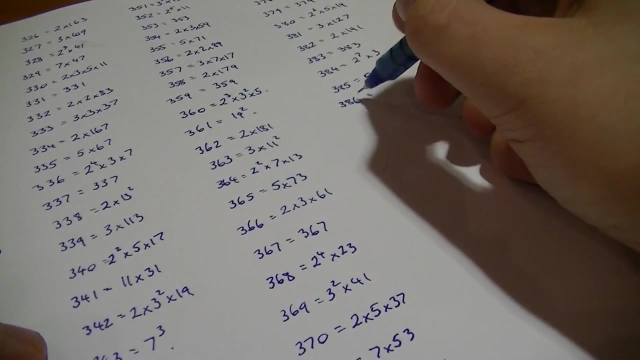 More mental than you might think. Three hundred and eighty-five, Well, that was five seventy-sixths, This is five seventy-sevenths, So it's five by seven, by eleven. Three hundred and eighty-six, That's two. one hundred and ninety-threes. 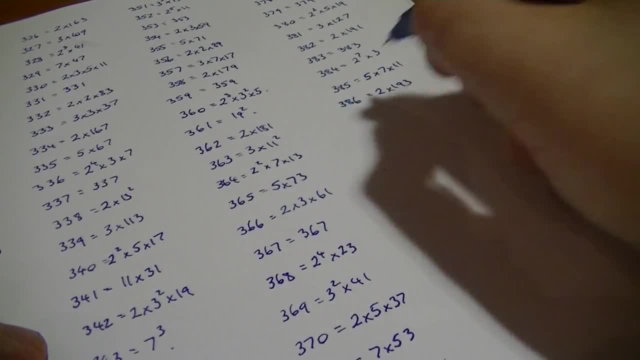 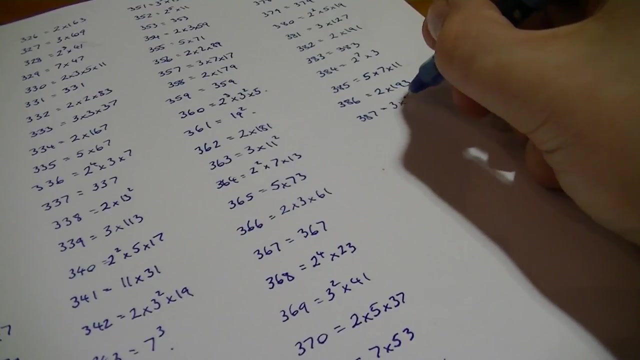 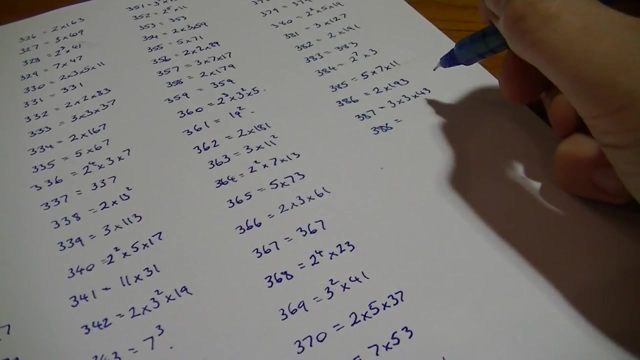 That's a prime. Three hundred and eighty-seven, That is three. one hundred, That's three. one hundred and twenty-times, That's three by three, by forty-three. Three hundred and eighty-eight, That's two, one hundred and ninety-fours. 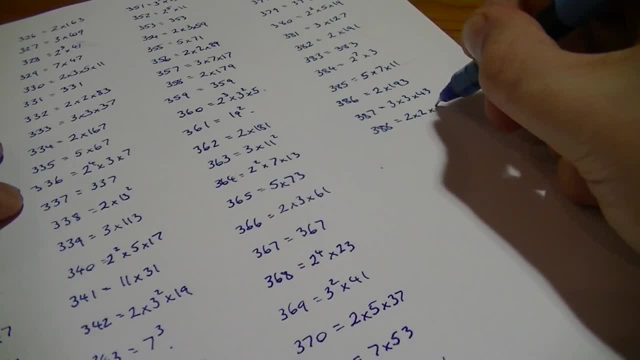 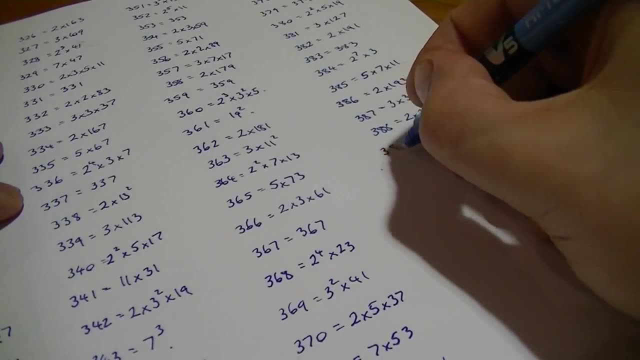 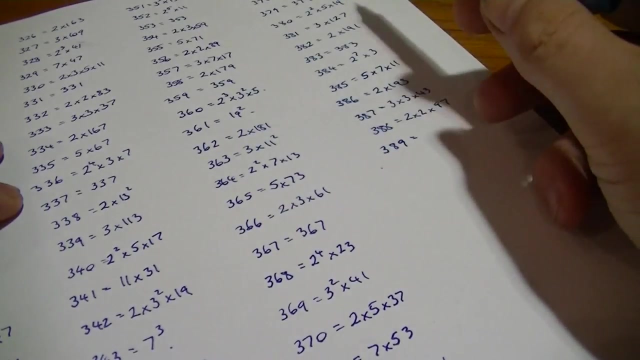 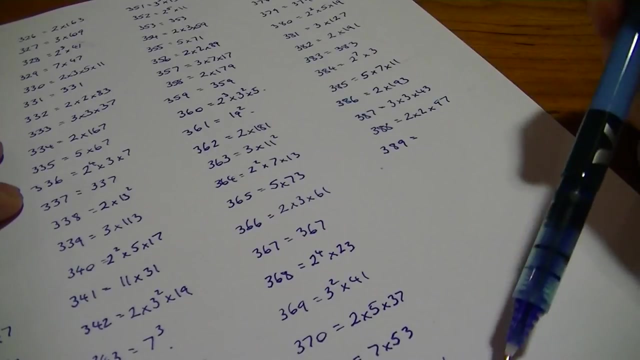 So that's two by two by ninety-seven, Three hundred and eighty-nine, Not supposed to be two or three or five or seven or eleven, Or thirteen Or seventeen Or seventeen Or nineteen Or nineteen. So that's a prime. 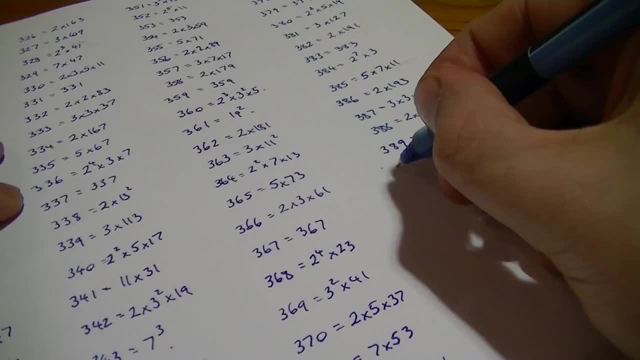 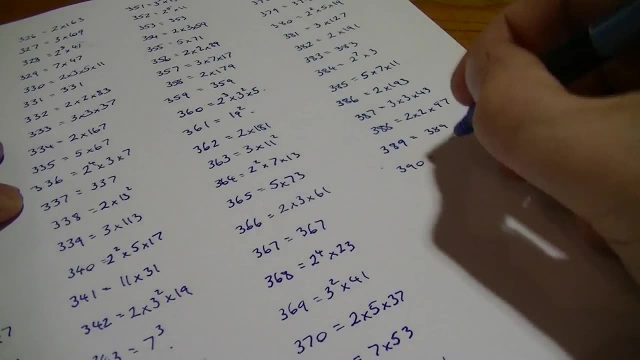 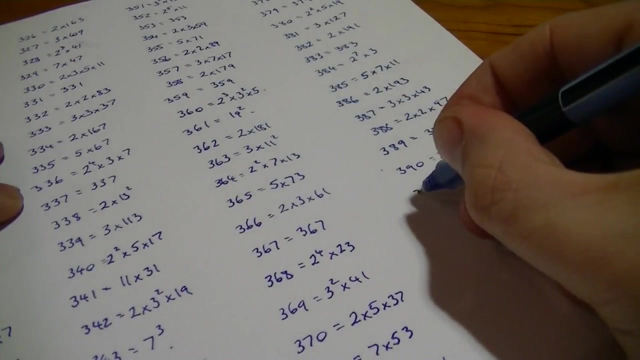 Three hundred and nineteen, That's ten thirty-nines. Thirty-nine is three, thirteenths, So that's two by three, by five, by thirteen. Three hundred and ninety-one. That's not supposed to be two or three or five. 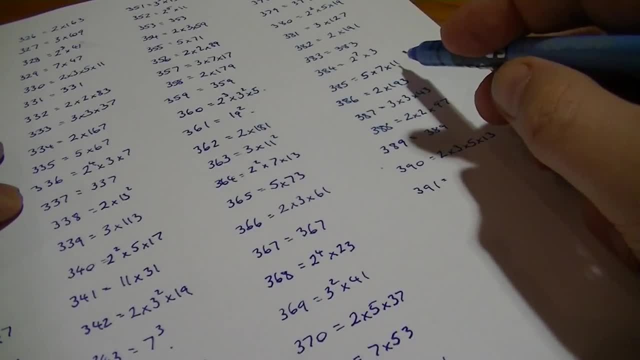 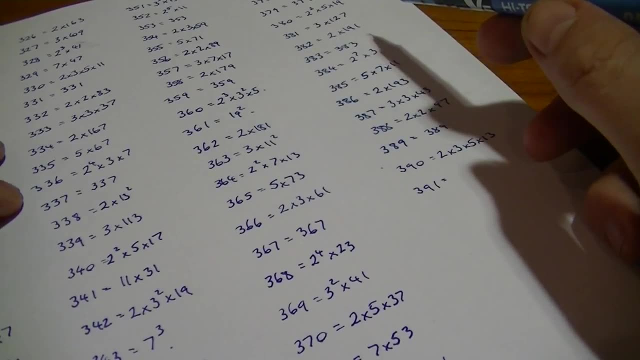 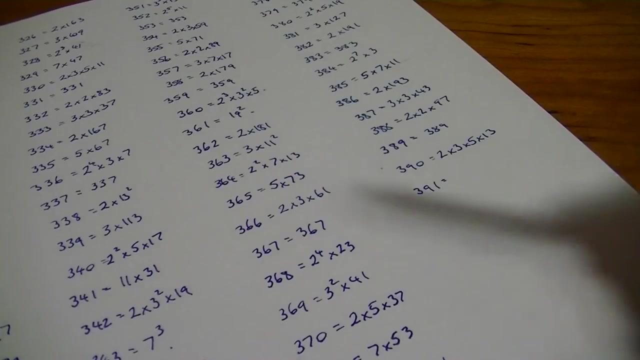 Which is ten. No, No, No. Thirteen, That'll be three-sevenths, No, Thirteen, Seventeen, Yep Seventeen, It's twenty-two, twenty-three-sevenths, So that's seventeen by twenty-three. 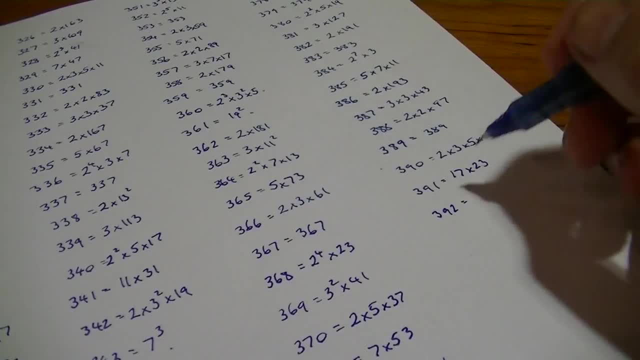 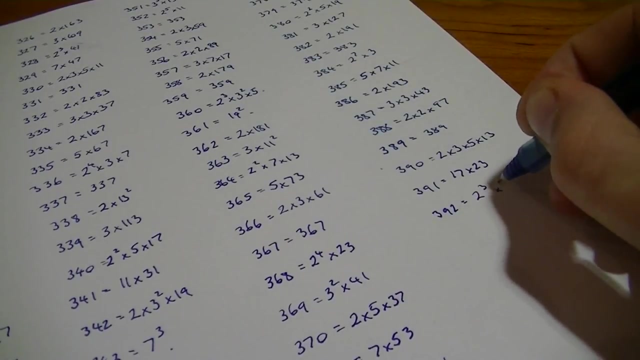 Three hundred and ninety-two, That's two times Yeah, That's almost a guess of who knows Alright Two Once you move to one hundred and ninety-six. Two times one hundred and ninety-six, So that's two cubed by seven squared. 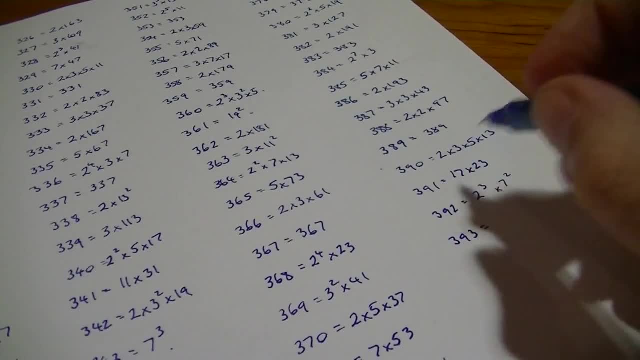 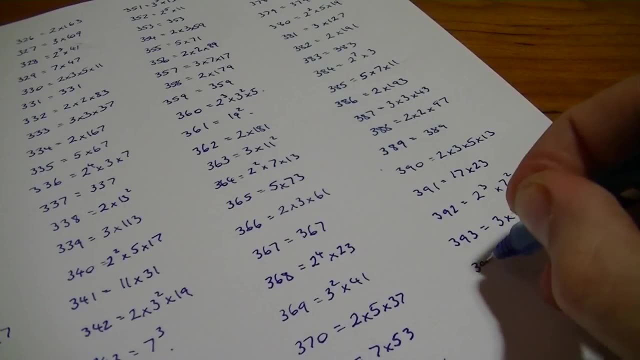 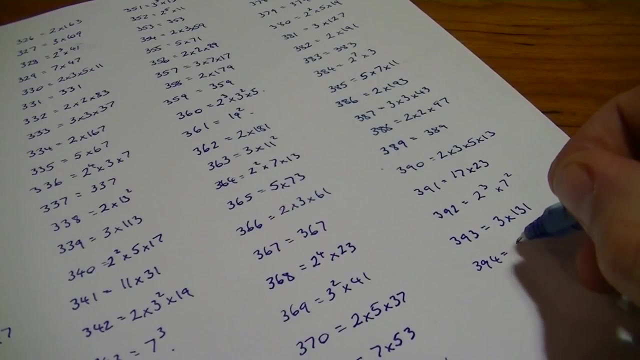 Three hundred and ninety-three, That's three times one hundred and thirty-one. Thirty-one's a prime. Three hundred and ninety-four, So that's two times one hundred and ninety-seven. One hundred and ninety-seven's a prime, Good job. 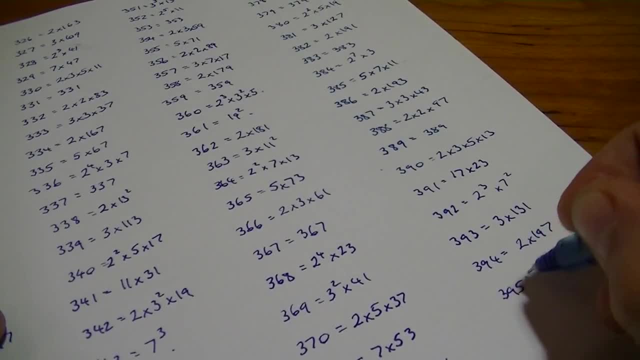 Three hundred and ninety-five, Four hundred's five-eighty, So that's five-seventy-nine. Seventy-nine is a prime Five by seventy-nine. Three hundred and fifty, Forty-five. Three hundred and ninety-six Is two times one hundred and ninety. 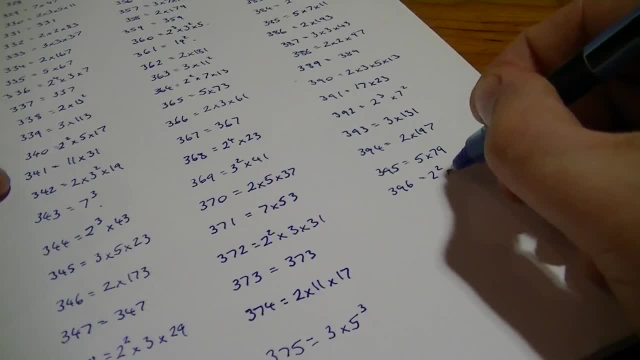 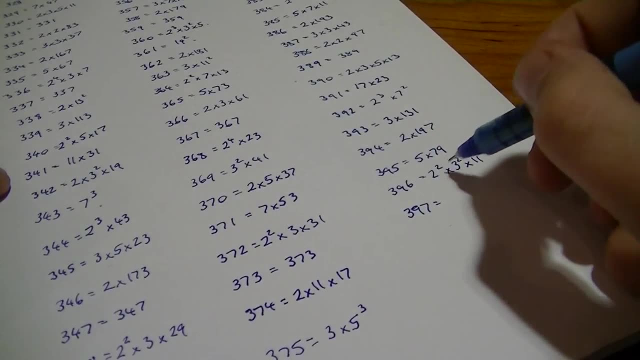 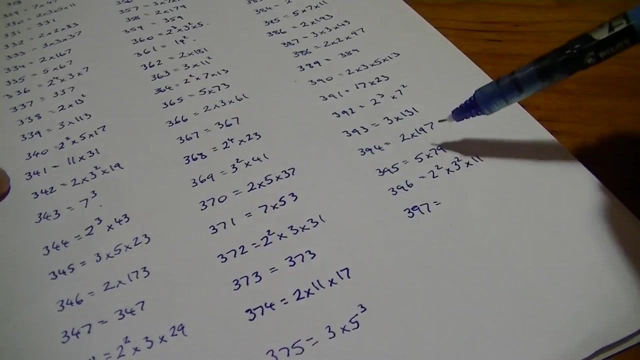 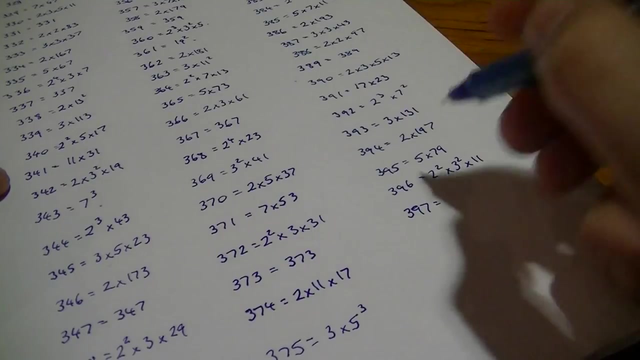 Yep, So that's two squared by three, squared by eleven. Three hundred and ninety-seven, Not if it's by two or three, or five or seven or eleven or thirteen or seventeen Or seventeen or nineteen. No, That's a prime. Three hundred and ninety-eight. 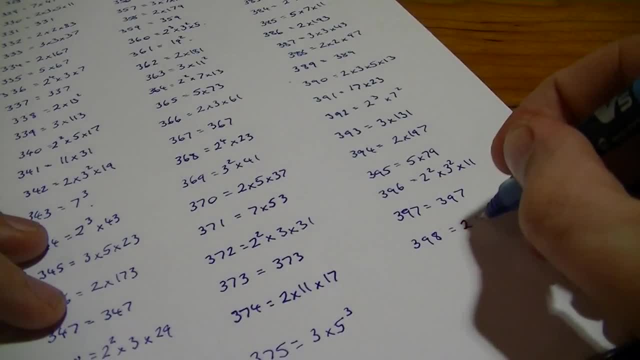 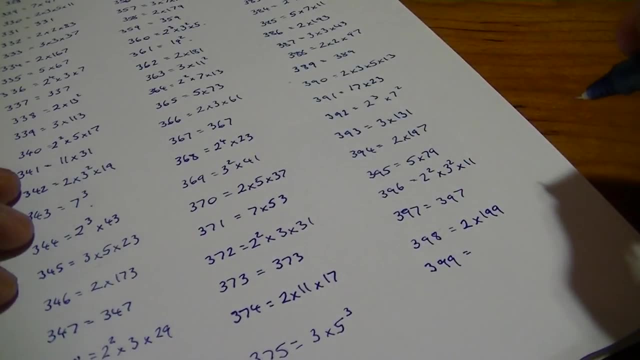 That's two times one hundred and eighty-nine. That's a prime Three, Two by one. Nine, Nine, Three hundred and ninety-nine, That's three times one hundred and thirty-three. That's three by seven, by nineteen And four hundred.